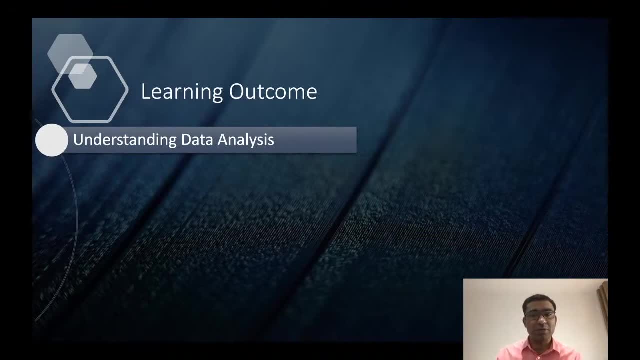 interpret and how to get your result quickly So you can use that tip anywhere, or all type of tests or all type of data analysis that will be better for you in order to understand what is happening there. Okay, First thing, we need to understand the data. The second one would be introduction to this. 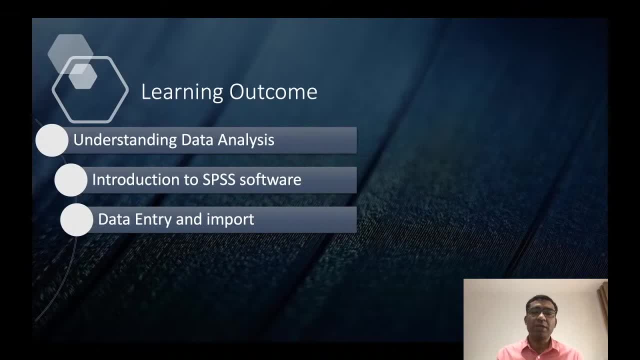 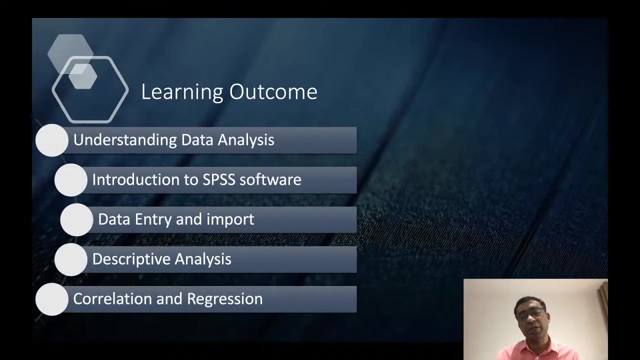 SPSS software. The next step would be: we need to understand the SPSS environment: how we can do the data entry, how we can import our excel sheets, how we can work with the SPSS software. That would be next point. And finally, we will do some descriptive analysis and correlation. 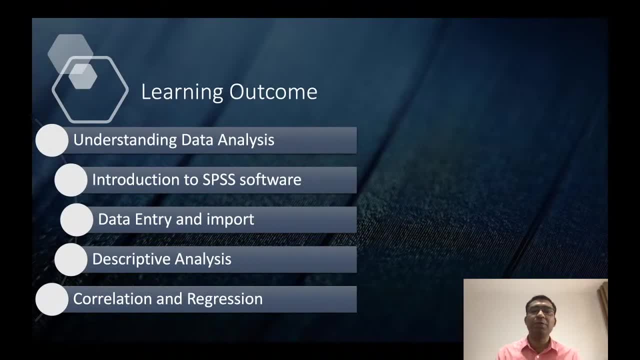 and regression. that is part of your CELIPA. So this would be the learning outcome for today's lecture. But let's start and let's try to learn step-by-step, So in that case you can be in a condition to understand the concept very clearly. Okay, now let's move on. So first thing we need: 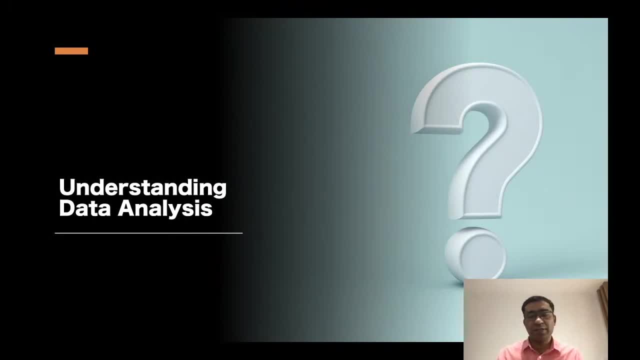 to understand is basically what is your data analysis? and, if you remember, in the last class I already explained about the different forms of the scale and at that time I was talking about we have to learn which scale and what type of data would be available and what type of analysis we can do on each type of 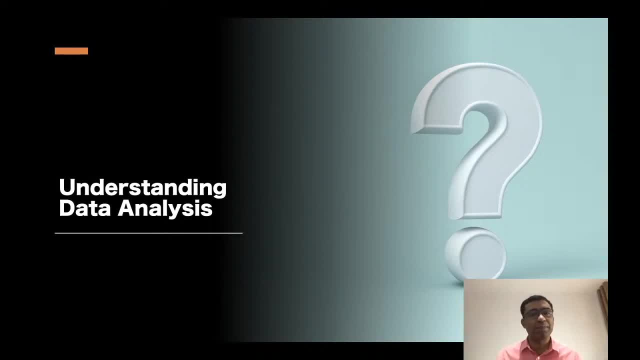 the data or each type of the scale. okay, so scales are very important in this regard and also we need to understand that the scales can be used to collect data. but also we have to understand each scale have some limitation in the data analysis. we cannot deal every scale like. 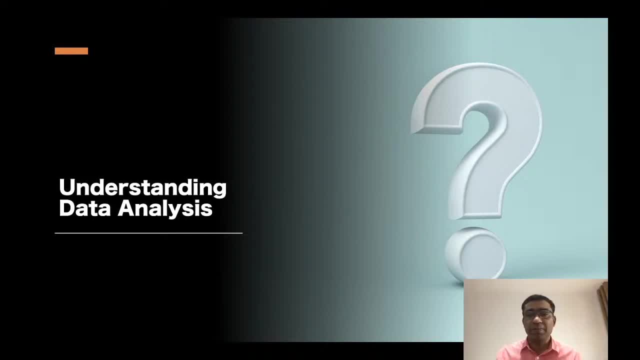 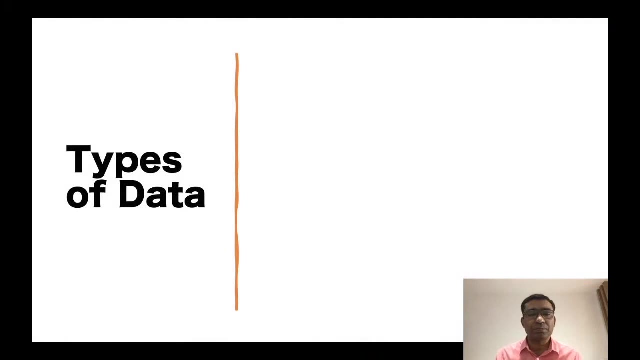 similar. so we have to do some pre-work and we have to understand what are the limitations on each scale and how we can improve or how we can use these scales in our research. okay, so this is the basic concept. now let's let's start with the previous class. 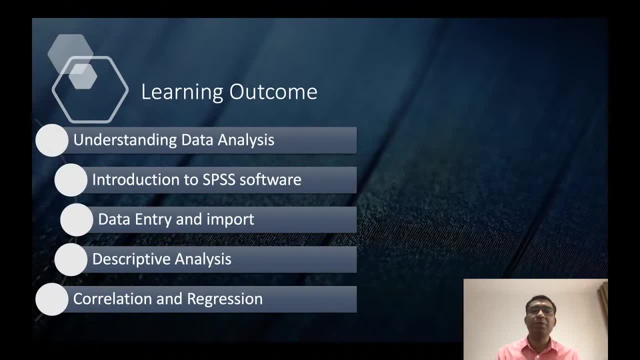 and regression. that is part of your CELIPA. So this would be the learning outcome for today's lecture. So let us start and let us try to learn step by step, So in that case, you can be in a condition to understand the concept very clearly. Okay, Now let us move on. So, first, 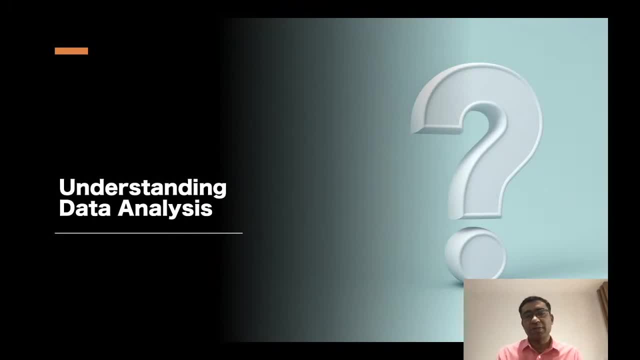 thing we need to understand is basically what is your data analysis and, if you remember, in the last class I already explained about the different forms of the scale and at that time I was talking about learn which scale and what type of data would be available and what type of analysis we can do on. 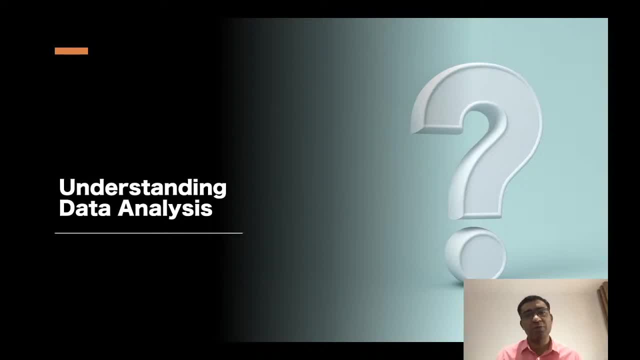 each type of the data or each type of the scale. okay, so scales are very important in this regard and also we need to understand that the scale can be used to collect data. but also we have to understand each scale have some limitation in the data analysis. we cannot deal every scale like. 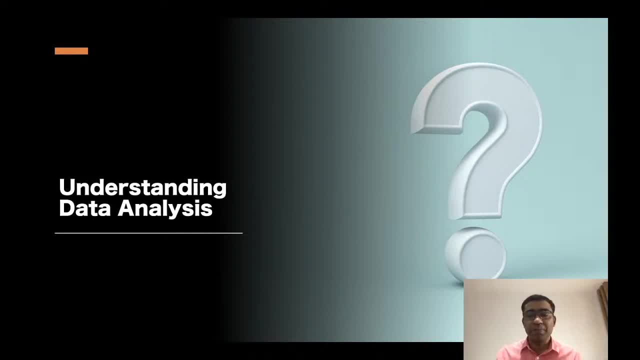 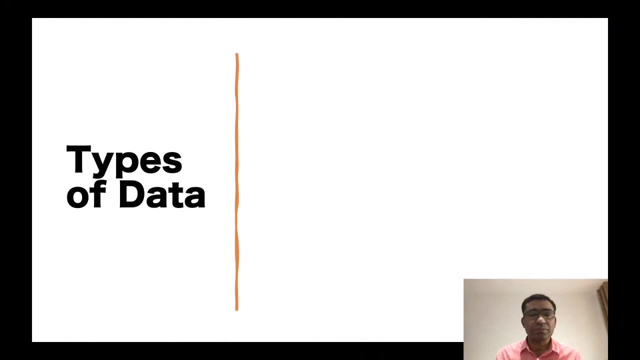 similar. so we have to do some pre-work and we have to understand what are the limitations on each scale and how we can improve or how we can use these scales in our research. okay, so this is the basic concept. now let's let's start with the previous class. 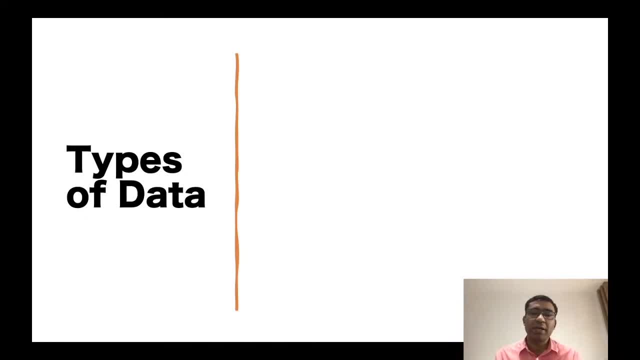 a class before the last class. if you remember, i told you about the four different types of the data. now these are the types of the scales also. so we understand that the first scale is nominal. do you remember what is nominal scale? any confusion on this? everybody is clear on the. 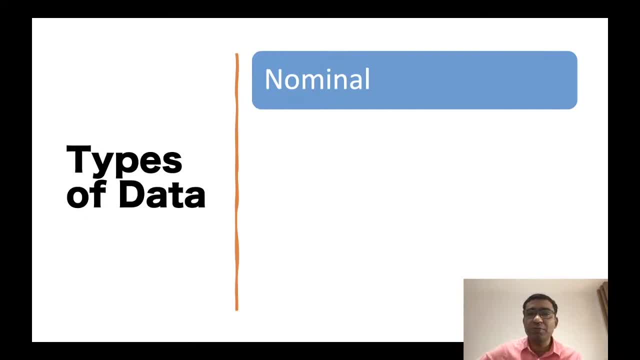 nominal scale. nominal scales are those scale where we use different types of the categorization labels to identify the different groups of your sample or your population. okay, so this is called nominal scale. for example, color, for example, different age groups. so all these different types of the scales are different. 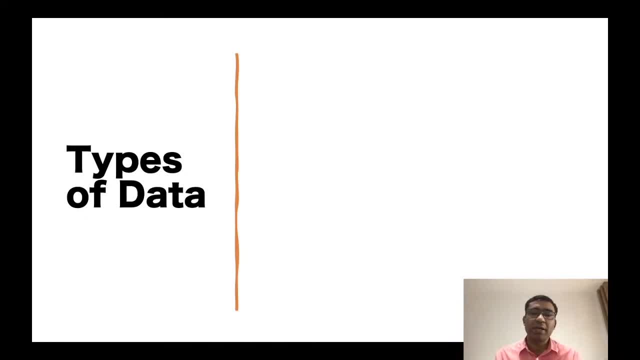 a class before the last class. if you remember, i told you about the four different types of the data. now these are the types of the scales also. so we understand that the first scale is nominal. uh, do you remember what is nominal scale? any confusion on this? everybody is clear on the. 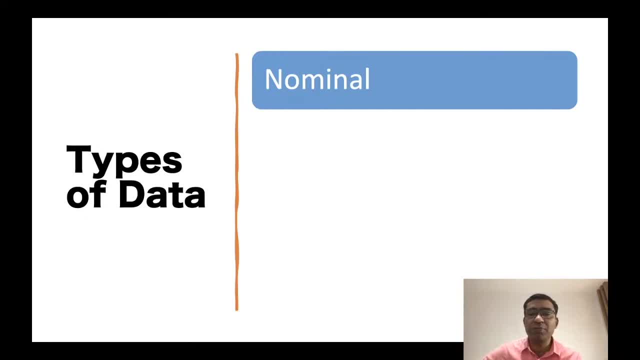 nominal scale. nominal scales are those scale where we use different types of the categorization labels to identify the different groups of your sample or your population. okay, so this is called nominal scale. for example, color, for example, different, uh, age group. so all these different types of the scales are. 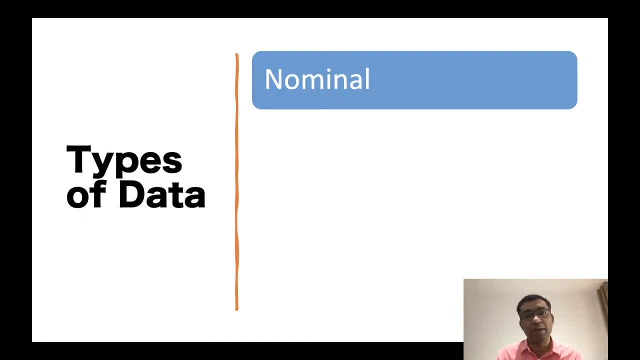 uh, different types of the groups are basically nominal: male, female. okay, classes, semesters, all these are basically nominal scales. okay, now in the nominal scale, because it is just simple categorization of group. so we have very limited options in terms of doing statistical analysis, if you remember. 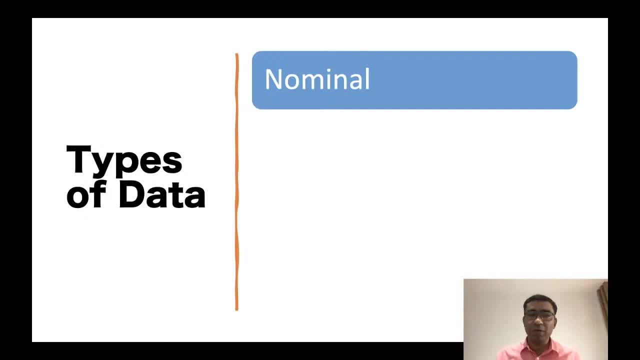 i mentioned that on the nominal scale we can only do frequency distribution. you remember we can only do frequency distribution. remember this nominal scale you cannot take mean you cannot run all the descriptive statistics, because it is the nominal scale and it is categorized with respect to the different groups. 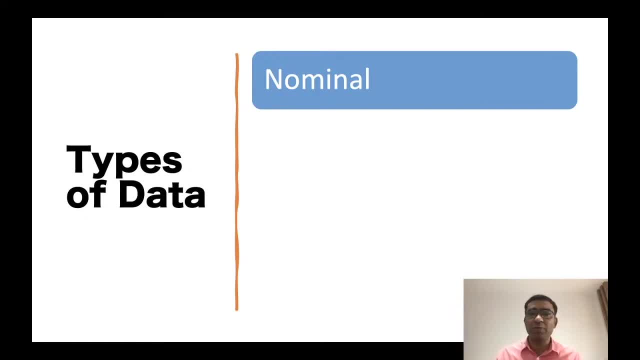 labels or tags. so that is why we cannot do means or medians or more, we just do simple frequency distribution. okay, then i mentioned the ordinal scale. if you remember, the ordinal scale is the scale where i mentioned that the- the data is followed by an order- mean that there is a rank. 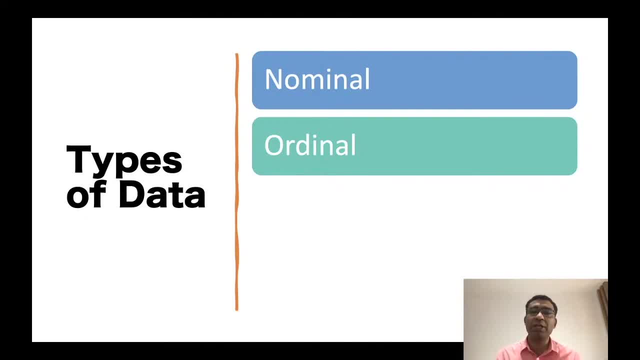 between the options available for the user. so the data we receive from the ordinal scale is will be in the ranking. okay, so this rank scale or this ordinal scale. we have some limitations. we can use descriptive or we can use some statistics, but very limited inferential statistics are possible. I am using these two words: descriptive statistics and 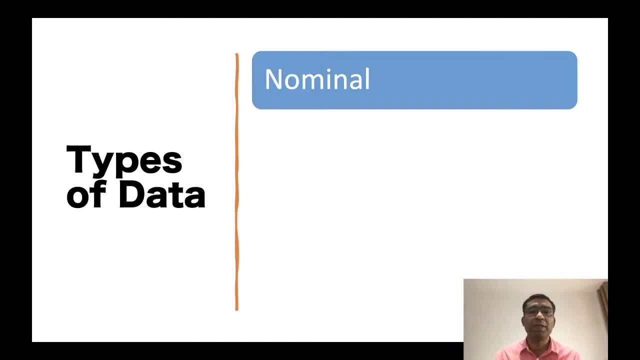 types of the groups are basically nominal: male, female, okay, classes, semesters, all these are basically nominal scales. okay now in the nominal scale, because it is just simple categorization of group. so we have very limited options in terms of doing statistical analysis. if you remember, i mentioned that on the nominal scale we can only do 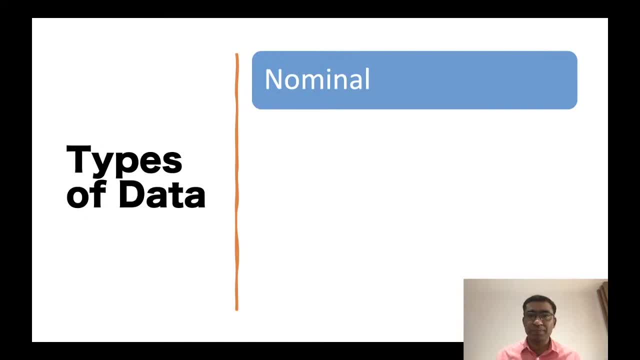 frequency distribution. you remember we can only do frequency distribution. remember this nominal scale you cannot take mean, you cannot run all the descriptive statistics, because it is the nominal scale and it is categorized with respect to the different groups, labels or tags. so that is why we cannot do means or medians or more, we just do. 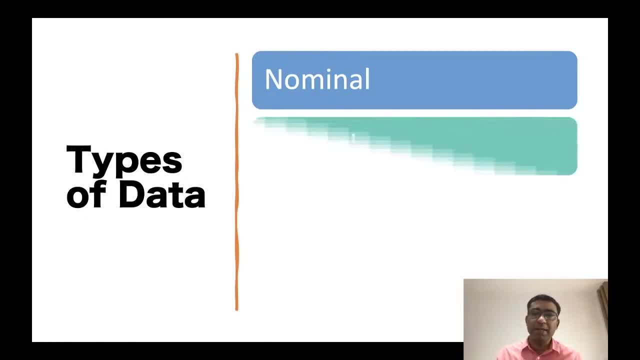 simple frequency distribution. okay, then i mentioned the ordinal scale. if you remember, the ordinal scale is the scale where i mentioned that the- the data is followed by an order- mean that there is a rank between the options available for the user. so the data we receive from the ordinal scale is will be in the ranking. okay, so this rank scale or this ordinal scale? 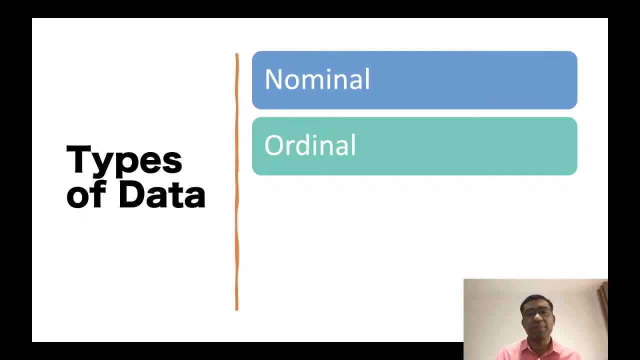 we have some limitations. we can use descriptive or we can use some statistics, but very limited inferential statistics are possible. i am using these two words: descriptive statistics and inferential statistics. i am going to explain these two terms in a while, so don't worry about that. i will explain each and every step in detail. 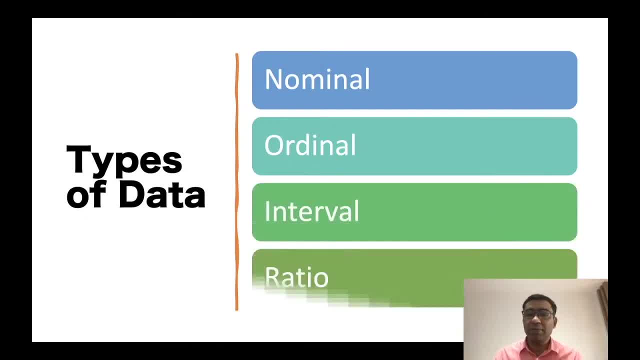 for here. so the next scale was interval. and then we have ratio scale, so we are using interval scale in terms of rating scale, and also we are using liquid scale in terms of interval scale. so you are using rating or you are using interval scale- sorry, liquid scale in the under the interval scale. so that is how we have different types. 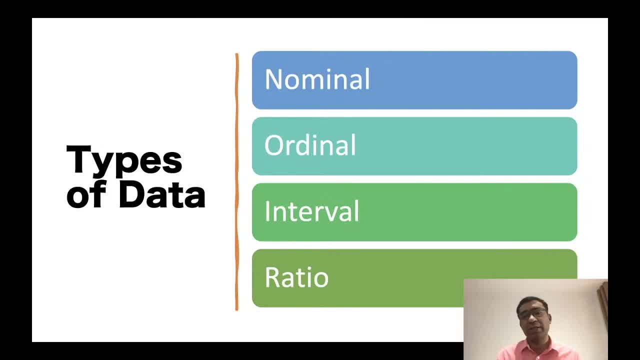 of our data and this is what i explained in detail in the previous lecture. so you can get that lecture and you can understand that this is very simple, in order to understand these different types of the data. why i'm telling you this now? because this is what we need to. 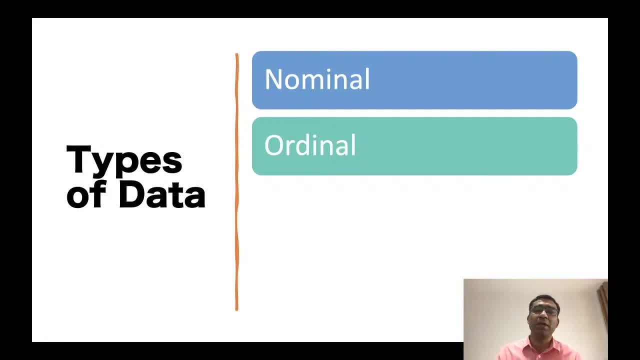 inferential statistics. I am going to explain these two term in a while, so don't worry about that. I will explain each and every step in detail for here. so the next scale was interval, and then we have ratio scale. so we are using interval scale in terms of rating scale and also we are using Likert scale in 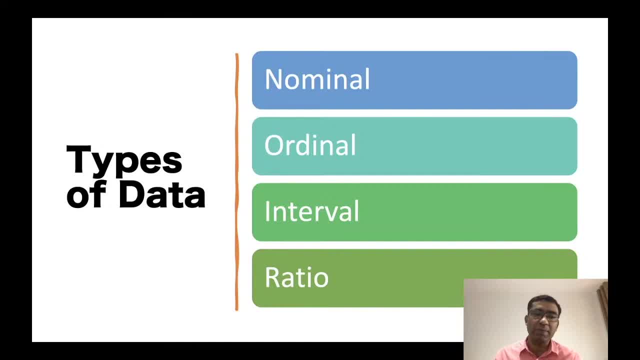 terms of interval scale. so you are using rating or you are using interval scale- sorry, Likert scale- in the under the interval scale. so that is how we have different types of our data and this is what I explained in detail in the previous lecture. so you can get that lecture and you can understand that this. 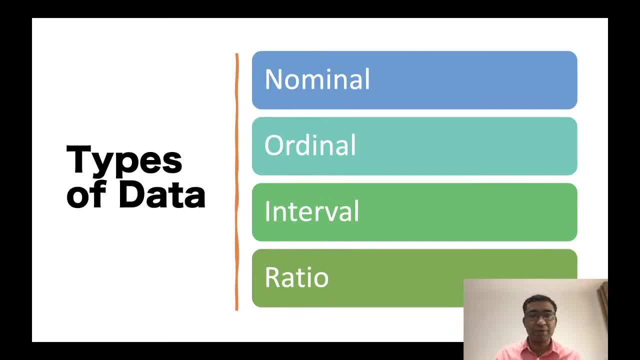 is very simple in order to understand these different types of the data. why I am telling you this now? because this is what we need to use in the SPSS. so please make sure when I explain everything it is clear to you. okay, if you have any question, you can post in the comment and I will try to. 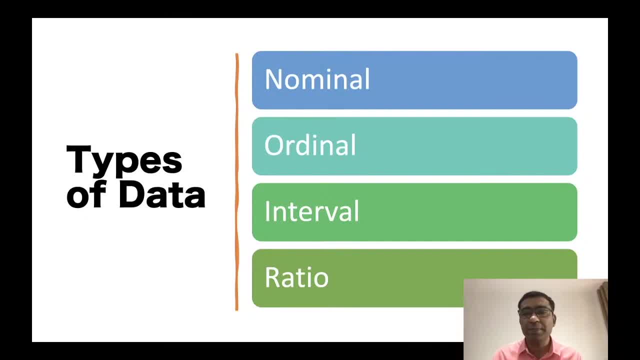 answer your question instantly, okay, so here I would take a little break and I request you to post your answer if all these scales are very clear to you and you are using it in your research, okay, so, just waiting for your reply. please mark your answers and, my dear students, one thing we should remember: today i'm not in the mood of 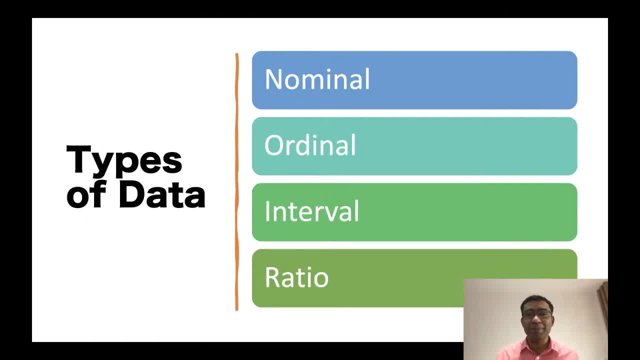 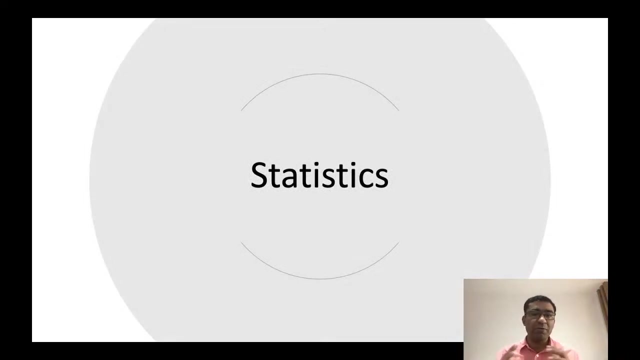 listening that particular answer you always give me me if i ask you anything, if you have any question you should ask. don't tell me everything is clear, okay. so let's move on. now we are clear about these scales. let's move to the next step. the next step is trying to understand statistics. okay, now, if you try to understand, 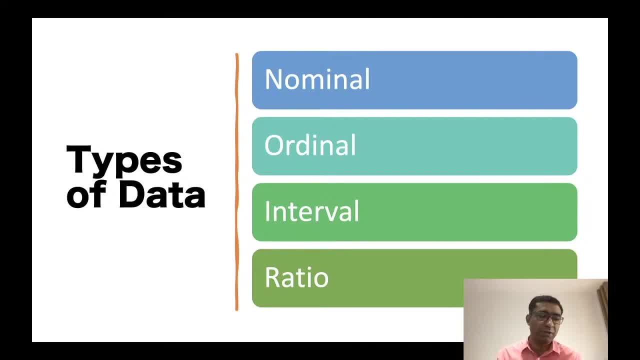 use in the spss. so please make sure when i explain everything it is clear to you. okay, if you have any question you can post in the comment and i will try to answer your question instantly, okay, so here i would take a little break and i request you to post your answer if 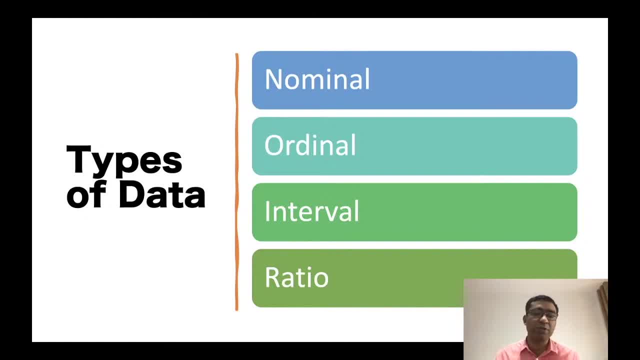 all these scales are very clear to you and you are using it in your research. okay, so just waiting for your reply. please mark your answers and my dear students, one thing we should remember: today i'm not in the mood of listening that particular answer you always give me. if i ask you anything, if you have any question, you should ask. 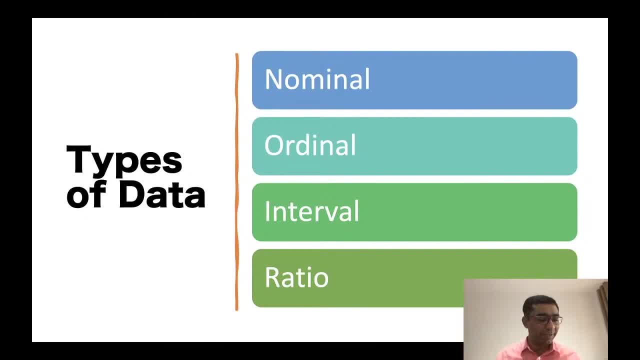 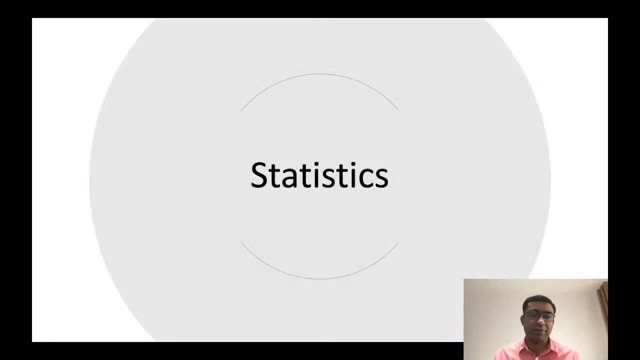 don't be afraid to ask the question. tell me everything is clear. okay, so let's move on. now we are clear about these scales, let's move to the next step. the next step is trying to understand statistics. okay, now, if you try to understand the statistic, there are two major categories of statistics. we call it. one is basically descriptive. 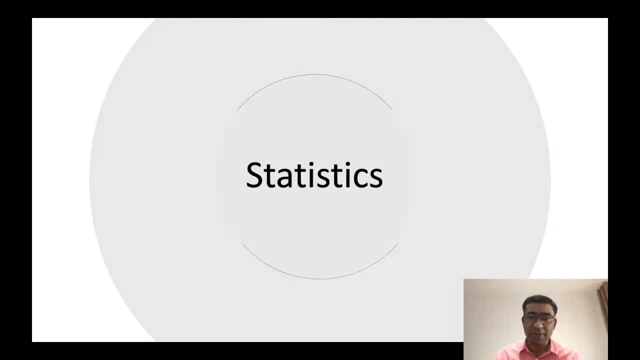 statistics and other is called inferential statistics. okay, now, what is descriptive statistics? now, descriptive statistics is very simple: we are trying to present the data, organize it or summarize it, the information. okay. so me that we are presenting data, we are trying to organize, we are trying to develop some charts or some graphs based on the frequency distribution mean. 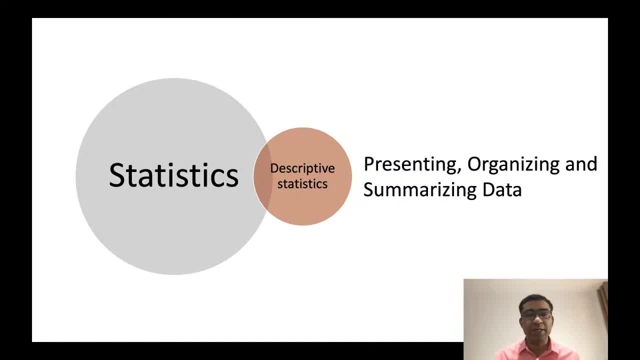 more median. but not much analysis is being done. so what we are doing, we are just taking data and presenting the numbers only. okay, this is the number of male, this is the number of female, this is the number of employed- self-employed, private or government. so we are just taking the data and representing it and organizing it in a 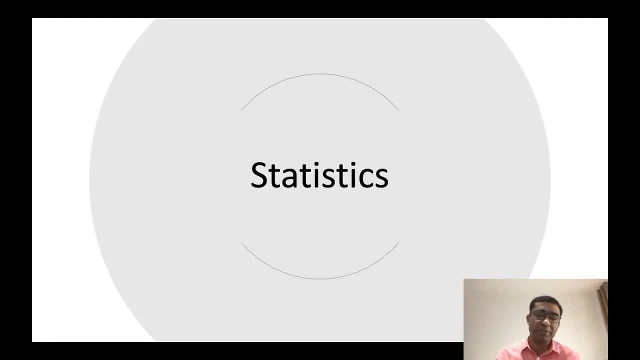 the statistic. there are two major categories of statistics we call it. one is basically descriptive statistics and other is descriptive statistics, is called inferential statistics. okay, now, what is descriptive statistics? now, descriptive statistics is very simple. we are trying to present the data, organize it or summarize it. the information, okay, so mean that we are. 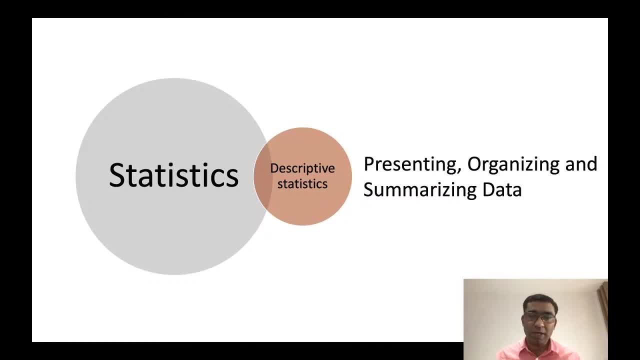 presenting data. we are trying to organize, we are trying to develop some charts or some graphs based on the frequency distribution, mean more median, but not much analysis is being done are doing. we are just taking data and presenting the numbers. okay, this is the number of male. this: 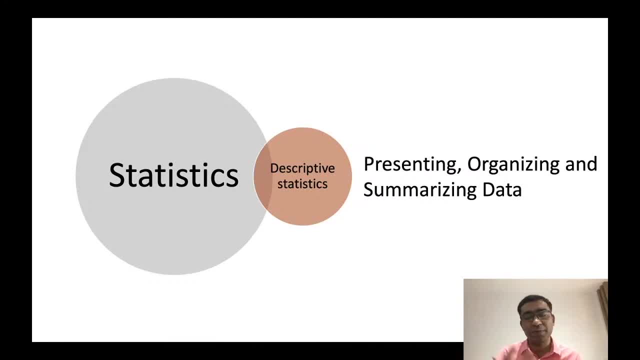 is the number of female. this is the number of employed, self-employed, private or government. so we are just taking the data and representing it and organizing it in a format in which we can understand the numbers very effectively or very clearly. okay, now remember: descriptive statistic does not deal with the hypothesis testing or any other inferential analysis. it 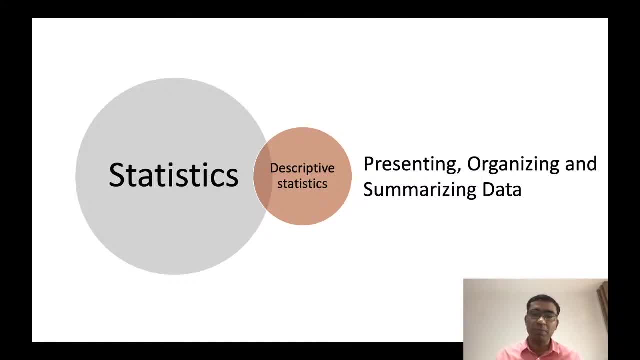 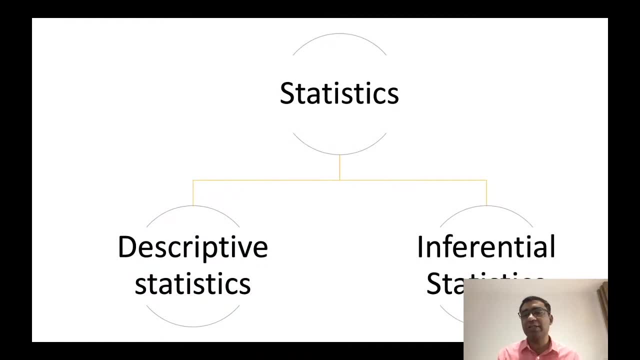 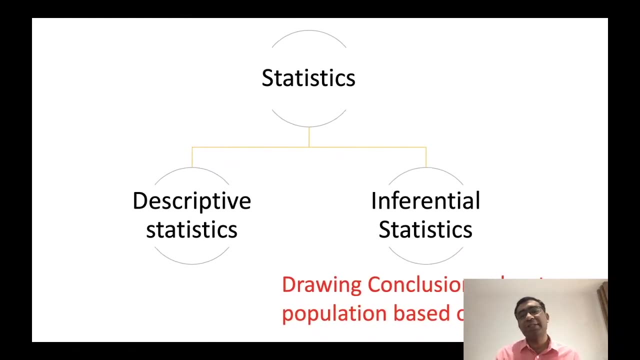 just deal with the frequency distribution, need more, mean more median variation and all this. i will explain it later on. okay now, the second type of the statistics is called inferential statistics. okay now, inferential statistics is interesting. it is basically your hypothesis. testing is included in the inferential statistic. 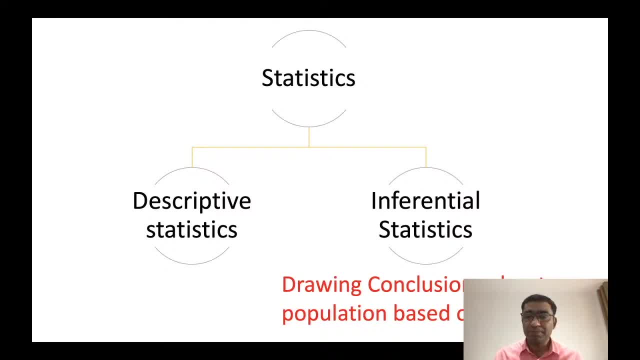 basically inferential statistics. take sample, do the analysis and try to predict the future. or try to predict the prediction for whole population. okay so, in simple word, drawing conclusion about a population based on the sample we collected. okay so inferential statistics is different than the descriptive statistics. in the inferential statistics we do decisions, we do predictions, we do. 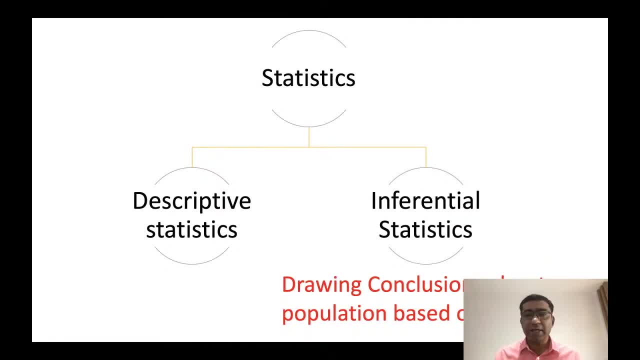 uh, forecasting, we are trying to analyze the behavior of a population based on the sample. we draw from a limited sample, we draw from the population, so this is called inferential statistics. okay, clear. so descriptive is just the presentation of data and inferential it is based on the 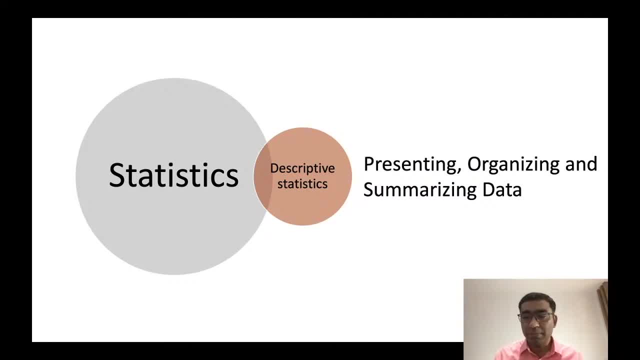 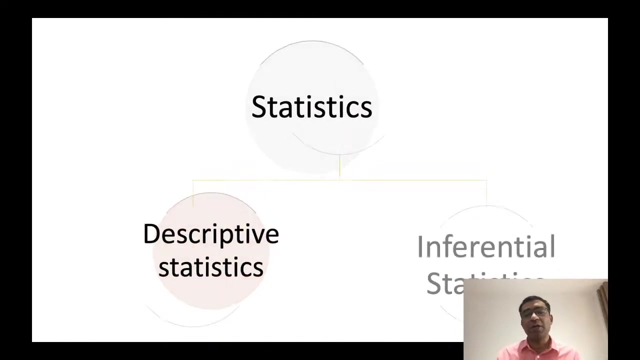 format in which we can understand the numbers very effectively or very clearly. okay now, remember, descriptive statistics does not deal with the hypothesis testing or any other inferential analysis, it just the frequency distribution, need more mean, more median variation and all this. I will explain it later on. okay now the second type of the statistics is called: 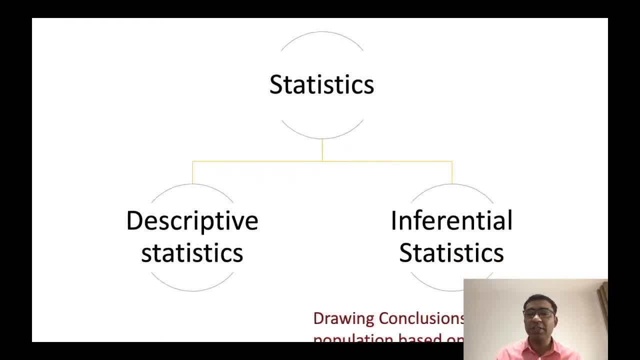 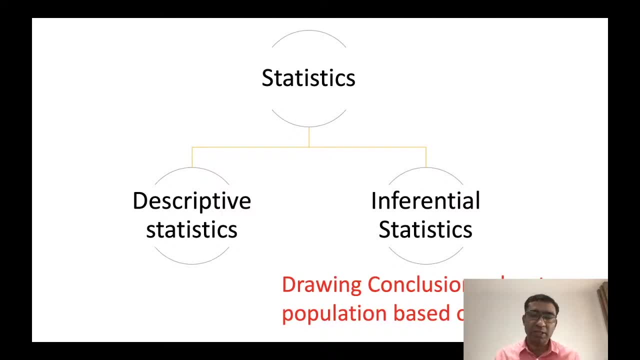 inferential statistics. okay now, inferential statistics is interesting. it is basically your hypothesis. testing is included in the inferential statistic, basically in fresh statistics. take sample, do the analysis and try to predict the future, or try to predict they prediction for whole population. okay, so, in simple word, drawing conclusion about a population based on 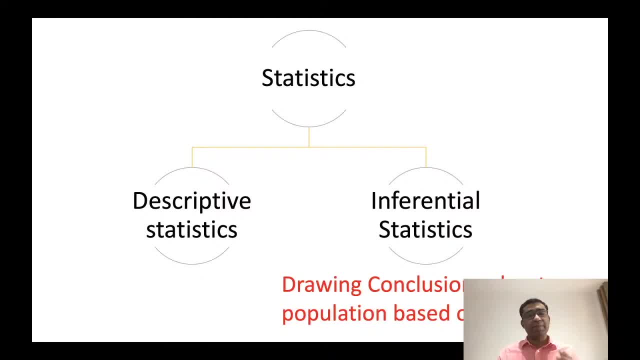 the sample we collected. okay, so inferential statistics is different than the descriptive statistic. in the inferential statistics we do decision, we do prediction, we do forecasting. we are trying to analyze the behavior of population because we try to predict the future as much as possible. so in this 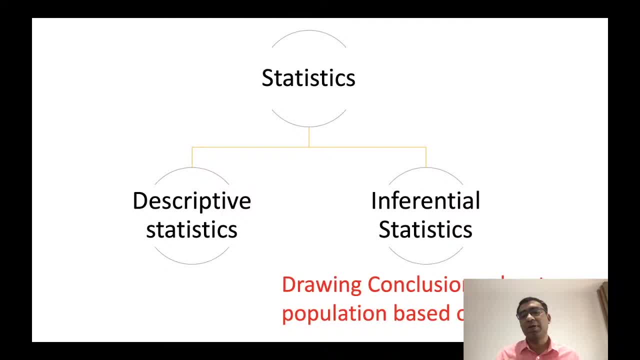 population based on the sample. we draw from a limited sample. we draw from the population, so this is called inferential statistics. okay, clear. so descriptive is just the presentation of data and inferential it is based on the decision making. we are trying to estimate, we are trying to predict or we are trying to. 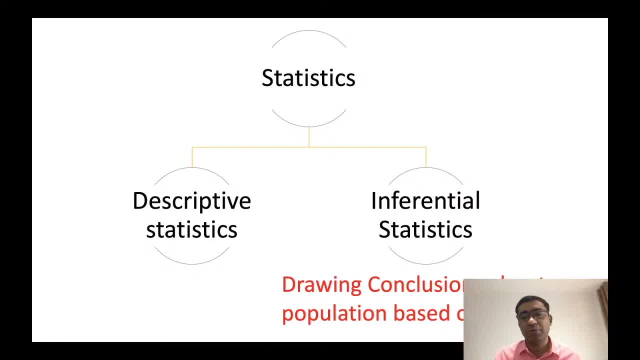 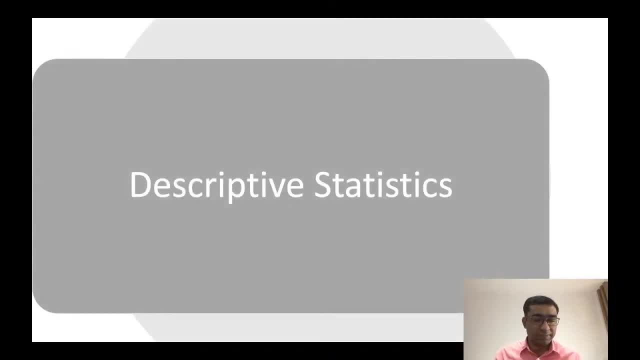 explore, or we are trying to write about, the future. okay, now let's move on to the next point now, the descriptive statistics. what is the descriptive statistics and how it help us in our research, and what are the different forms of the descriptive statistic? let me show you what are the different form. 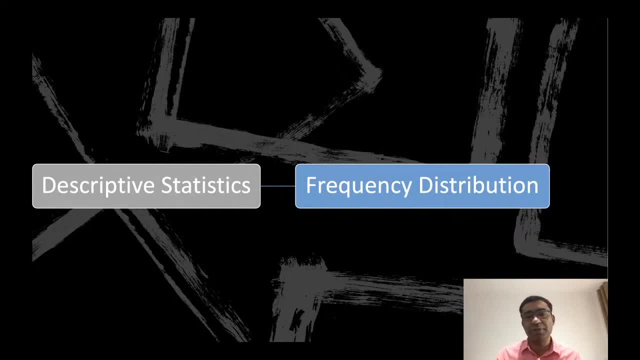 the first thing is frequency distribution. when your scales are nominal, what you can do is you can just tell them: okay, how many, specific group, how many. for example, if we are using male and female, so how many mean how many females? so we can say that, okay, 30% female and 70% male available in my sample size. so this is just a. 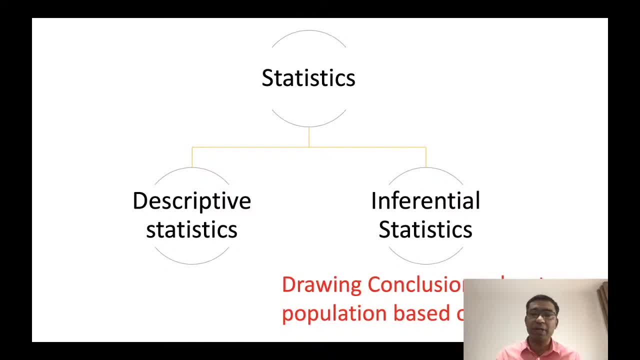 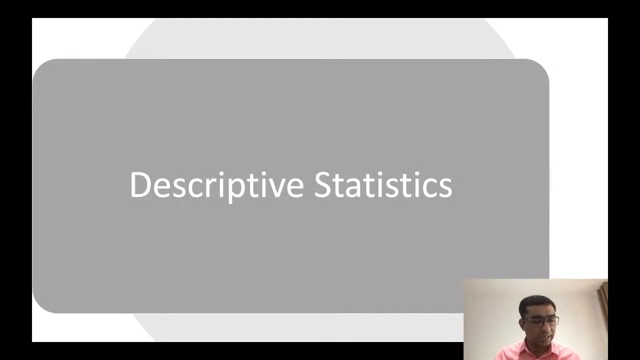 decision making. we are trying to estimate, we are trying to predict or we are trying to explore or we are trying to write about the future. okay, now let's move on to the next point now- the descriptive statistics. what is the descriptive statistics and how it help us in our 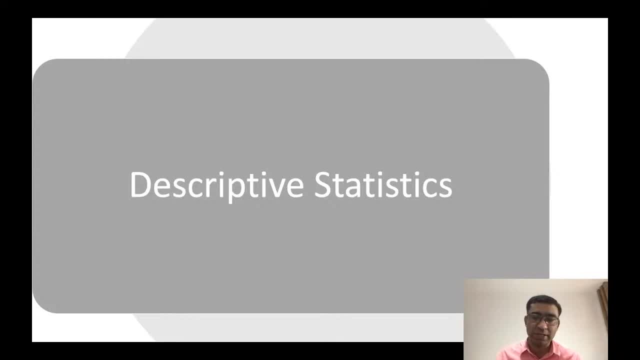 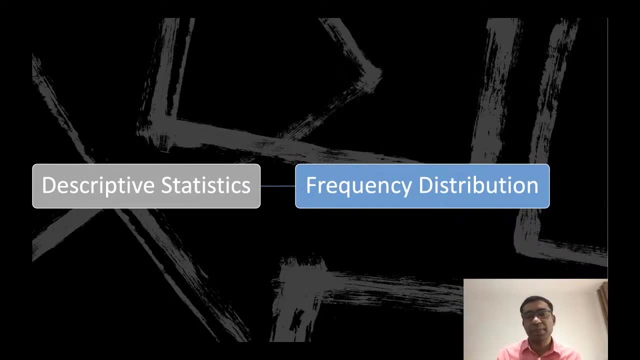 research and what are the different forms of the descriptive statistic. let me show you what are the different form. the first thing is frequency distribution. when your scales are nominal, what you can do is you can use your scales to predict the normal or nominal frequency distribution when just tell them, okay, how many, specific group, how many, for example, if we are. 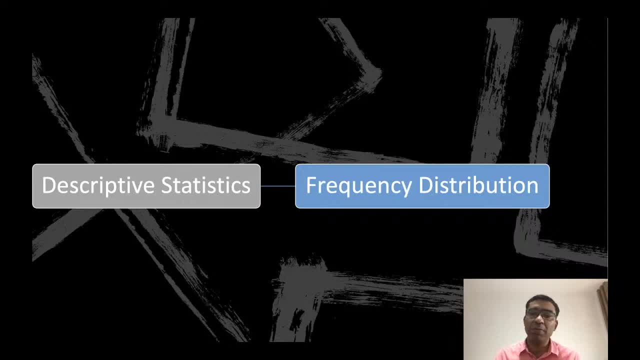 using male and female. so how many mean? how many females? so we can say that, okay, 30 percent female and 70 percent male available in my sample size. so this is just a description or it is just a detail of our data or our sample which we collected and we are just trying to give the frequency distribution. okay, 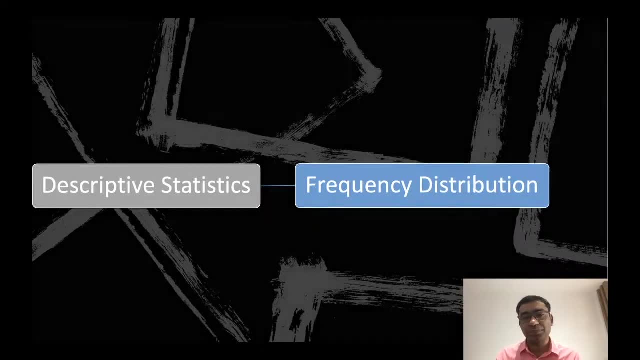 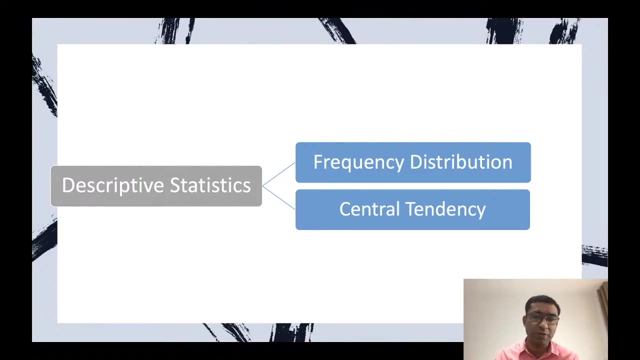 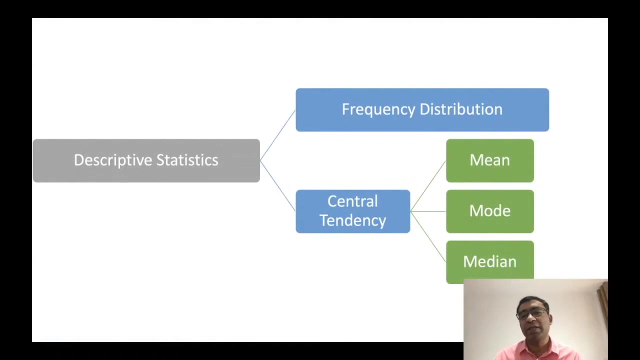 based on the number of available option in one. okay now the second one is central tendency. so in descriptive statistics either you can do frequency distribution or you can do central tendency. measures of central tendency there are three. these are mean mod of median. I think everybody knows about. 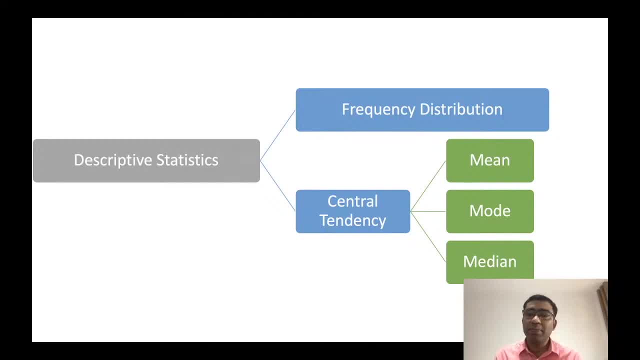 these three numbers or three names, mean is basically an average. so we can take an average. so we can take an average. mod is the most frequent number, the number which is most repeated in your data. okay, for example, if you selected one, two, three, four, five is your liquid. 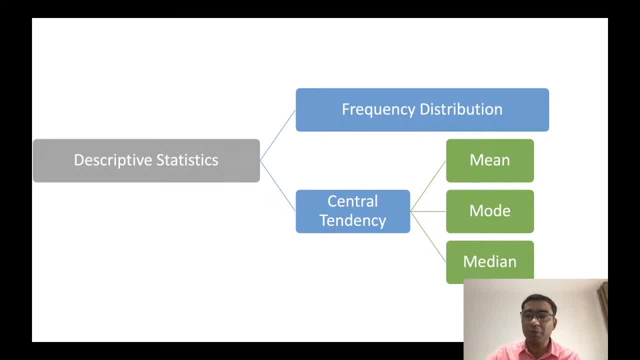 scale and the mostly people they replied you for. the four would be the mod. okay, so the mod is the more frequent number, the most frequent value of frequent number in your data. is called mode, okay, clear. and then the median. the median is simple. median is basically the middle value of your data, okay, so if you will, 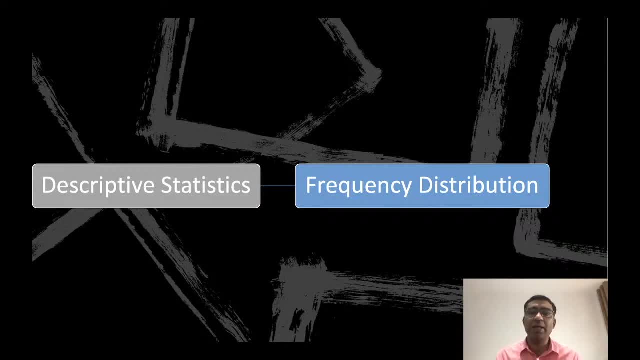 description or it is just a detail of our data or our sample which we collected and we are just trying to give the frequency distribution okay, based on the description. so this is a description of the data, our sample. i suppose why these physical activities arelean. this feature is based on theジャ Str 다. 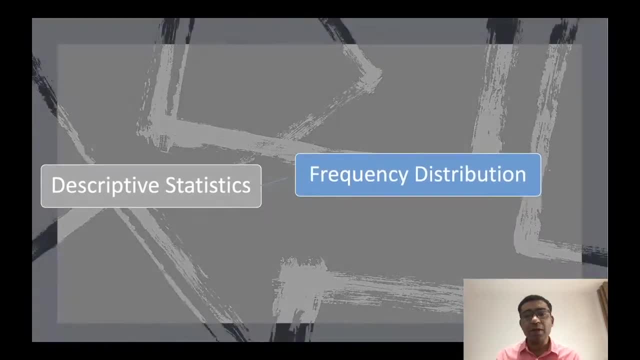 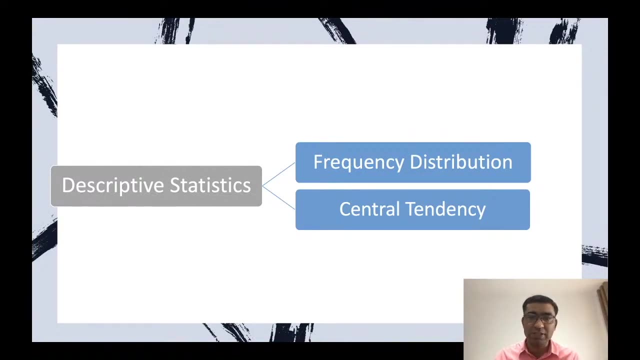 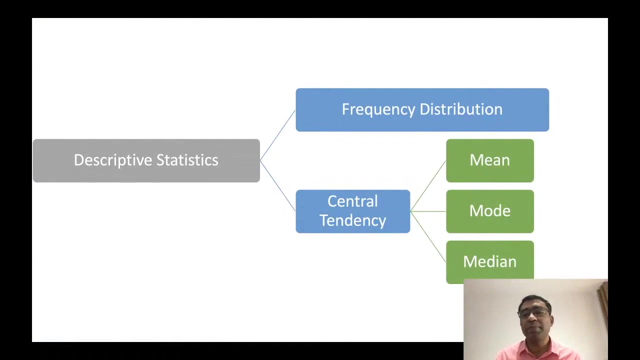 the number of available option in one group. okay now the second one is central tendency. so in descriptive statistics either you can do frequency distribution or you can do central tendency. measures of central tendency there are three. these are mean, mod or median. i think everybody knows about these three numbers or three names. mean is basically an average, so we can take an average. 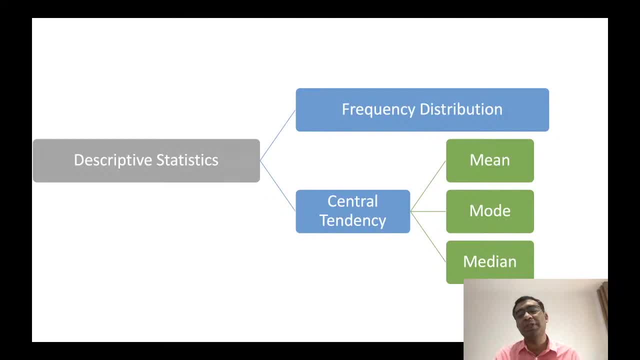 mod is the most frequent number, the number which is most repeated in your data. okay, for example, if you selected 1, 2, 3, 4, 5 is your liquid scale and the mostly people they replied you 4. the 4 would be the mod. okay, so the mod is the more frequent number, the most frequent value of. 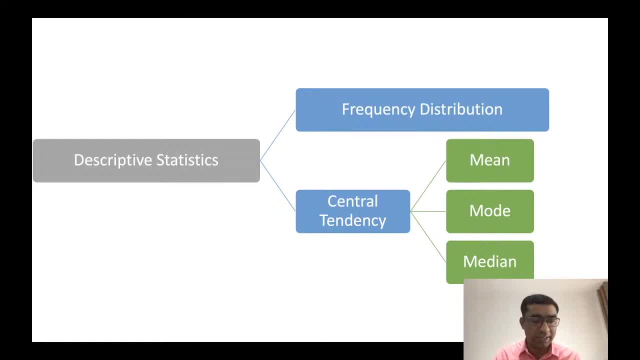 frequent number in your data is called mod- okay, clear. and then the median- okay, median is simple. median is basically the middle value of your data. okay, so if you will divide your data into two values, 50 percent and 50 percent, the middle value would be called as a. 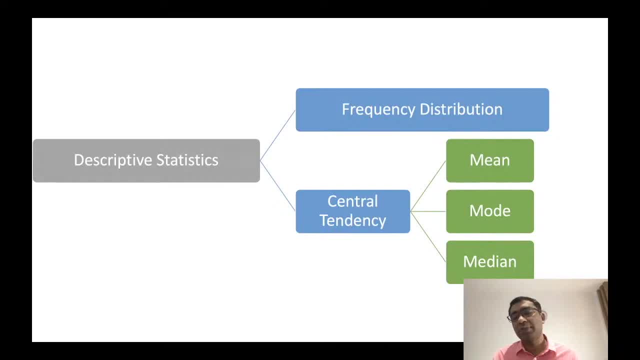 median. okay, so these all are called measurements of central tendency. okay, is it clear? okay, if it is clear, let's move on the next one. okay, i'm not going into the details of how we can measure it, because we are going to use the softwares to measure it, but you have to understand the structures. so it's a simple measure, okay, so 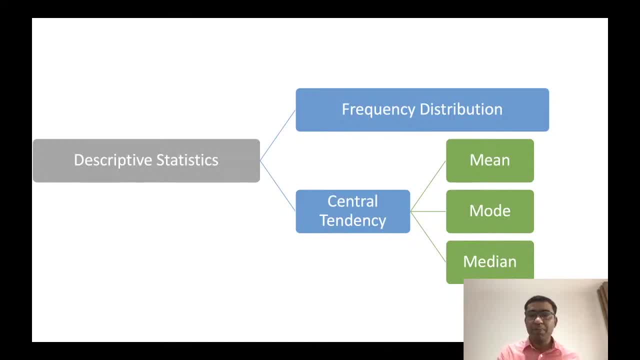 divide your data into two values: fifty percent and fifty percent. the middle value would be called as a median. okay, so these all are called. say it meant measurements of central tendency. okay, is it clear you? okay, then let's move on. okay, the next one. okay, I'm not going into the details. we can measure it, because we are going to use the softwares to measure it, but you have to unconsciously understand how we can measure it, because we use the softwares to measure it, but you have to Netflix. 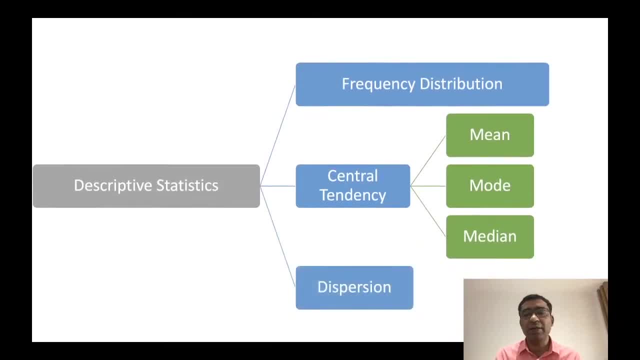 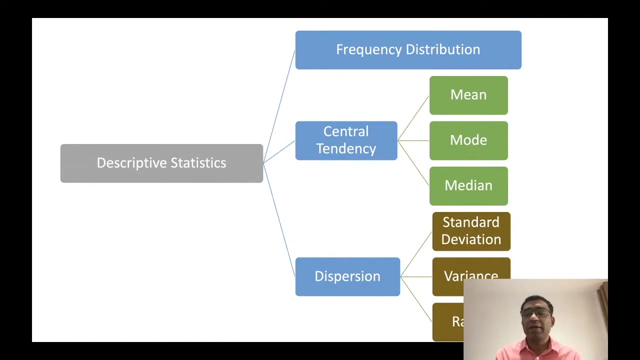 understand what are these values. okay, now the second third part is dispersion. we can measure dispersion based on our descriptive statistics, and dispersion have three different values. okay, you can use standard deviation. standard deviation is simply, if I. I explained it in a very simple word, if you have a mean. 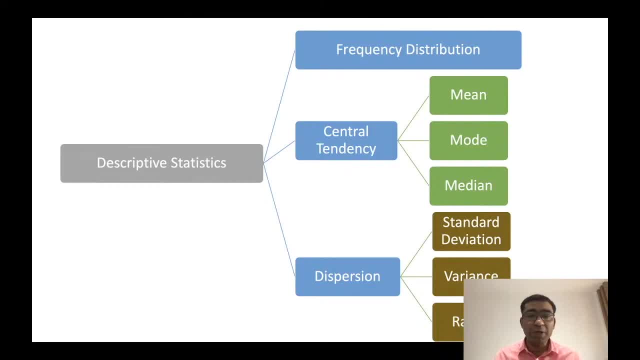 value of 5. so how much other values are separated from the mean value is called standard deviation. for example, the next value is 5.5, so 5 is your mean and 5.5 is the next value, so 0.5 is your standard deviation. okay, so we are trying. 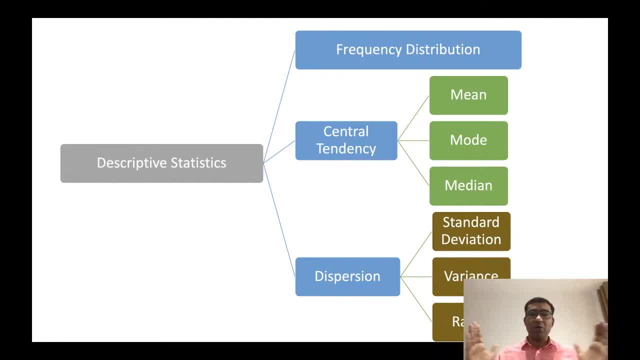 to assess whether your data is scattered or they are very near to the mean. remember, we always prefer the data which is normally distributed based on the standard deviation value. so, for example, distributed or mainly Concentrated around the mean. Okay, so around the central tendency. That is why we have to measure the standard deviation, if your data is too much scattered. 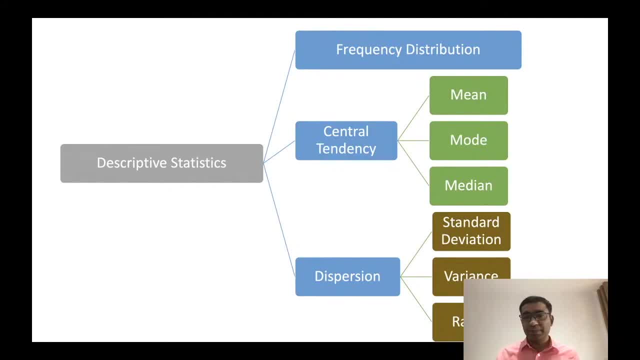 It is difficult for us to measure, To do the inferences. Okay, so we need to have a bell shape or normalize Data, normal distribution. that I will explain in future if I find time on this, but for now you should understand that this my years of. 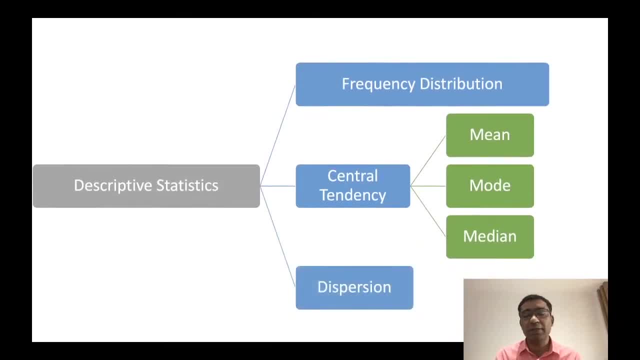 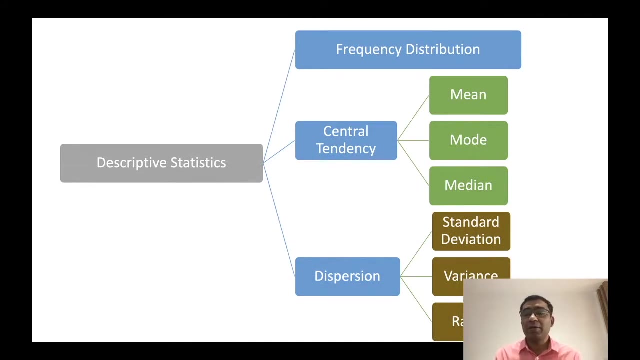 understand what are these values. okay, now the second third part is dispersion. we can measure dispersion based on our descriptive statistics, and dispersion have three different values. okay, you can use standard deviation. standard deviation is simply- if i i explained it in a very simple word- if you have a mean value of five, so how much other values are separated from the mean value is? 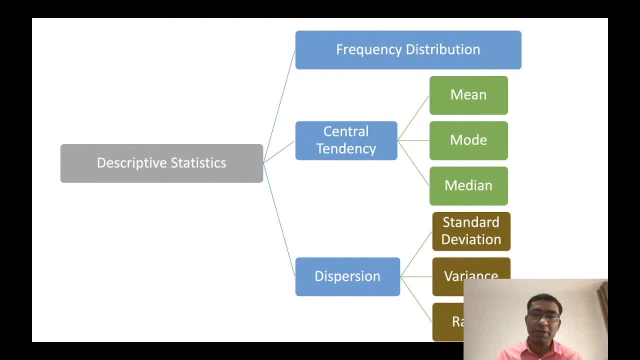 called standard deviation. for example, the next value is 5.5, so 5 is your mean and 5.5 is the next value, so 0.5 is your standard deviation. okay, so we are trying to assess whether your data is scattered or they are very near to the mean, remember. 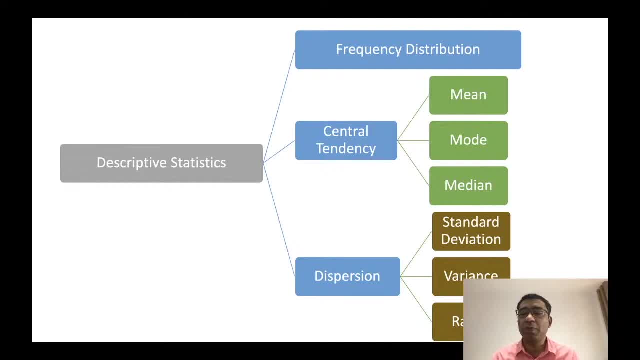 we always prefer the data which is normally distributed or mainly concentrated around the mean, okay, so around the central tendency. that is why we have to measure the standard deviation. if your data is too much scattered, it is difficult for us to measure, uh to do the inferences. okay, so we need to have a bell shape or normalize data. normal distribution- that i will. 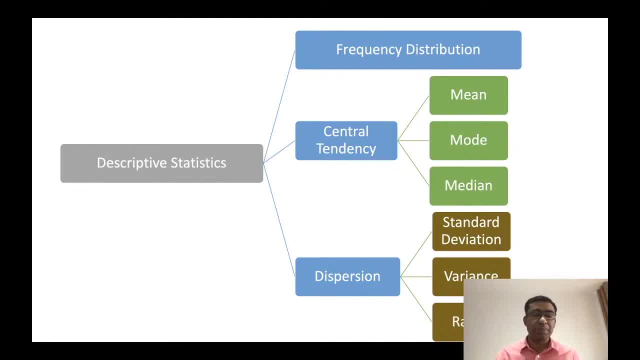 explain in future if i find time on this, but for now you should understand that this measures of central tendency and then dispersion. dispersion is basically the variance. so we have standard deviation- how much your data is scattered around your mean- and then we have variation, or variance. variance is basically uh, how much your uh data is uh, very mean that it have. 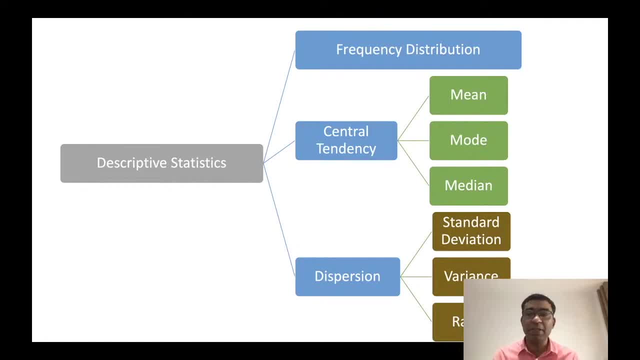 different values. okay, so how much is the difference between the? each value is called variance. okay, so means that average variation means that one value and the second value, how much they are different from each other? okay, and the range is basically, uh, the length of the data, for example in: 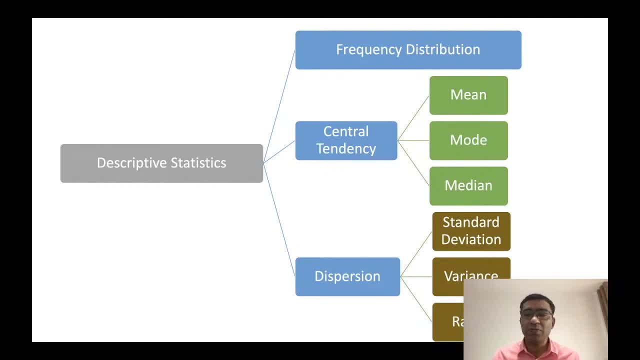 in your lickert scale. if you use uh one to five scales and your respondent, they give only uh option. nobody choose uh option. one means one, so one is not available in your data. but the people they choose 2 and some people they choose 5. so 5 minus 2, 3 would be your range. okay, so the range is the data. 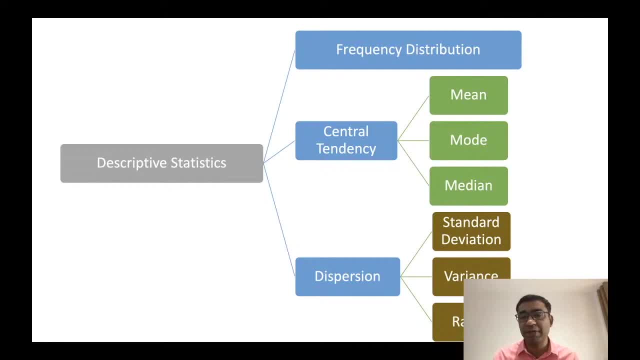 Center tendency and then dispersion. dispersion is basically the variance. So we have standard deviation- how much your data is Scattered around your mean- and then we have variation or variance. variance is basically how much your data is very mean that it have Different values. Okay, So how much is the difference between the? each value is called variance. 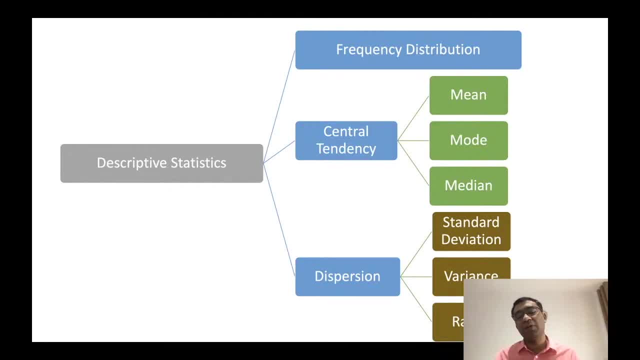 Okay, So means that average variation means That one value and the second value how much they are different from each other. Okay, and the range is basically That the length of the data. for example, in in your Likert scale, if you use one to five Scales and your respondent, they give only 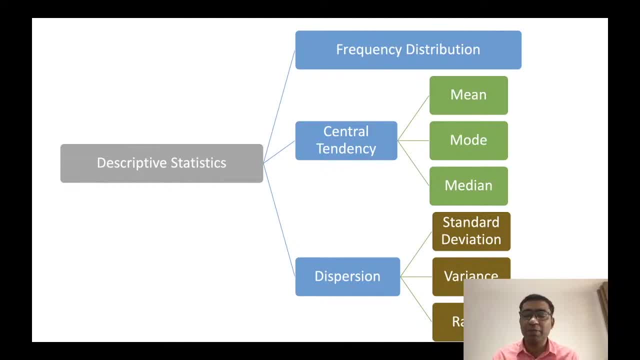 option. Nobody choose option. one means one, So one is not available in your data. But the people they choose two and some people they choose five. So five minus two, three would be your range. Okay, so the range is the data. the consistency of the data mean that and the lowest value and the maximum value, so the 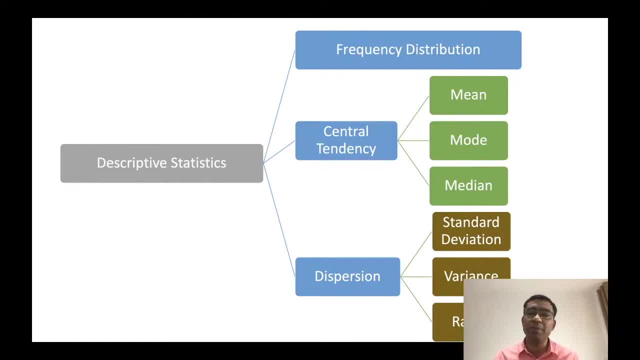 The difference between the maximum and the minimum value is called your range. So we can see that how much is the range of our data? That is also an important measure of dispersion. okay, So dispersion is scatteredness. how you are much, your data is scattered from the mean. 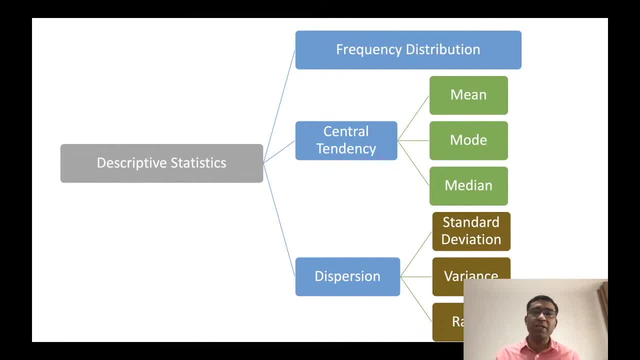 So in the descriptive statistics we can do very simple thing: frequency, distribution, Myers of central tendency and dispersion. Okay, please remember these Names because we are going to calculate these all today and we are going to see how we can interpret them. Okay, Now remember, I am NOT going to give you any. 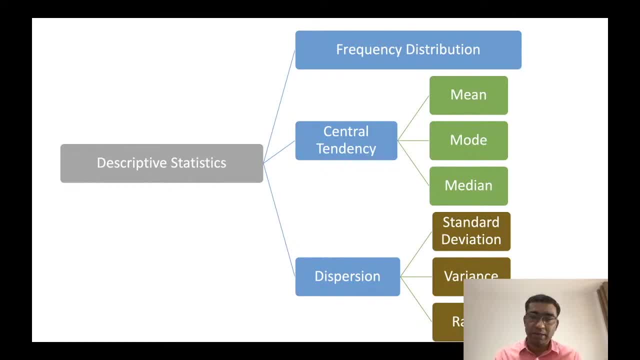 information on how we can write the interpretation. I will explain and My explanation you have to write by yourself. Okay, I will explain everything and you have to write it for you and for your examination also. So make sure You have done with this Standard, deviation, variation and the range. I think all of you are clear on this. So can we move on? 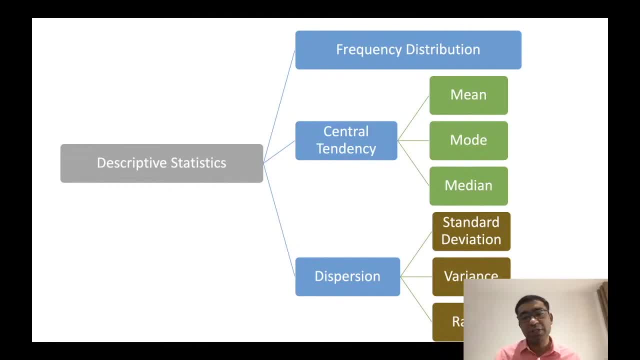 the consistency of the data means that and the lowest value and the maximum value. so the, the difference between the maximum and the minimum value is called your range. so we can see that how much is the range of our data? that is also an important measure of dispersion. okay, so dispersion. 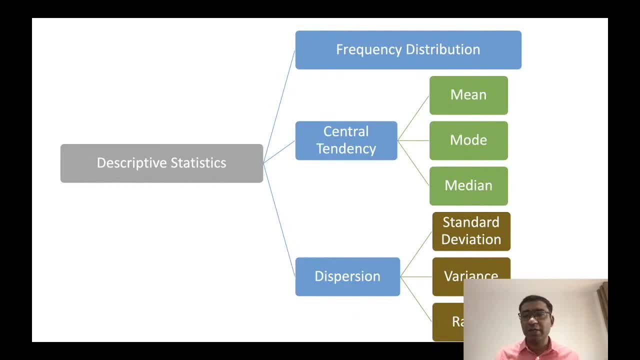 is scatteredness, how your much your data is scattered from the mean. so in the descriptive statistics we can do very simple thing: frequency, distribution, measures of central tendency and dispersion. okay, please remember these names because we are going to calculate these all today and we are going to see how we can interpret them. okay, now, remember, i am not going to give you any. 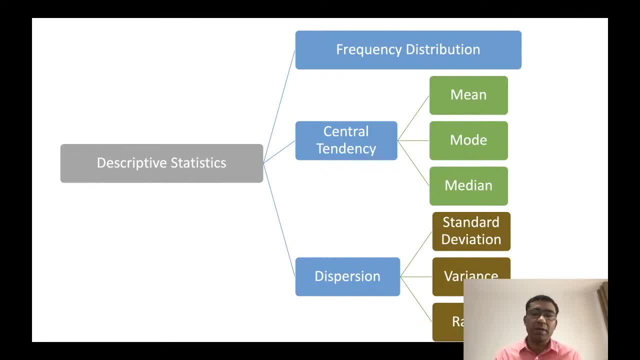 information on how we can uh write the interpretation. i will explain and from my explanation you have to write by yourself. okay, i will explain everything and you have to write it for you and for your examination also. so make sure you have done uh with this standard deviation, variation and the range. i think uh all of you are. 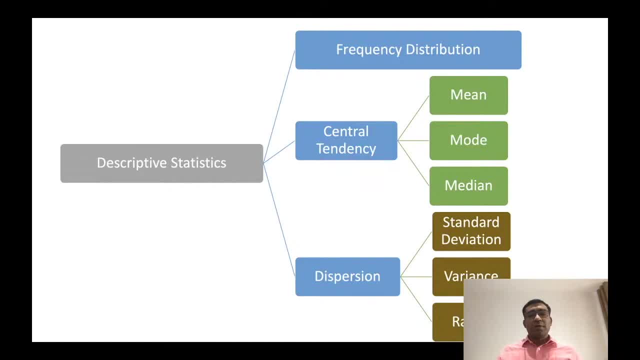 clear on this. so can we move on? so can we uh clear this descriptive statistics. everybody is clear on these three point: frequency distribution, central tendency and dispersion. frequency distribution is just simple measurement of your frequencies or the number of particular group in your sample. and then we have central tendency, which is mean mod median, and then we have 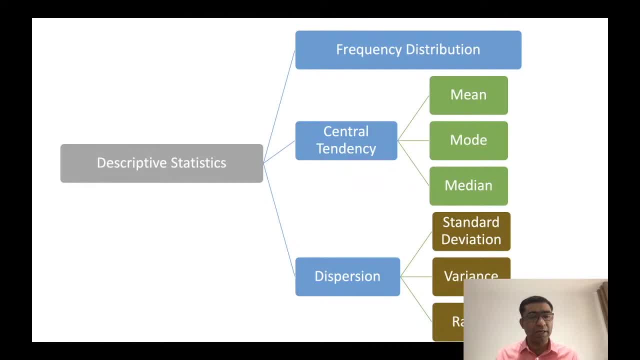 dispersion. dispersion is basically standard, deviation, variation and range. okay, so, i hope so. everybody is uh okay with this. okay, so please remember this: you can write any questions in the comment box and i will give you a link to the given question as well in the following comments. 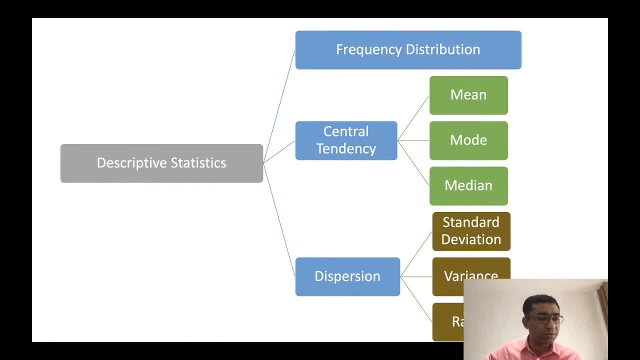 okay, then we will see you in the next one. now let's move on to the next point. so, as you can see, i have two points in front of me for this analysis, and that one is a question about theomme. this is the first point. this is the second one is about the memory. this is the second point. 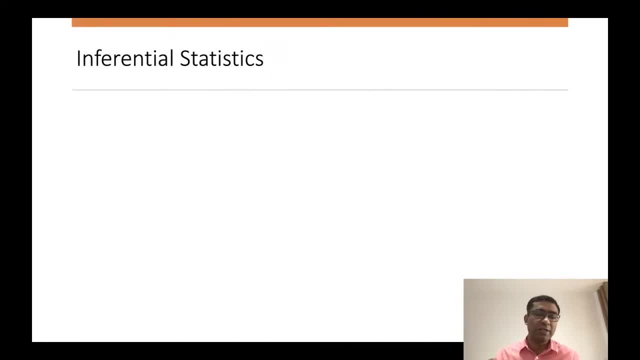 is the number of frequencies that we use, and these are the number of frequencies that we use for the, our number of frequencies that are used in the information that is used in the outputs where we have to do all the analysis, we have to do the decision making. okay, now inferential. 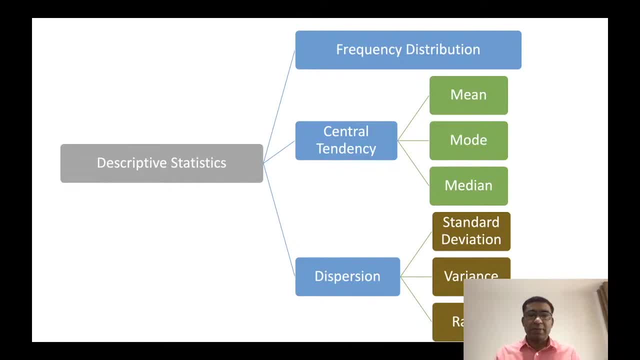 So can we clear this Descriptive statistics? everybody is clear on these three point: frequency distribution, Central tendency and dispersion. frequency distribution is just simple measurement of your frequencies or the number of particular group in your sample. and then we have central tendency, which is mean, mod, median, and then we have 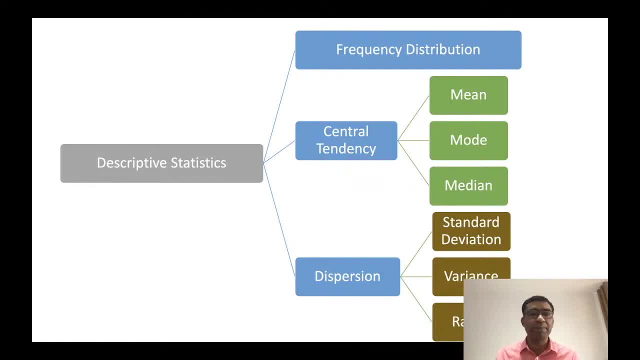 Dispersion. dispersion is basically standard, deviation, variation and range. Okay, so I hope so everybody is okay with this. Okay, Any question here? If you have any question, you can write in the comment box so I can reply to your answer your question. if you have any question, you can write in the comment box so I can reply to your answer your question. 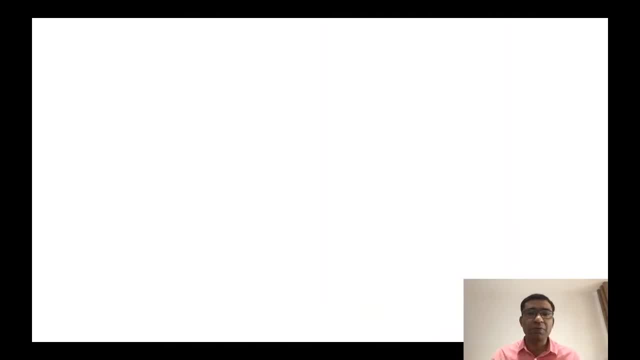 Okay, if this point is clear, let's move on to the next point. the next point is Understanding the inferential statistics. that is the main point where we have to do all the analysis. analysis, we have to do the decision making. okay now, inferential statistics is huge. there are so. 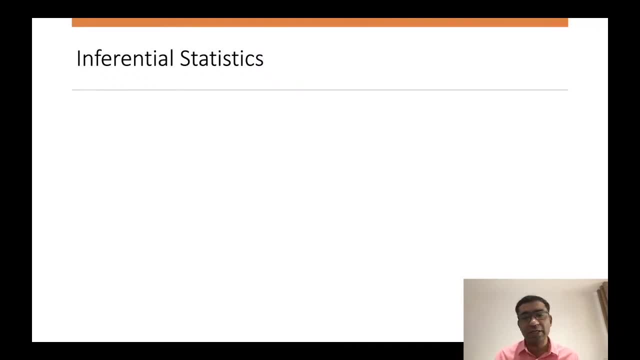 many tests, so many different inferential statistics are available: parametric, non-parametric, a lot of inferential statistics is available. okay, now the point is: according to your research, i will give you very brief introduction of inferential statistics and i will tell you a few tests: which. 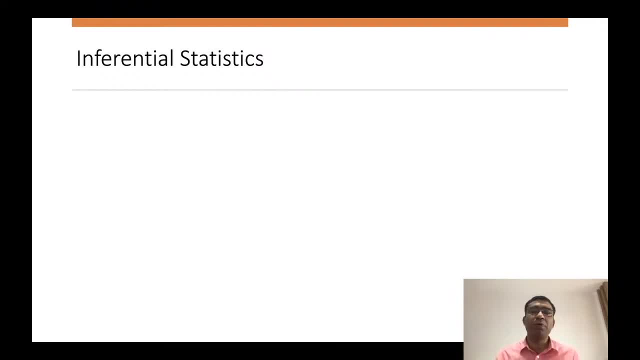 are very important for you in order to do your final year project or do your research article or research paper. so if you are not a statistician, don't worry about this. i will explain everything and we can do it together easily. no problem with that, okay? so make sure, uh, you are clear about. 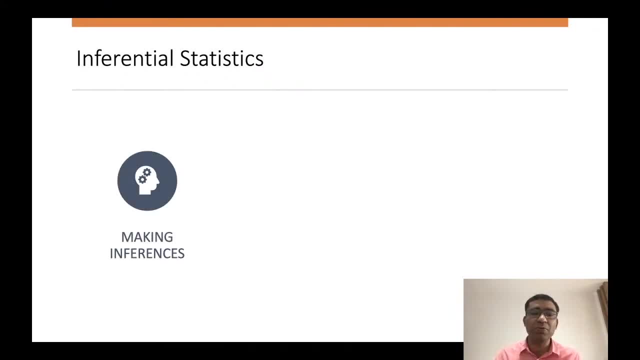 the inferential statistics. now, inferential statistics, why we do? because we need to make inferences, we need to make predictions, we need to hypothesize, hypothesis testing, and we need to determine the relationship between the variable. so all these are main purposes of inferential statistics. so you can see that all the analysis which we do. 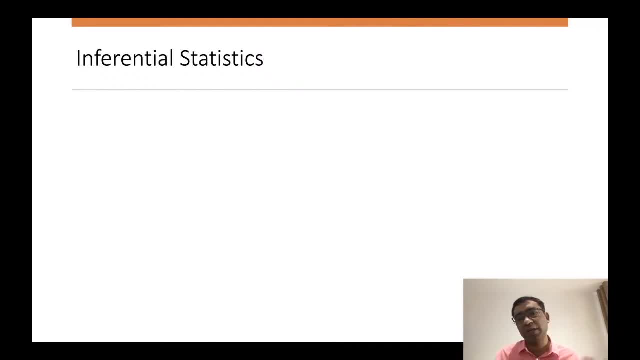 statistics is huge. there are so many tests, so many different inferential statistics are available: parametric, non-parametric- a lot of inferential statistics is available. okay, now the point is, according to your research, i will give you very brief introduction of inferential statistics and i will tell you a few tests which are very important for you in order to 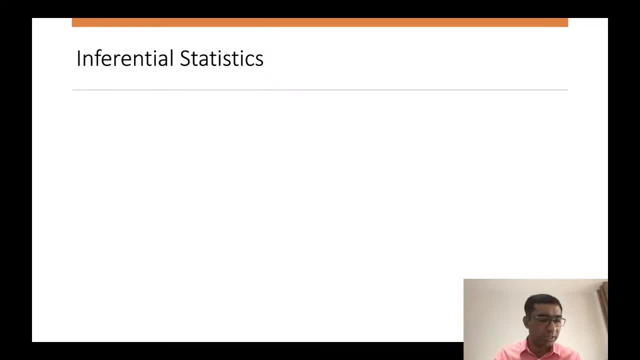 do your final year project or do your research article or research paper. so if you are not a statistician, don't worry about this. i will explain everything and we can do it together easily, no problem with that, okay, so make sure, uh, you are clear about the inferential. 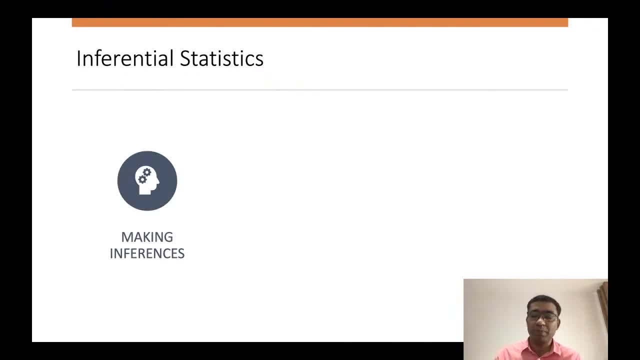 statistics, now inferential statistics. why we do? because we need to make inferential, we need to make predictions, we need to hypothesis testing and we need to determine the relationship between the variable through all these are main purposes of inferential statistics. so you can see that all the analysis which 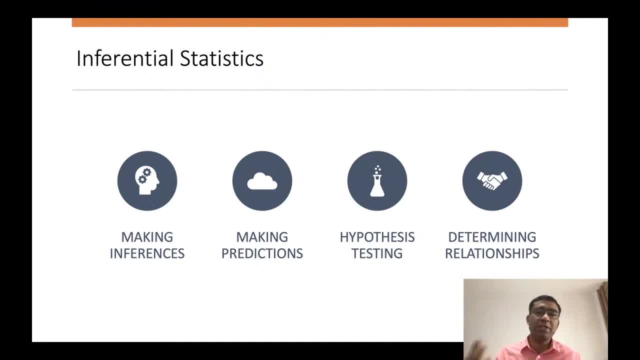 we do is here. frequency, distribution or descriptive is just a representation of data. it is important, but not important like inferential statistics. without inferential statistics you are not able to predict for your whole population from your sample okay. so that is why inferential statistics is very important. 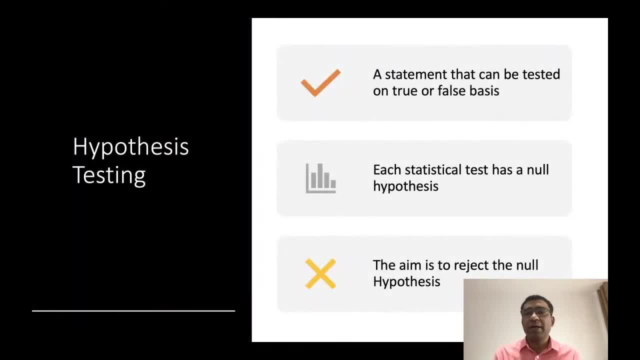 now let's move to the next point: hypothesis testing. so what is hypothesis testing, which we are trying to do on today's lecture with the help of SPSS software? so what is hypothesis testing? now? if you remember, I asked you to develop hypothesis and everybody have their own hypothesis according to their research. so that is. 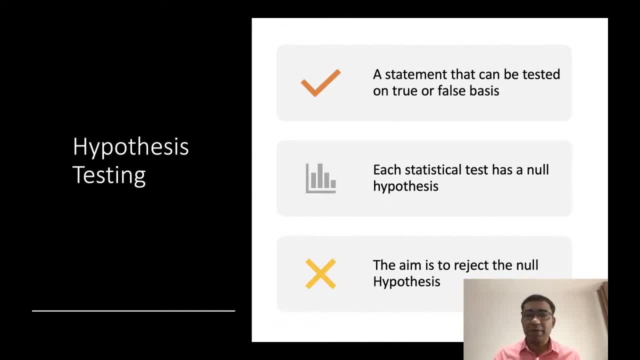 your hypothesis. now, this is a statement. hypothesis is a statement. I mentioned this so many time. hypothesis is a statement that can be tested- or true or false basis. okay, so we have to mention whether our hypothesis is true or false based on the evidence we collected in the form of. 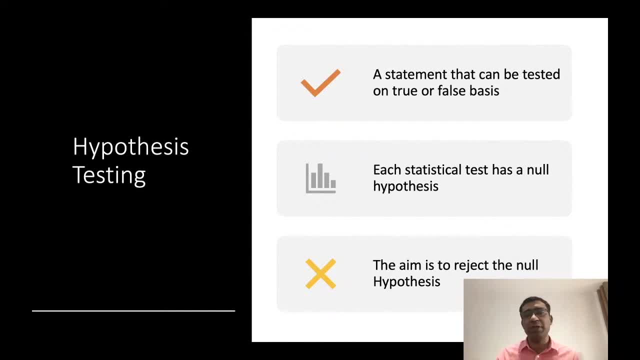 data. okay, so we do some inferential statistics and then we reject the, our hypothesis or null hypothesis. but here You have to remember one very, very, very important point: Each test, because we have a lot of statistical tests. Okay, So each test, have a null. 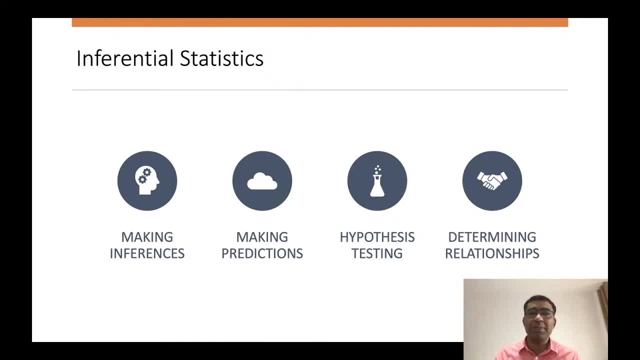 is here. frequency, distribution or descriptive is just a representation of data. it is important, but not important like inferential statistics. without inferential statistics, you are not able to predict for your whole population from your sample, okay. so that is why inferential statistics is very important. now let's move to the next point. 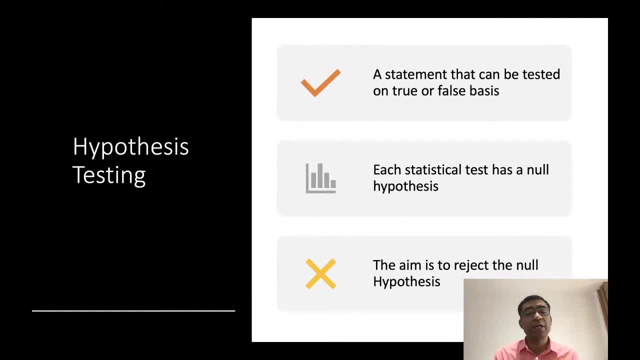 hypothesis testing. so what is hypothesis testing, which we are trying to do on today's lecture with the help of spss software? so what is hypothesis testing? now, if you remember, i asked you to develop hypothesis and everybody have their own hypothesis according to their research. so that is your hypothesis. 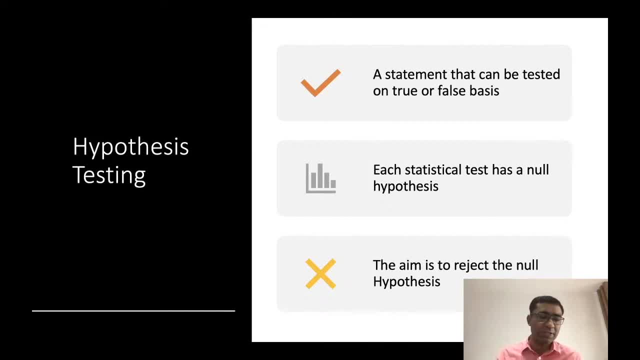 now, this is a statement. hypothesis is a statement. i mentioned this so many time. hypothesis is a statement that can be tested, or true or false basis. okay, so we have to mention whether our hypothesis is true or false based on the evidence we collected in the form of data. okay, so we do some. 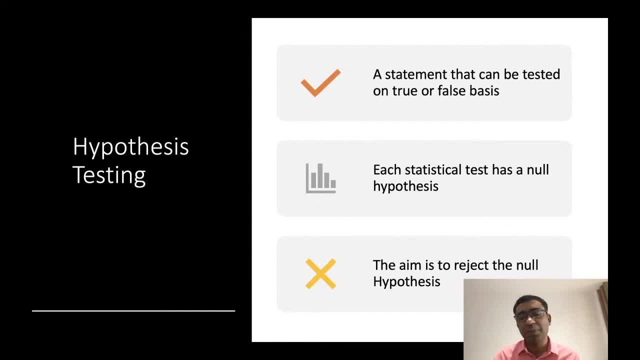 inferential statistics and then we reject our hypothesis or null hypothesis. but here you have to one very, very, very important point: each test, because we have a lot of statistical tests. okay, so each test have a null hypothesis. okay, remember this point: each test have a null hypothesis, so we can't change that null hypothesis. 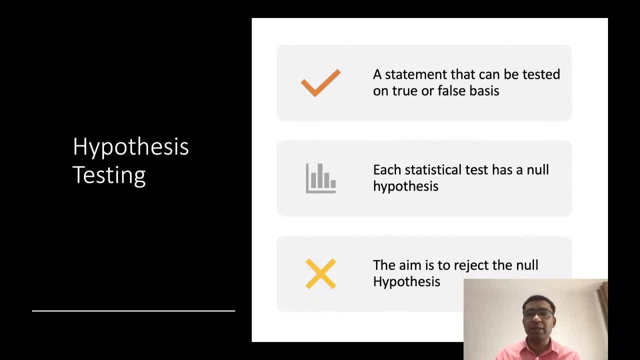 we have to learn what to do with this statistical analysis. we cannot shape our own hypothesis based on our own requirement. just we can analyze and what type of hypothesis is required. but if we are talking about the statistical test, that the hypothesis are already established, so you cannot change much of. 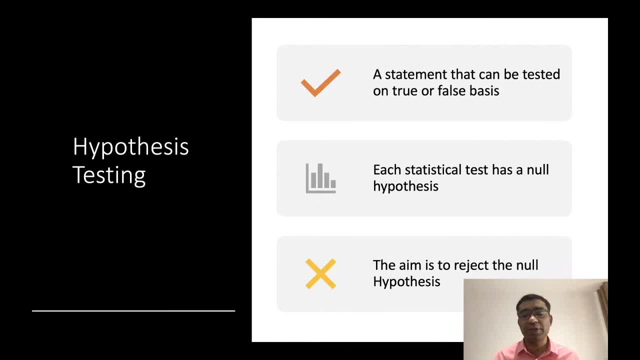 this wording of this hypothesis or much of these chronological explanation of these hypothesis. okay, so you have to understand, because that is possible. but I told you in your hypothesis, I told you you can develop your hypothesis based on a few statements. for example, there is a positive relationship between: 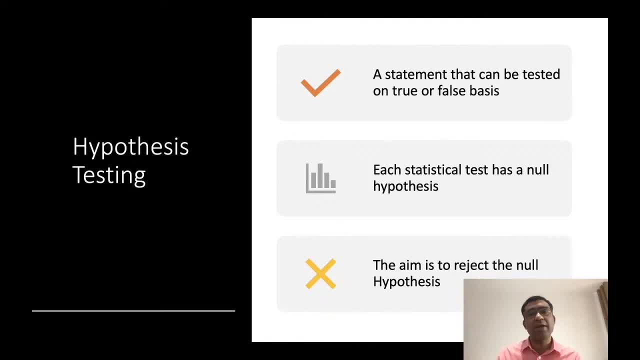 Hypothesis. okay, Remember this point: each test have a null hypothesis, So we can't change that null hypothesis. We have to learn What to do with this statistical analysis. we cannot shape our own hypothesis based on our own requirement. Yes, we can analyze, and what type of hypothesis is required. 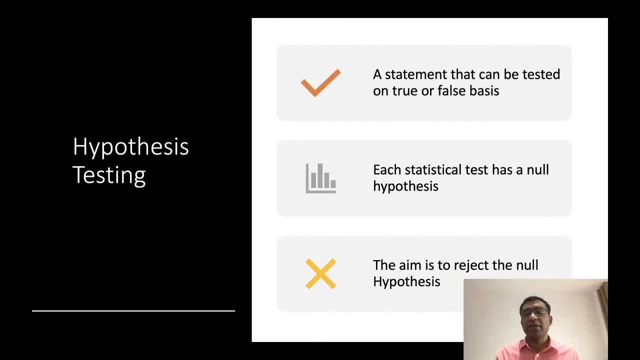 But if we are talking about the statistical test, that the hypothesis are already established. so you cannot change much of this wording of this hypothesis or much of these Chronological Explanation of these hypotheses. Okay, so you have to understand, because that is what I told you in your 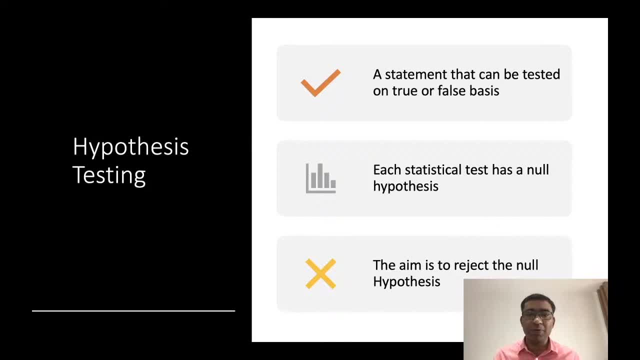 Hypothesis. I told you, you can develop your hypothesis based on a few Statements. for example, there is a positive relationship between a and B. There is a negative relationship between a and B. There is a relationship between a and B. Okay, there is a difference between a and B. 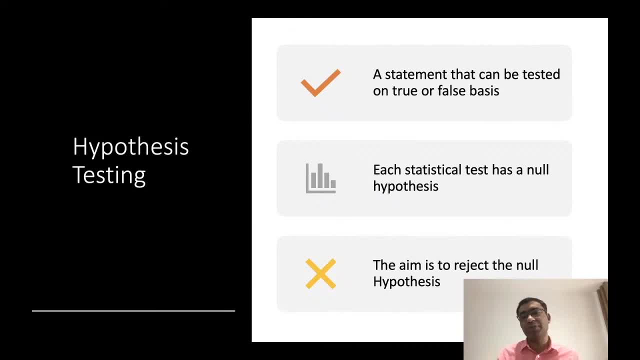 So all These are different types of the hypothesis which we need to understand. they are Directly coming from some test, Okay, some statistical procedures. so that is why we have to understand which type of the statistical test is Applicable to our hypothesis. This is very important. which type of inferential statistics is? 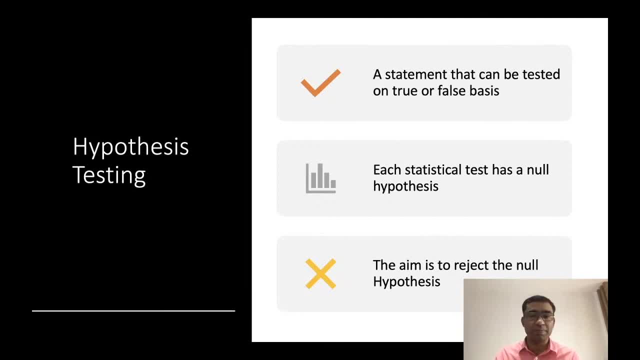 Okay, or is required to test my hypothesis, okay, so you have to clear that part. okay, now let's move to the next point. as I mentioned, each statistical test have its own hypothesis. I will. I will explain while we are doing these hypothesis testing, but remember: 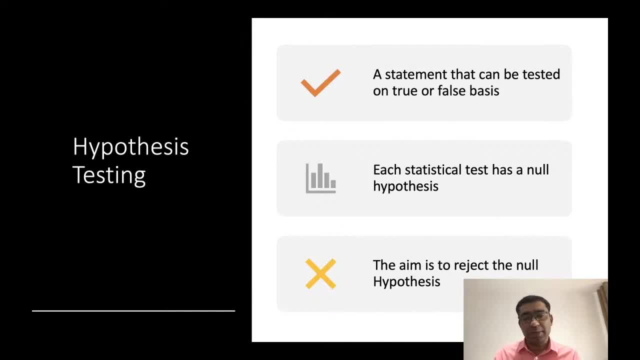 each hypothesis have its own statement and what we are trying to do this is called a null hypothesis. every test have its own null hypothesis. so what we are trying to do is we are trying to reject the null hypothesis and accept the alternative hypothesis. don't worry about the wording. 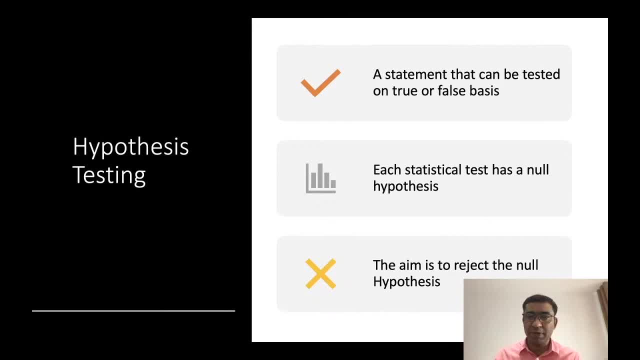 A and B. there is a negative relationship between A and B. there is a relationship between A and B. okay, there is a difference between A and B. so all these are different types of the hypothesis which we need to understand. this. they are directly coming from some test, okay, some statistical procedures, so that 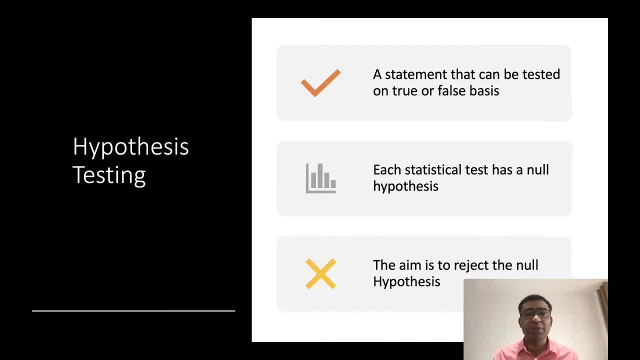 is why we have to understand which type of the statistical test is applicable to our hypothesis. this is very important. which type of inferential statistics is okay or is required to test my hypothesis? okay, so you have to clear that part. okay, now let's move to the next point. as I mentioned in the previous video, we talked about the 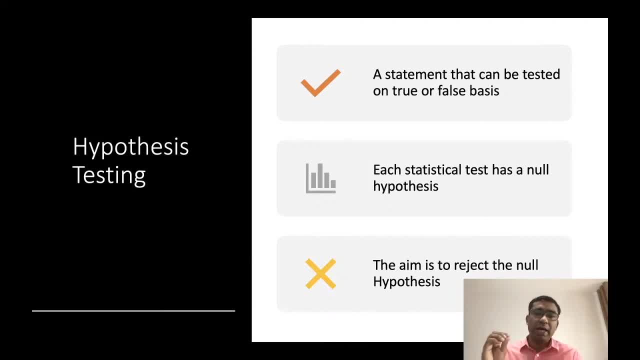 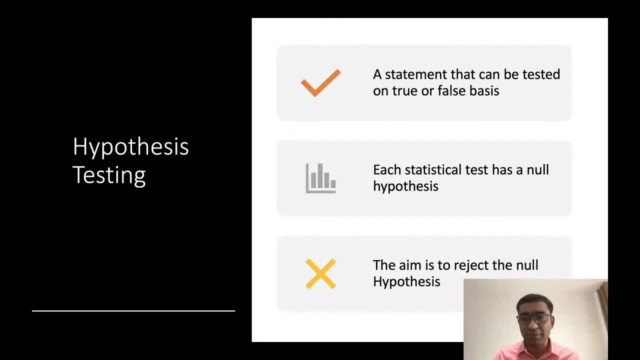 alternative hypothesis are those which you have crafted during your research, so you have already developed the research hypothesis. those research hypotheses are also named as alternative hypothesis. how we are going to test it, i will explain, but here i think we should be clear about the hypothesis testing. now the next question will come into my mind. okay, how i can accept or reject any. 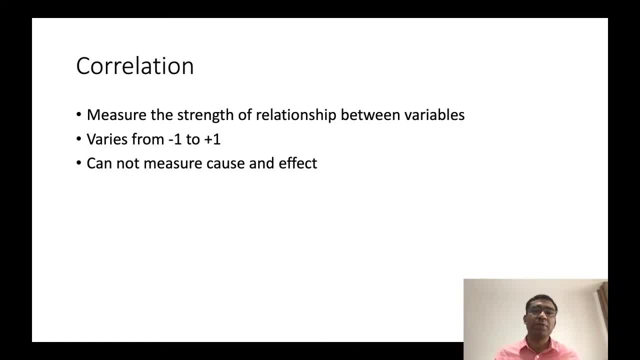 hypothesis. now here comes some very important statistical procedures. i choose only two statistical procedures for today's class and the later we will explain. if it is required. we can do uh another round uh in in any other day, but here i am just talking about the correlations and regressions. okay now, correlations and regressions. what are the? 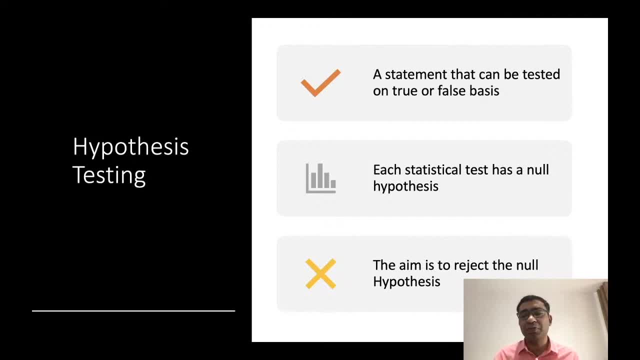 alternative hypothesis are those which you have crafted during your research, so you have already developed the research hypothesis. those research hypothesis are also named as alternative hypothesis. how we are going to test it, I will explain, but here I think we should be clear about the hypothesis testing. now the 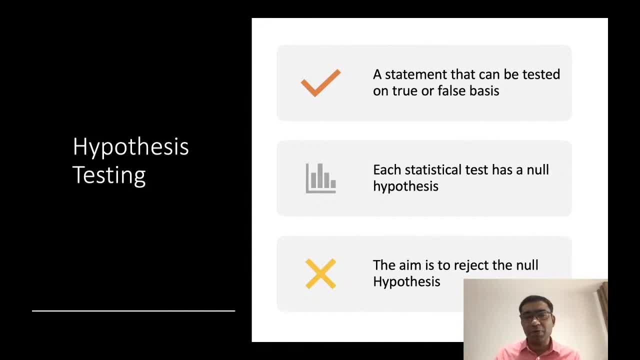 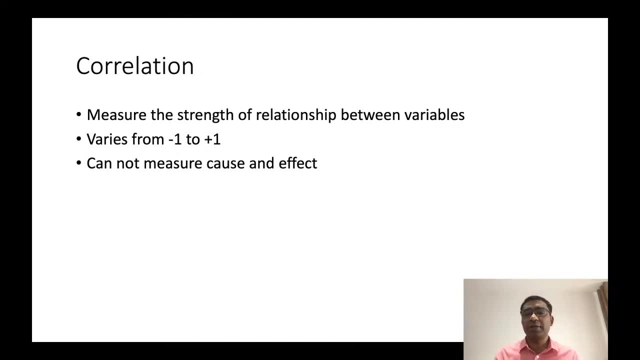 next question will come into my mind: okay, how I can accept or reject any hypothesis. now here comes some very important statistical procedures. I choose only two statistical procedures for today's class and the later we will explain. if it is required, we can do another round in any other. 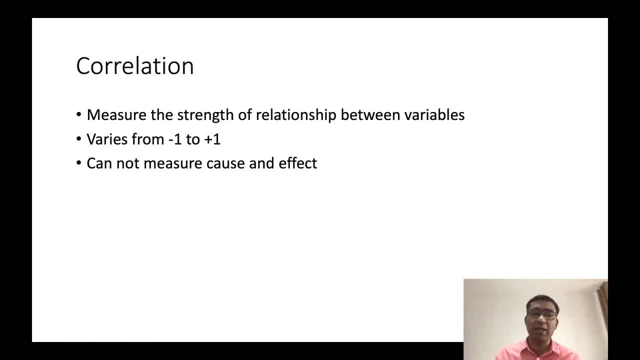 day, but here I am just talking about the correlations and regressions. okay, now, correlations and regressions. what are the correlation? so correlations are the statistical tests which gives us the strength of relationship between two variables. okay, remember it, always have two variables and if the value varies, 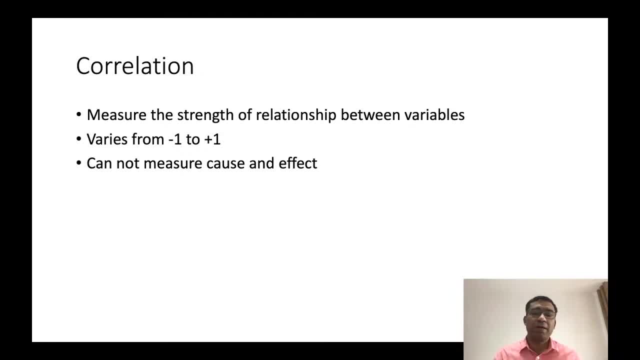 from minus 1 to plus 1. okay, remember, in correlation we have only two variable. there is no independent, there is no dependent variable in correlation. remember, independent and dependent is just in the regression. so if you have independent and dependent variable, you cannot run correlations. okay, you cannot. 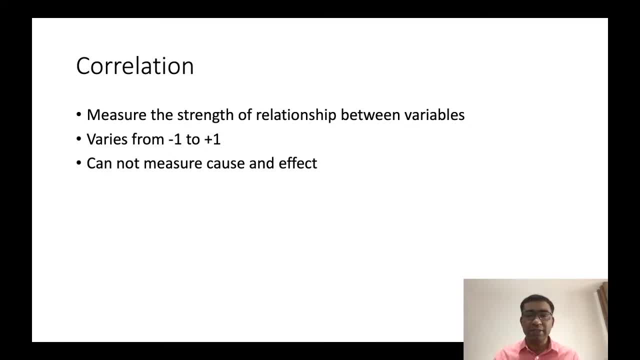 decide your relationship based on the correlation. yes, we do correlation analysis, but just to test the, the correlation, the nature of relationship. but we cannot conclude or we cannot accept or reject our hypothesis based on the correlations. if your variables are dependent and independent, okay, remember, correlation is not able to test the causal relationship. please make sure you understand this point. 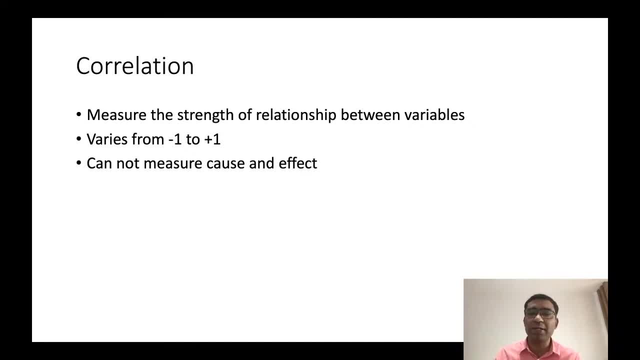 okay, the values of correlation. they are from minus 1 to plus 1. very simple: minus 1 to plus 1. okay now, minus 1 to plus 1 means that minus 1 is strongly negative correlations. when we say negative correlations, it means that one value is increasing while the other value is decreasing. okay, 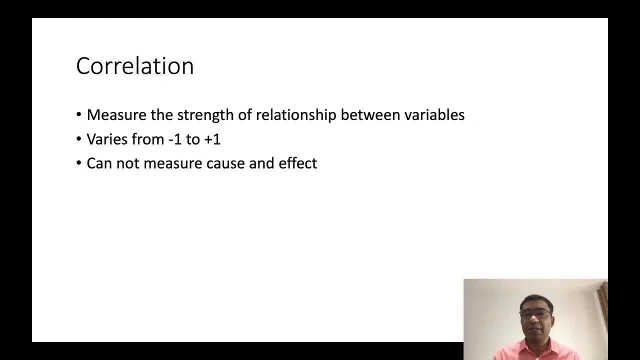 correlations. so correlations are the statistical tests which gives us the strength of relationship between two variables. okay, remember it, always have two variables. and if the value varies from minus one to plus one, okay, remember, in correlation we have only two variables. there is no independent, there is no dependent variable in correlation, remember. 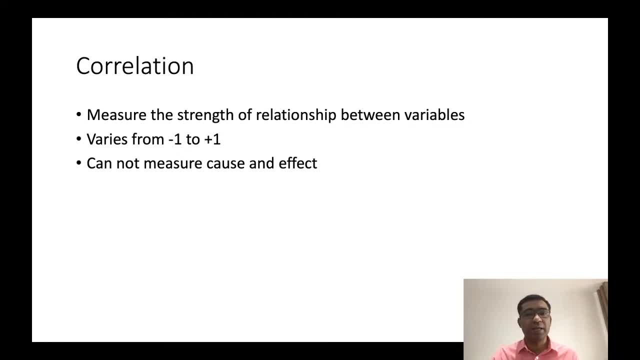 independent and dependent is just in the regression. so if you have independent and dependent variable you cannot run correlations. okay, you cannot decide your relationship based on the correlation. yes, we do correlation analysis, but just to test the nature of relationship. but we cannot conclude or we cannot accept or reject our hypothesis based on the correlations if your variables are. 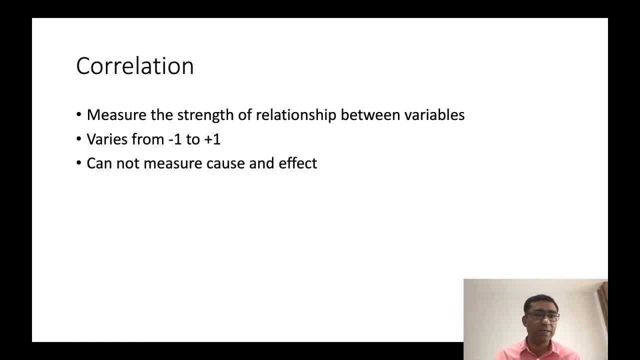 dependent and independent. okay, remember, correlation is not able to test the causal relationship. please make sure you understand this point, okay. the values of correlation, they are from minus one to plus one. very simple, minus one to plus one. okay now, minus one to plus one means that minus one is strongly negative correlations. when we say negative correlations, 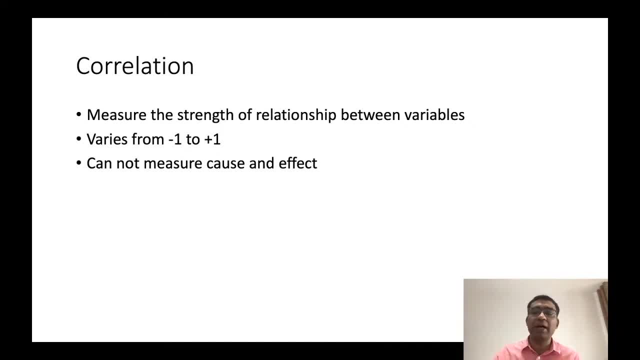 it means that one value is increasing while the other value is decreasing. okay, is it clear? so one value is increasing and other value is decreasing. i will show you in in in the graphical form also. but remember, i mentioned two, three very important things about the correlation. first, it measures. 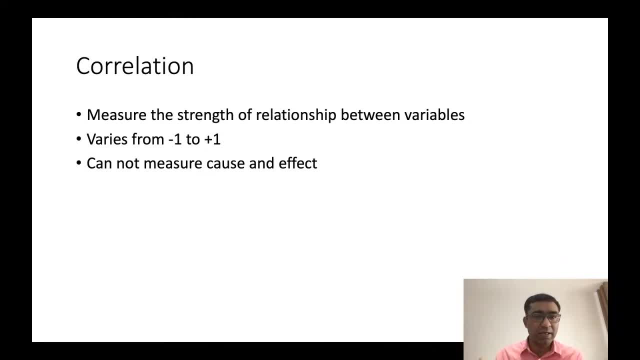 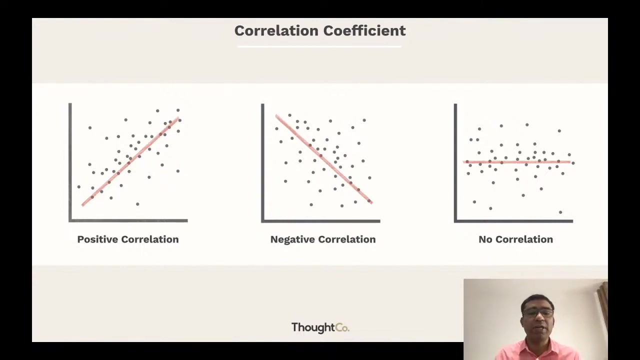 the strength of relationship. second, it only involves two variables. third, it do not have any dependent or independent variables. remember, it do not have any dependent and independent variables. okay, let's move on. let's see. this is the examples of correlations. okay, if i scattered your data, if i plot your data and i check this so you can see that there is a. 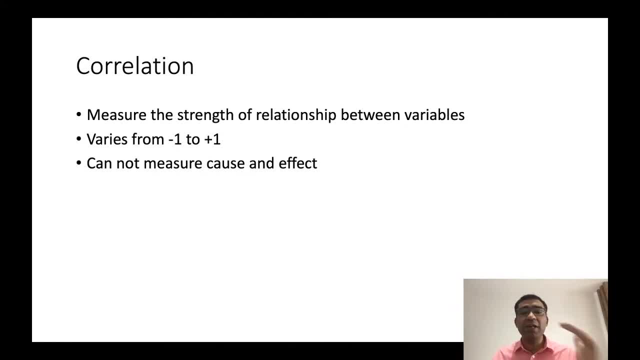 is it clear. so one value is increasing and other value is decreasing. i will show you in in in the graphical form also. but remember i mentioned two, three very important things about the correlation. first, it measures the strength of relationship. second, it only involves two variables. third, it do not have any dependent or independent. 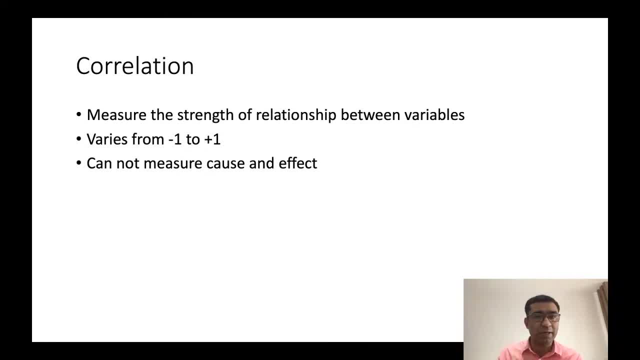 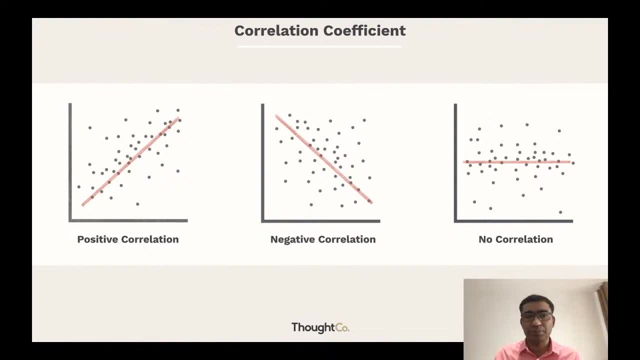 variables. remember it, do not have any dependent and independent variables. okay, let's move on. let's see, this is the examples of correlations. okay, if i scattered your data, if i plot your data and i check this so you can see that there is a trend, if i mention this one, this value, if you can see that this line is straight, 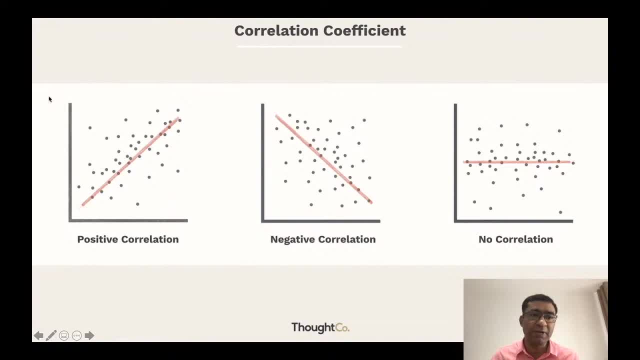 it means that this value is x and this value is y. okay, so if i write it here, so this one is x and this one is y, right? so if i explain the value of x from, for example, here i have 0 to 5, okay, and here also we have 0 to 5, for example. 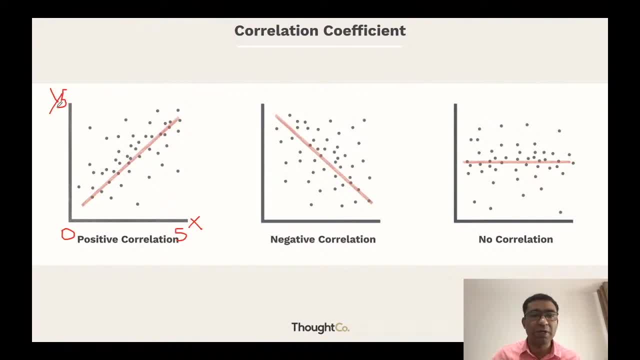 for example- I'm just giving you an example. okay, now, if I draw, here is one, here is one. so, if you can see this one. so the value of X, when the value of X is one, the value of Y is also one. so let's see, here there's a slight improvement, right, increase. so here also increase. so let let me. 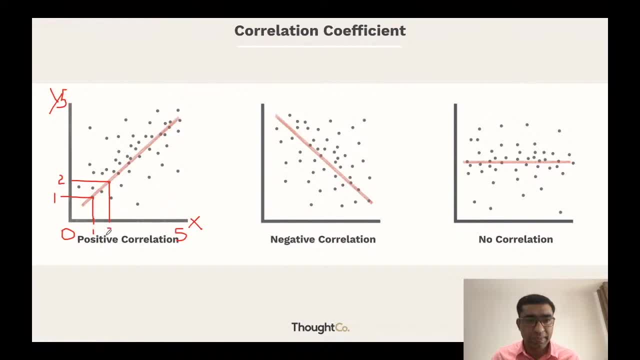 just mention this: one, two and two. so you can see that the value of X is two and same with the value of Y is also two, and you can see that all these are increasing trend increasing mean, when I say value of X is increasing from here to here, the value of Y is also increasing. okay, yeah, so this is called a. 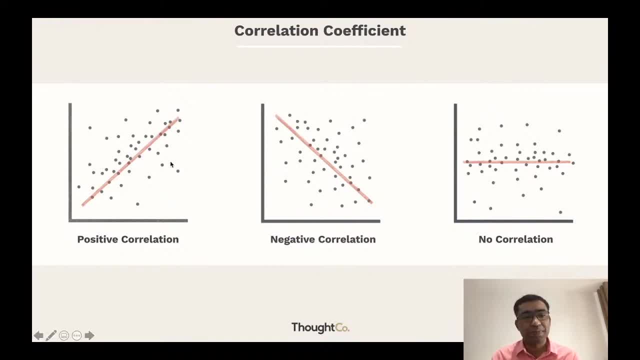 trend. if i have a linear and linear trend. that means, if i write this value, let's say this is a three-dimensional term, right, let's say: this is the model in which i also refer to this model as linear. this is the model in which i write it, so let me. 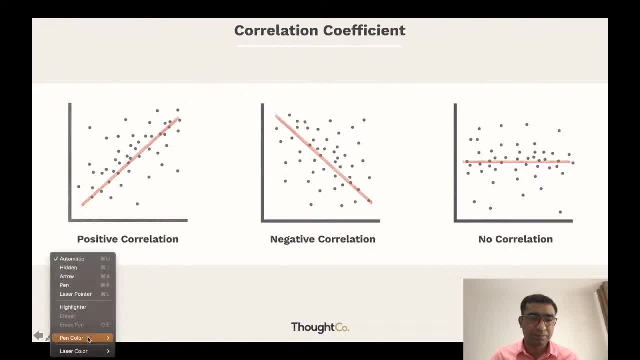 write the model in this way. let me write it this way. take the model and write it like this. okay, let me write it like this. it's going to be linear, so let me write it like this. so let's show the formula to explain the value of x here. 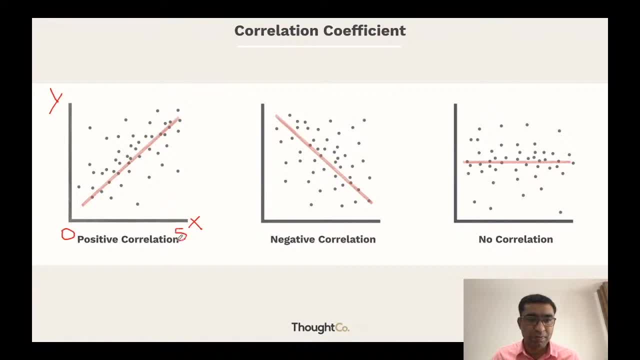 here I have 0 to 5, okay, and here also we have 0 to 5, for example. for example- I'm just giving you an example. okay, now, if I draw, here is one, here is one. so, if you can see this one, so the value of X, when the value of X is 1, the value of Y is: 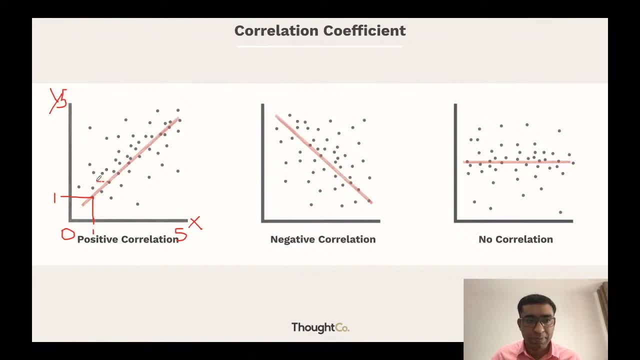 also 1. so let's see here there's a slight improvement. right increase, so here also increase. so let let me just mention this one: 2 and 2, so you can see that the value of X is 2 and same with the value of Y is also 2, and you can see that all these are. 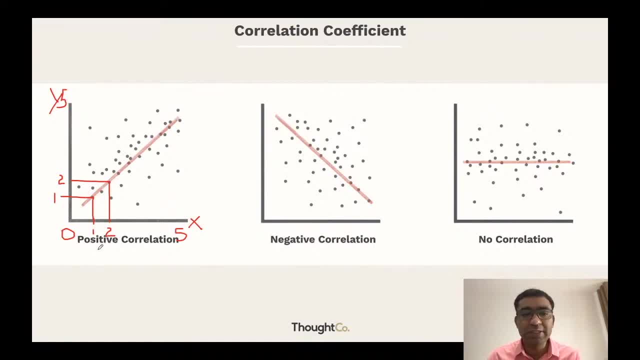 increasing trend. increasing mean when I say value of X is increasing from here to here, the value of Y is also increasing. okay, clear. so this is called a positive correlation. clear, anything, any point here, any question, you, you, okay, clear, any question. okay, let's, let's try to see this value now if I write: 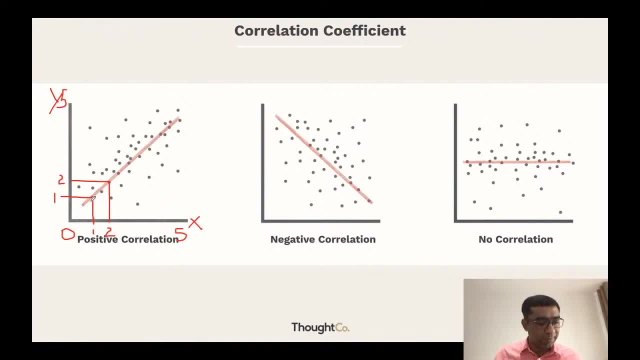 positive correlation. clear anything, any point here, any question? okay, clear, any question, okay, let's. let's try to see this value now. if I write here again X and Y and you can see that X is maximum means five when Y was one, okay, and if you see when Y is maximum, X is one. 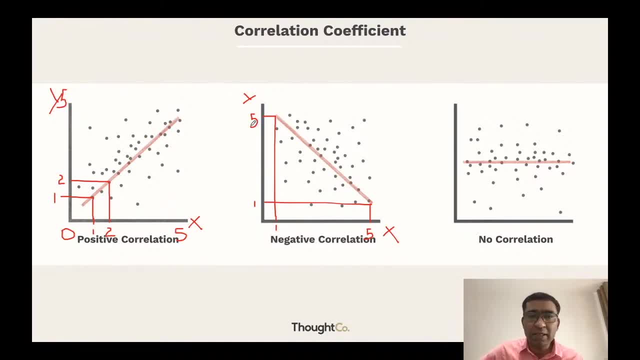 so you can see that with the increase in value of x, the value of y is decreasing. okay, the value of y is decreasing. so when x was 1, y was 5. when x is 5, y was 1. this is called a negative relationship. so this is an example of perfect positive correlation. which would be plus 1, r would be. 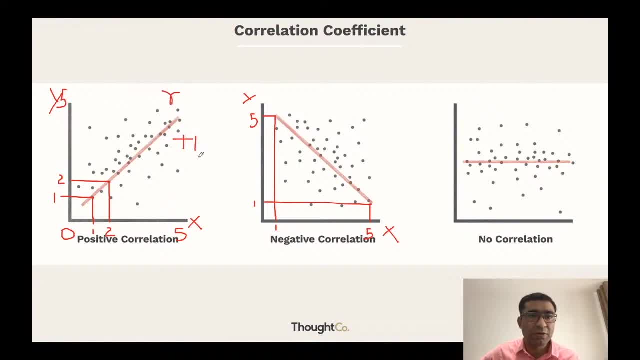 we call it correlation coefficient, which is r. so r is equal to 1 here. okay now. but here is r equal to negative 1, because it is perfectly negative correlation. okay now, this is negative 1. and here, if you see, all for all values of x, the y is same. there is no change in the value of y. so here r would be equal to. 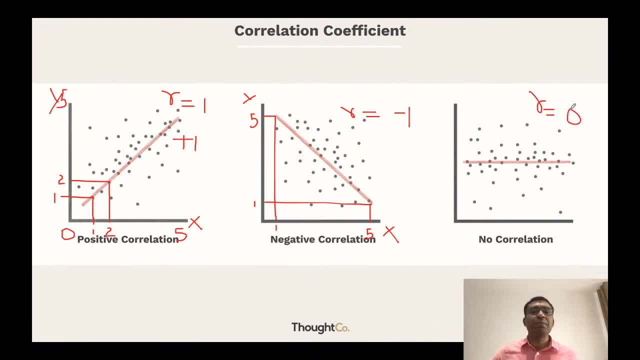 0, okay, so now here i understand. there are three possibilities: negative, positive and 0. if the negative, it means that there is a negative correlation, the value of one variable is increasing and the value of second variable is decreasing. okay, and in other case, value of one variable is. 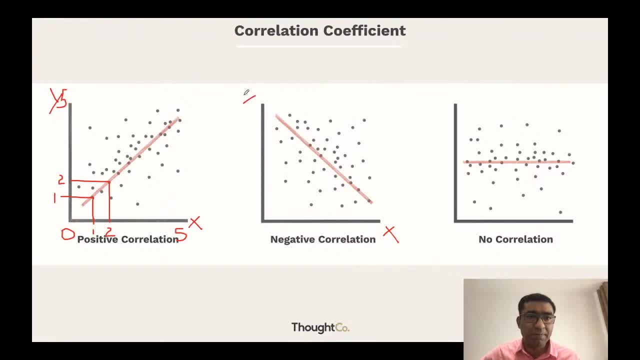 here again X and Y, and you can see that X is maximum means 5. when Y was 1. okay, and if you see when Y is maximum, X is 1. so you can see that with the increase in value of X, the value of Y is decreasing. okay, the value of Y is decreasing. so when X was 1, Y was 5. when X is 5. 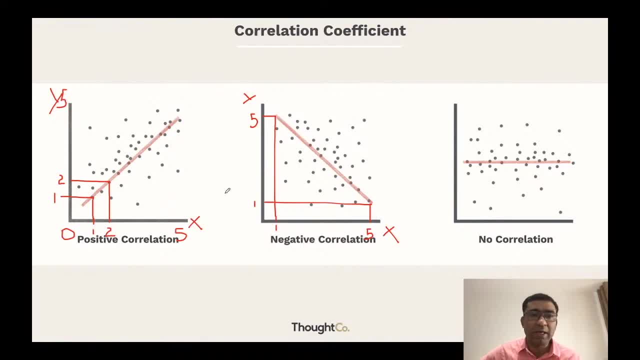 Y was 1, this is 1. is called a negative relationship. so this is an example of perfect positive correlation. which would be plus 1, r would be- we call it correlation coefficient, which is r. so r is equal to 1 here. ok now, but here is r equal to negative 1, because it is perfectly negative correlation. 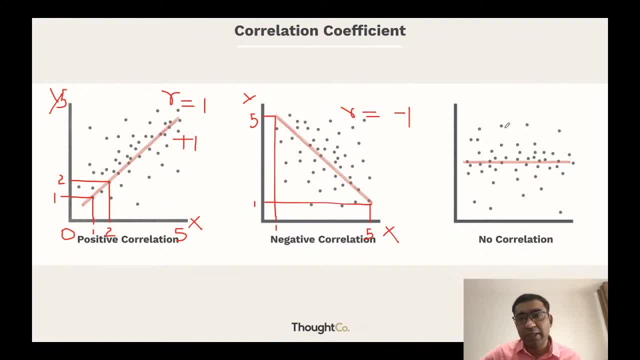 ok, now this is negative 1. and here, if you see all for all values of x, the y is same. there is no change in the value of x. So here r would be equal to 0. ok, so now here I understand. there are 3 possibilities. 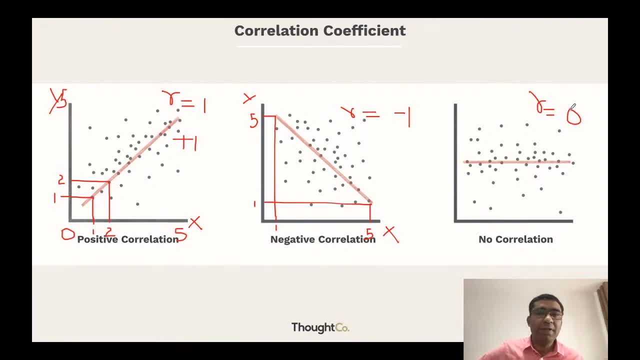 negative, positive and zero. if the negative, It means that there is a negative correlation. the value of one variable is increasing and the value of second variable is decreasing. ok, and in other case, value of 1 variable is increasing. the value of other variable is also increasing. this is positive and otherwise it is negative. 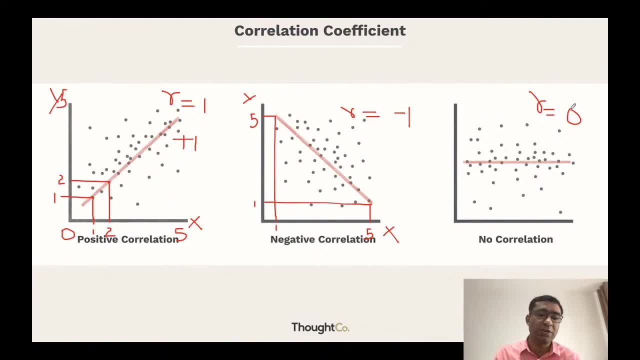 and if there is no relationship, the r is 0.. So this is simple correlation, and what we call correlation coefficient is r, So r can have positive, negative or 0.. Okay, so these three values are possible and we can explain each of them. Positive means that both variables are. 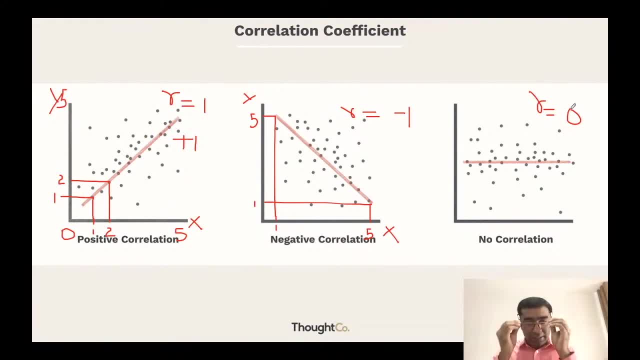 increasing and the value of other variable is also increasing. this is positive and otherwise it is negative. and if there is no relationship, the r is 0. so this is simple correlation, and what we call correlation coefficient is r. so r can have positive, positive and negative or 0. okay, so these three values are possible and we can explain each of them. 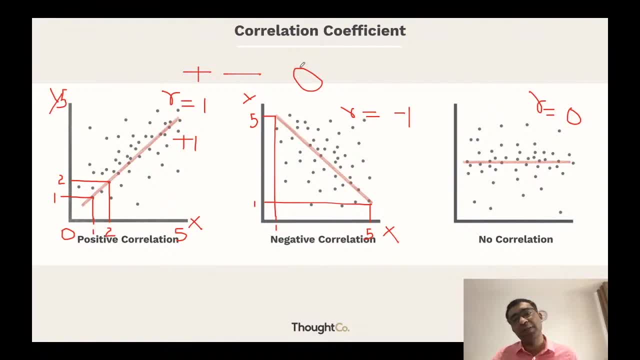 positive means that both variables are increasing. negative means that both variables are. one variable is increasing, so the other variable is decreasing. there is a negative relationship and in this, r equal to 0 means that there is no relationship. okay, clear, okay, okay, the main reason why this relationship between the relative and the ascendant is very many. 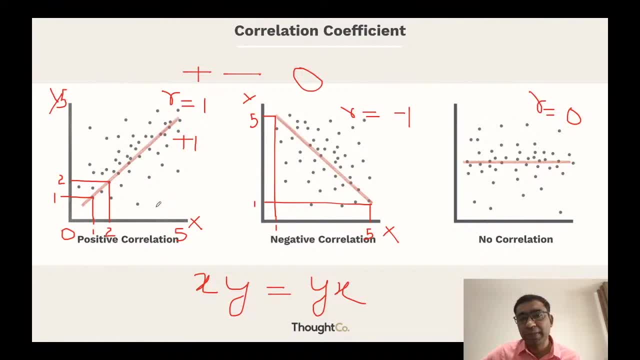 when the derivative is going and the flight is going, or when the conditionую versus the whole is different, because if there is a difference, okay, there has to be a positive relationship between them. ie this is equal to 0 or that there will be no 5, 0 will be. 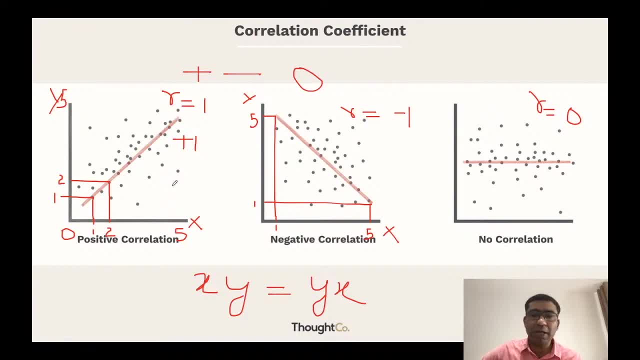 no 5, 0 or someday you will have the same relationship between relative and the, the you and to the relation that there will be. but forget to talk about the relationship 小心ly, because if we forget about the relation加油 or neuter coconut is interesting. 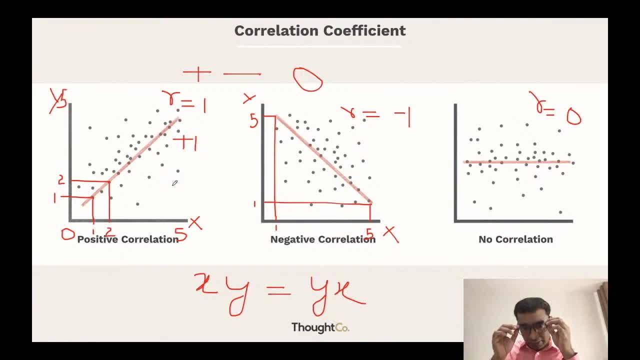 x and y, where I put x first and y later on, will be equal to y, x where I put y first and x later. okay, so this is also a simple parameter. okay, so you can understand. okay, clear, so can I consider? everybody is aware of this correlation now? 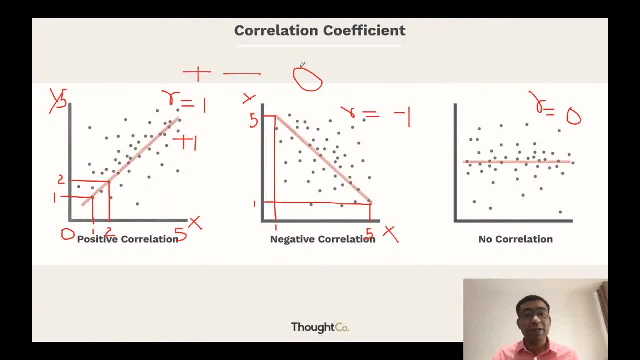 increasing. Negative means that both variables are. one variable is increasing, so the other variable is decreasing. there is a negative relationship and in this, r equal to 0 means that there is no relationship. Okay, clear. Okay, let us move to the next point. I think 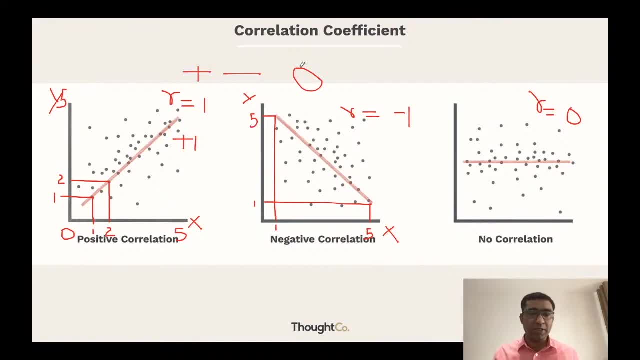 here you are clear about the r correlation coefficient. but here I am going to explain you one, One important thing: x, y is equal to y, x. This is important. This is where correlation is different than the regression. It means that if I say x to y or y to x, the value of r should: 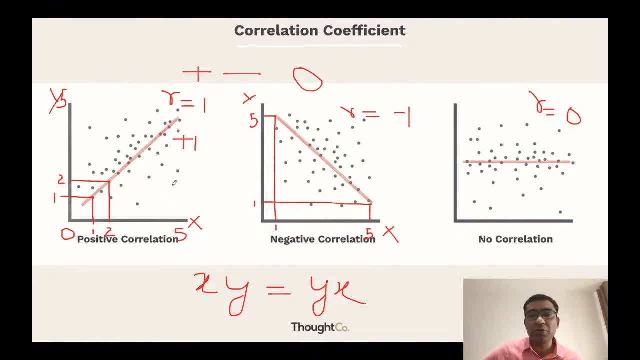 be same, There is no problem. Okay, So there is no dependent or there is no independent. Both variables behave in the same way. Okay. So if you write x and y later, so if you keep x independent, y dependent, no, no, no difference. 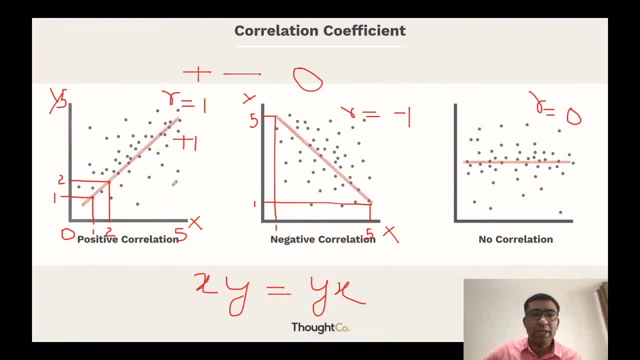 between these two. Okay, So x- y, the correlation between x and y, where I put x first and y later on, will be equal to y- x, where I put y first and x later. Okay, This is also a simple parameter. Okay, so you can understand. 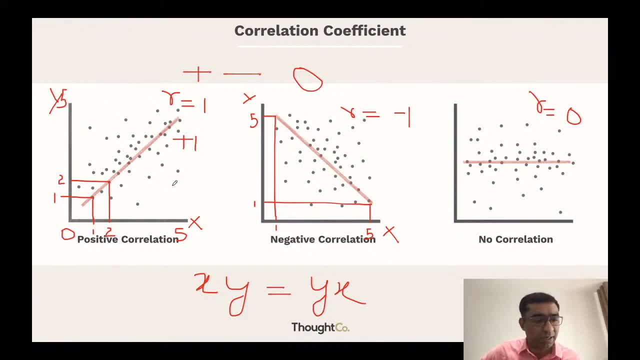 Okay, Clear. So can I consider everybody's aware of this correlation now? Yes, Can I have your reply on this? Okay, Okay, its real. Ok, okay, thanks. 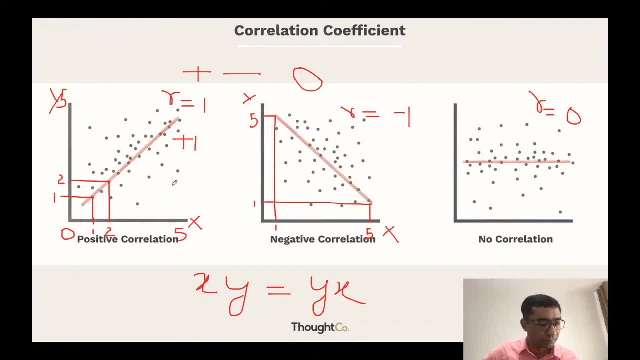 okay, can I have your reply on this? is it clear? um, can we? can we move on? ok, yes, very good question. can you give example of hypothesis statement to explain the correlation? ok, remember, when we say there is a relationship between A and B, ok, there is a relationship between A and B, for example, digital marketing and sales. so when we say 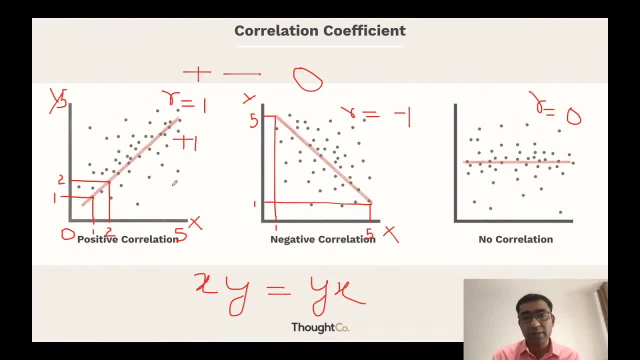 this statement. it can be a correlation if and only if- remember, if and only if- the sales and digital marketing. there is no dependent or there is no independent. ok, so in this case, both variables they work together. ok, That is why it is a correlation. So I am not talking about the dependent, I am not talking about the cause and effect. 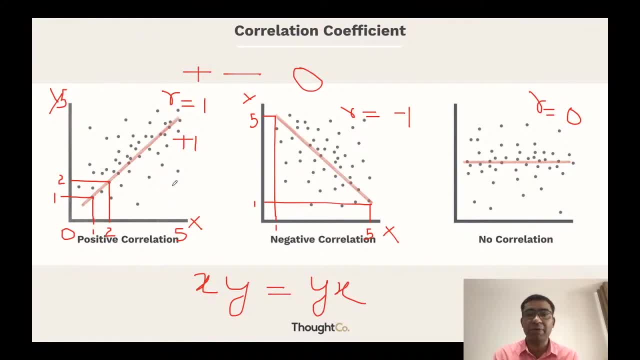 I am just talking about the relationship between variable A and variable B. ok, but in most of the cases in our research the variables nature is dependent and independent because we follow the causal relationship. I will explain in next point. but in simple word, correlation is simply the relationship between two variables. 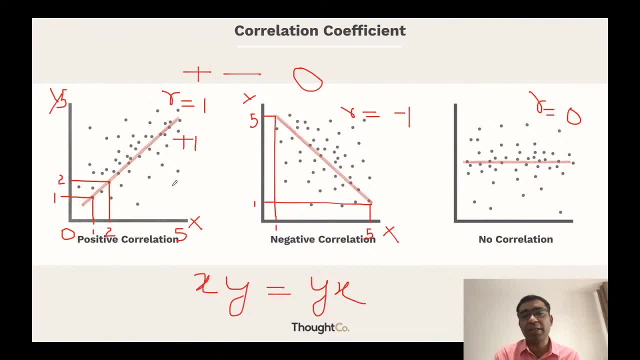 So if there any relationship between digital marketing and sales, this would be correlation hypothesis. ok, but remember one thing: don't confuse yourself with this statement, because we are looking at digital marketing as independent in our research and sales as a dependent variable. that is why correlation is not efficient, because I cannot say in this statement, if I say the 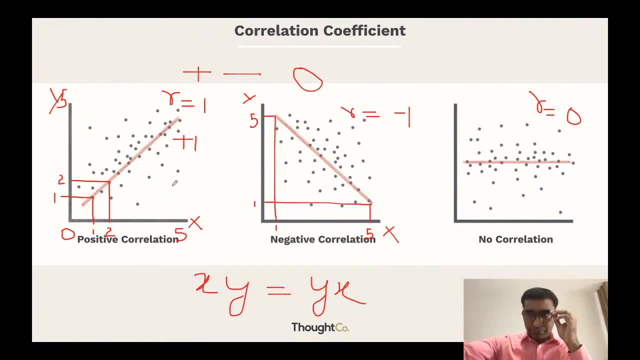 it clear, can we move on okay? yes, very good question. can you give example of hypothesis statement to explain the correlation? okay, remember, when we say there is a relationship between a and B, okay, there is a relationship between a and B, for example, digital marketing and sales. so when we say this statement, it can be a correlation up if on a if and only if. remember. 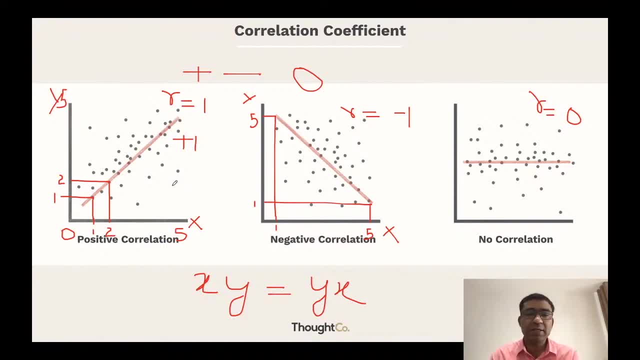 if, and only if, the sales and digital marketing. there is no dependent or there is no independent. okay, so in this case, both variables they work together, okay. that is why it is called correlation. so I am NOT talking about the dependent, I am NOT talking about the cause and effect, I am just 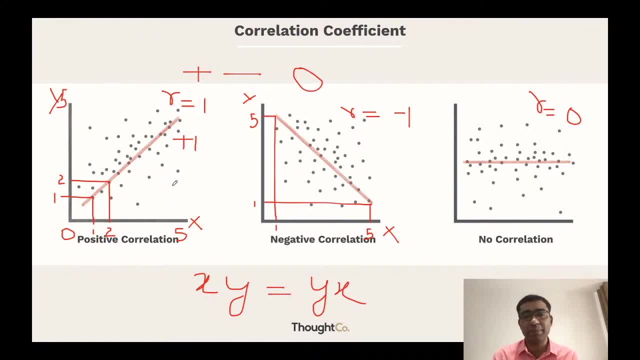 talking about the relationship between variable a and variable B. okay, but in most of the cases in our research the variables nature is dependent and independent because we follow the causal relationship. I will explain in next point. but in simple word, correlation is simply the relationship between two variables. so if there any relationship between digital marketing and sales, this would 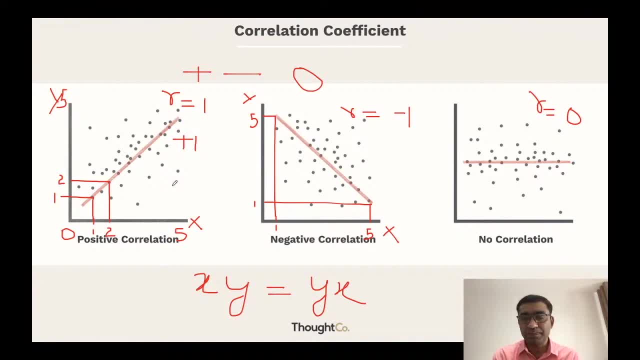 be correlation hypothesis, okay, but remember one thing: don't confuse yourself with this statement, because we are looking at digital marketing as independent in our research and sales as a dependent variable. that is why correlation is not efficient, because I cannot say in this statement, if I say the correlation, 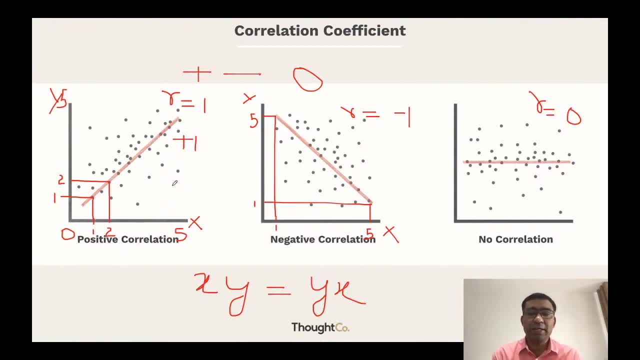 the, the digital marketing, and there is a relationship between digital marketing and sales. it means that when the sales increase, digital marketing increases. when the digital marketing increases, the sales should be increased. so you should be clarified on your relationship here. it is a problem. we can say that when digital 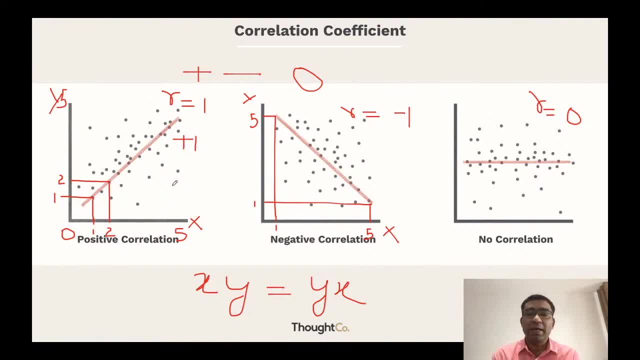 correlation, The digital marketing and there is a relationship between digital marketing and sales. it means that when the sales increase, digital marketing increases. when the digital marketing increases, the sales should be increased. so you should be clarify on your relationship here. it is a problem. we can say that when digital marketing increases, the sales increase. I agree with. 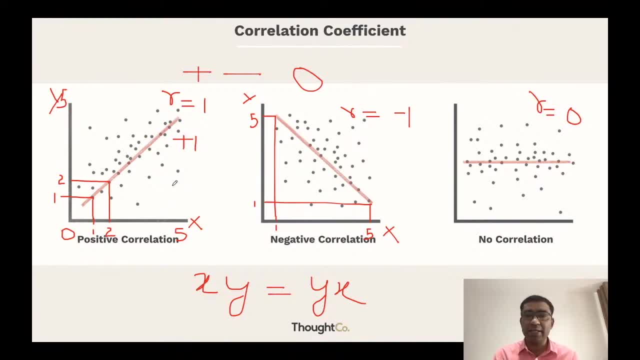 this statement. But when I say when the sales increases, digital marketing increases, this is something we we are not clear about. I don't think so. that is the case. in that case, this property, if you remember, this property- is not holding ok, so means that sales and digital marketing. 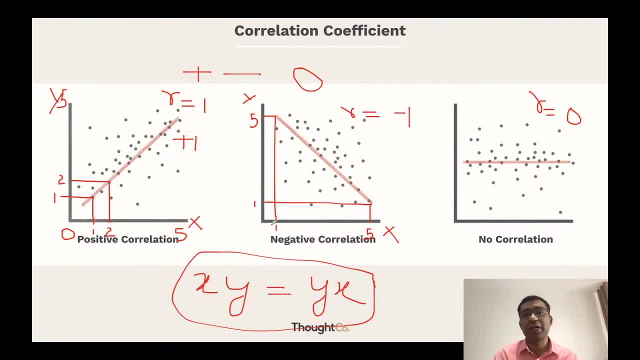 digital marketing and sales, so both are not same. so that is why we use regression, because this is a problem. ok, Ok, clear. yes, the positive value of the graph- it is like this, increasing and the negative value is decreasing. ok, clear, ok. so is this clear about the correlation? what is the hypothesis? 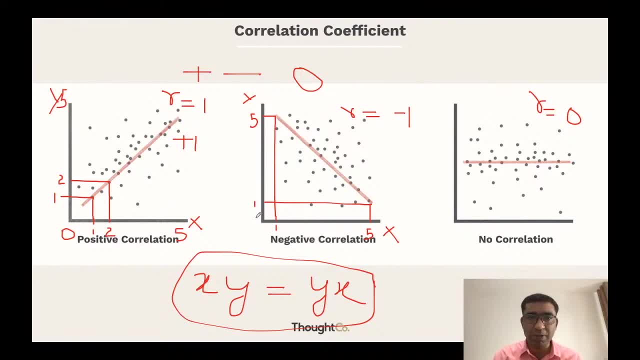 for correlation. the correlation is basically just simple relationship between two values. ok, If, for example- Ok, I want to see, is there any correlation between the death rate and sales, or, sorry, ice cream sales, for example, anything death rate or and covid. ok, so we should understand whether our 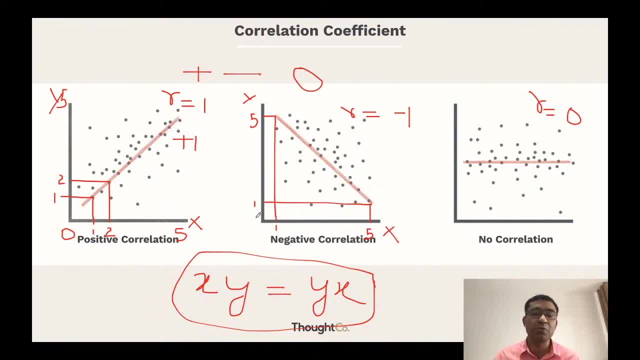 relationship is causal in nature or it is two way. ok, when the relationship is two way, we can use correlation, but when the relationship is one way, we call it causal relationship. in that case, correlation- Correlation is not significant or not sufficient to reply or answer you. reply your question. 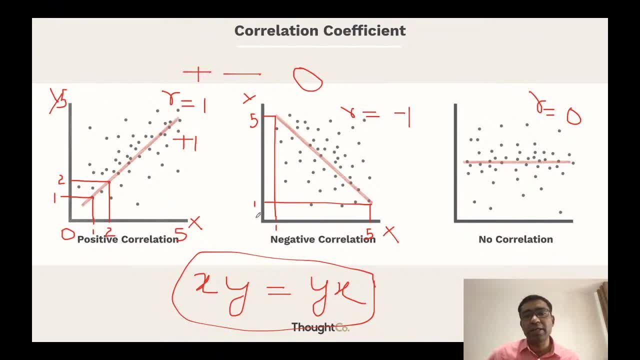 ok, clear. so correlation is just a relationship between A and B. ok, this, this, the correlation, can be a very good example in a love story. ok, a person A loves person B and person B loves person A, So both, no matter if we keep person A or person B. 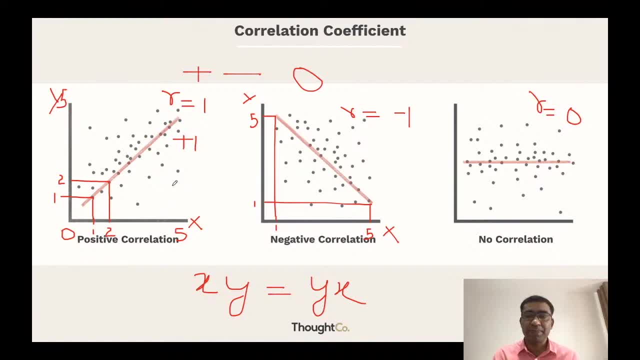 marketing increases, the sales increase. I agree with this statement, but when I say, when the sales increases, digital marketing increases, this is something we we are not clear about. I don't think so. that is the case. in that case, this property, if you remember, this property- is not. 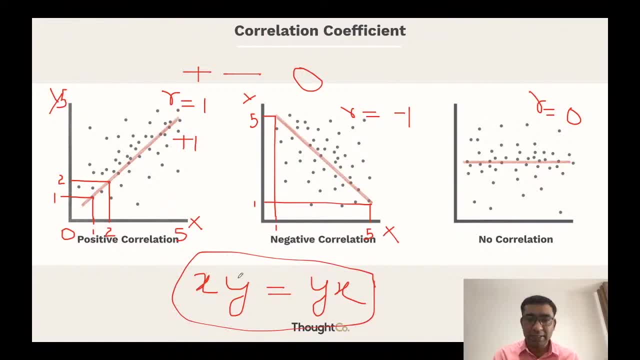 holding okay, so means that sales and digital marketing, digital marketing and sales, so both are not same. so that is why we use regression, because this is a problem. okay, okay, clear. yes, the positive value of the graph- it is like this, increasing and the negative value is decreasing. 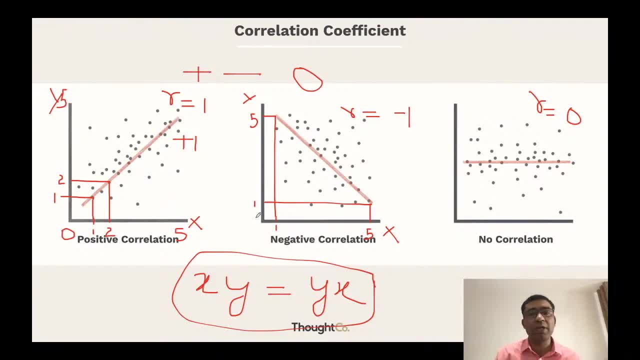 okay, clear, okay. so is this clear about the correlation? what is the hypothesis for correlation? the correlation is basically just simple relationship between two values. okay, if, for example, I want to see: is there any correlation between the death rate and sales, or, sorry, ice cream sales, for example, anything, death rate or and. 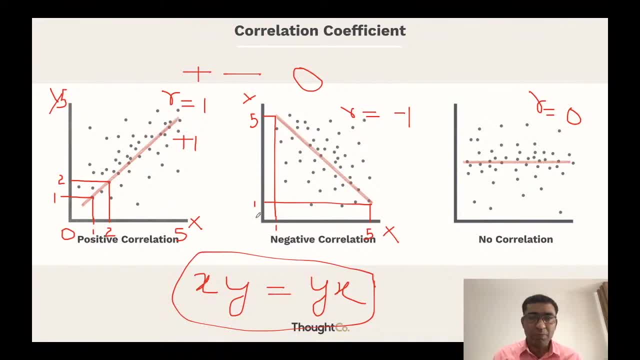 covet. okay. so we should understand whether our relationship is causal in nature or it is two-way. okay, when the relationship is two-way, we can use correlation, but when the relationship is one way, we call it causal relationship. in that case correlation is not significant or not sufficient to reply or answer. you. reply your question, okay, clear. so 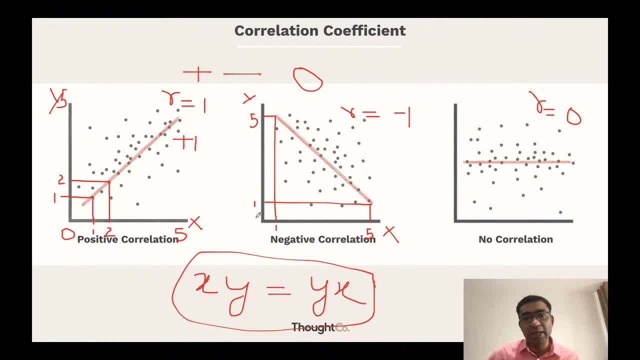 correlation is just a relationship between a and b. okay, this, this, the correlation, can be a very good example in a love story. okay, a person a loves person b and person b love person a, so both. no matter if we keep person a or person b, so both are loving. 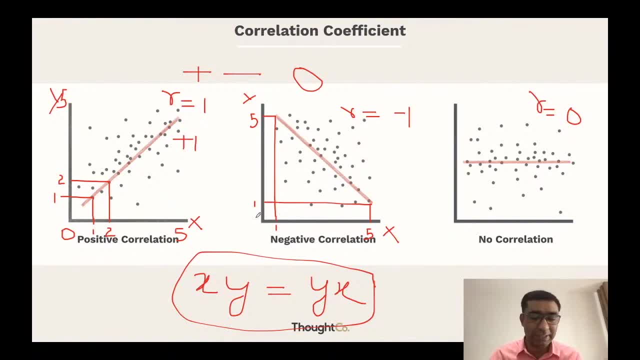 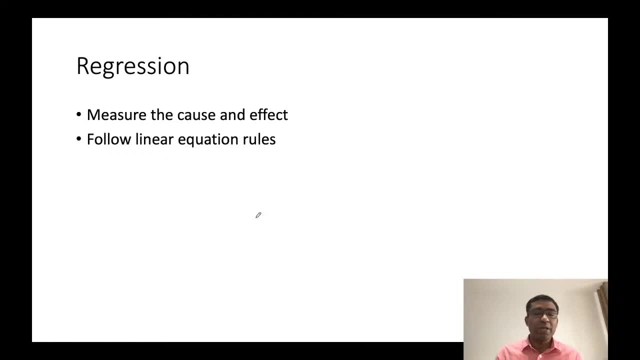 so in that case, it can be an example of correlation. let's move on to the next point: regression. now, this is important. we need to understand where the correlation have some limitations. do you understand? correlation have some limitation, but it will not give you cause and effect. now, when we say digital marketing has an influence on sales, digital marketing has an. 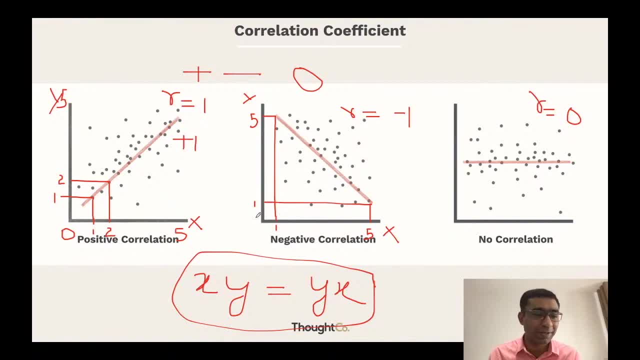 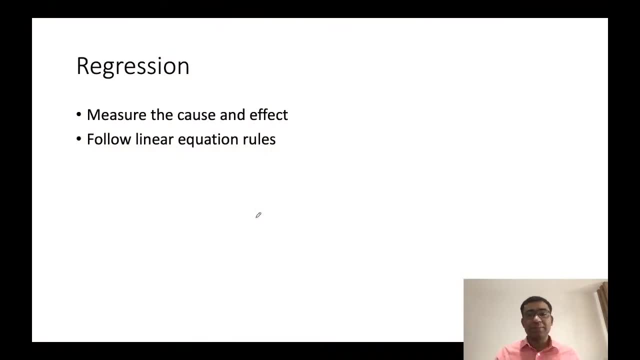 Ok, Ok, Ok, Ok, Ok, ok. So in that case, it can be an example of correlation. let's move on to the next point: regression. now, this is important. we need to understand where the correlation have some limitations. do you understand? correlation have some limitation, but it will not give you cause and effect. 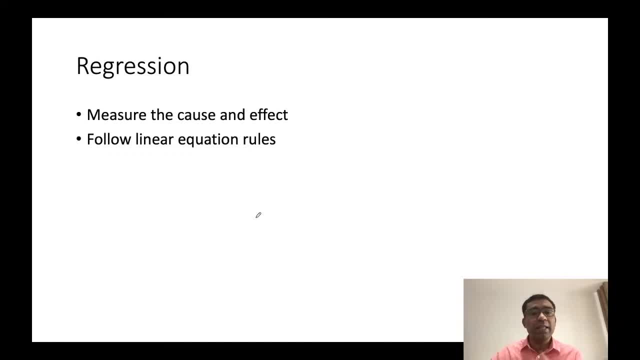 now, when we say digital marketing has an influence on sales, digital marketing has an impact on sales. marketing has a positive effect on sales. now I am using this word effect, influence, impact. okay, remember, these words are different. this word shows a causal relationship, not two-way relationship. remember, digital marketing has a 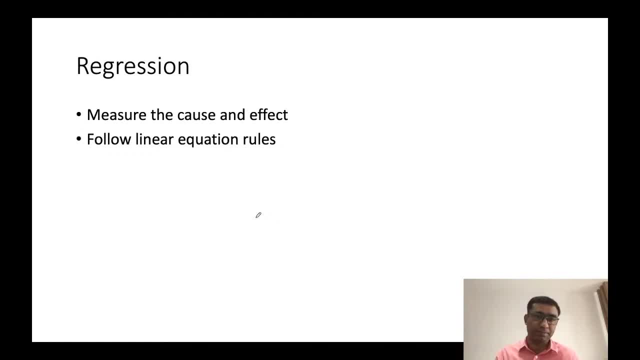 positive impact on sales. digital marketing has a positive relationship with the sales. when we say relationship, it's a simple relationship and it can be two-way, but we are just explaining one side of the relationship. that is why it is called a cause-and-effect relationship. okay when we say okay. 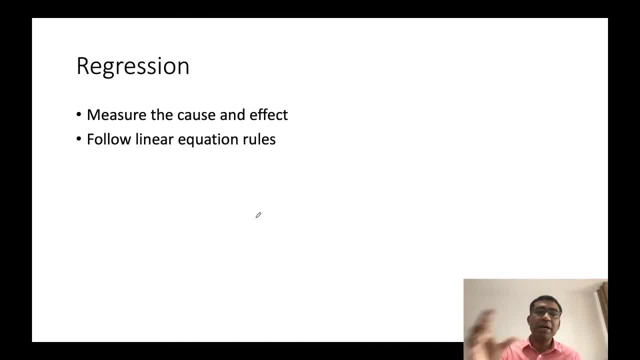 digital marketing has an influence on sale. digital marketing has an effect on sales. so all these are basically cause-and-effect types of the relationship. in such cases we have to use regression, not the correlation. okay, so regression is different, correlation is entirely different. so usually we don't use correlation to accept or reject the. 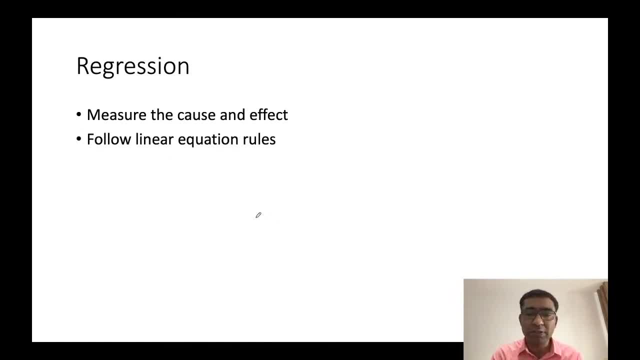 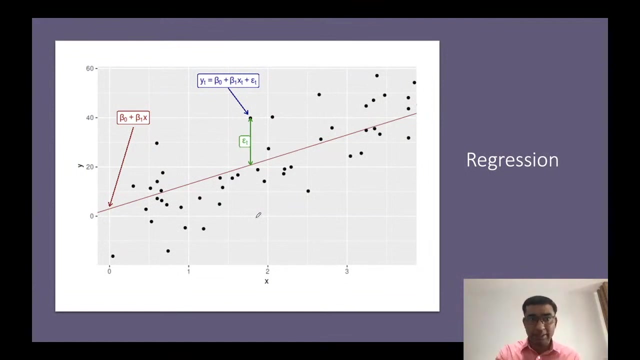 hypothesis, if our hypothesis are causal in nature. okay, so first thing. the second thing: regression is just like a linear equation. it follow the linear equation, okay, and I will explain in a while how it is different than correlation and what is actually regression is. so let's see, this is regression. okay, you can see this equation. it is same like. 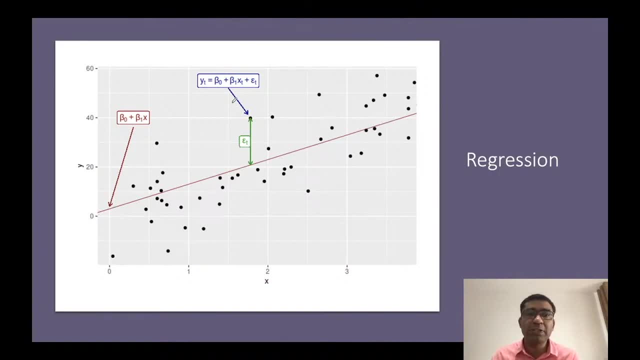 your correlation, but it follow this equation. okay, so this equation is very, very important. now let me try to explain these concepts. each one of them should be very important and you have to understand. okay, so why is your dependent variable? okay, so, why is your dependent variable? okay? 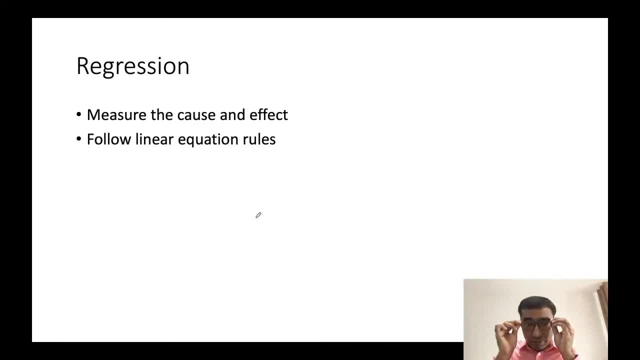 impact on sales. digital marketing has a positive effect on sales. now i'm using this word effect, influence, impact, okay, remember, these words are different. this word shows a causal relationship. okay, not two-way relationship. remember. digital marketing has a positive impact on sales. digital marketing has a positive relationship with the sales. when we say relationship, it's a 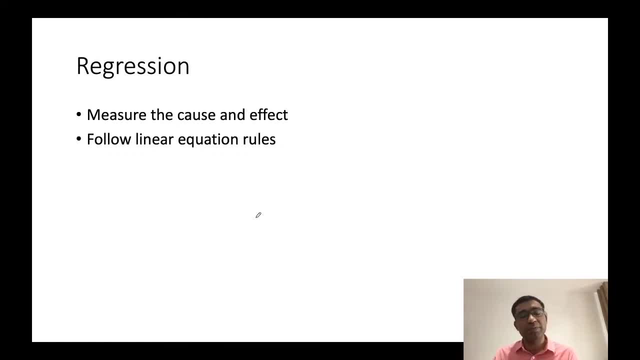 simple relationship and it can be two-way, but we are just explaining one side of the relationship. that is why it is called a cause and effect relationship. okay, when we say, okay, digital marketing has an influence on sales, digital marketing has an effect on sales. so all these are basically cause and effect types of. 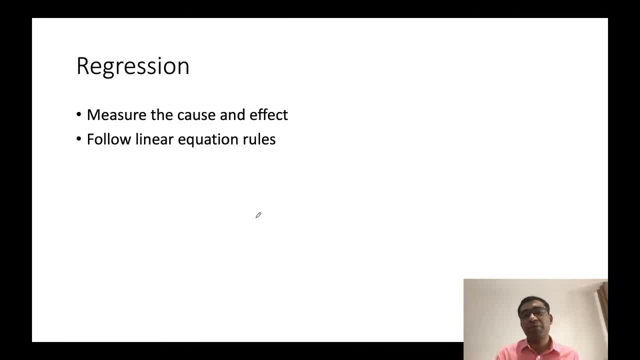 the relationship. in such cases we have to use regression, not the correlation. okay, so regression is different, correlation is entirely different. so usually we don't use correlation to accept or reject the hypothesis if our hypothesis are causal in nature, okay. so first thing. the second thing is: regression is just like a linear equation. it follow the linear equation. okay, and i will explain. 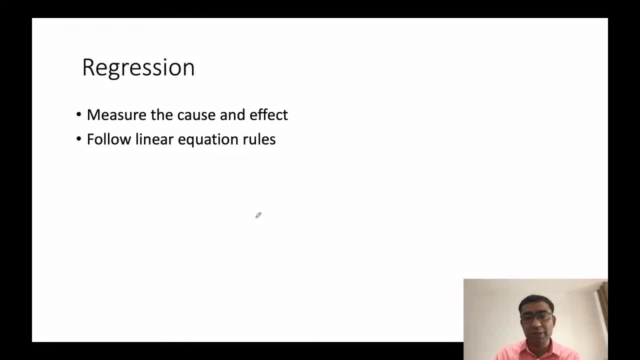 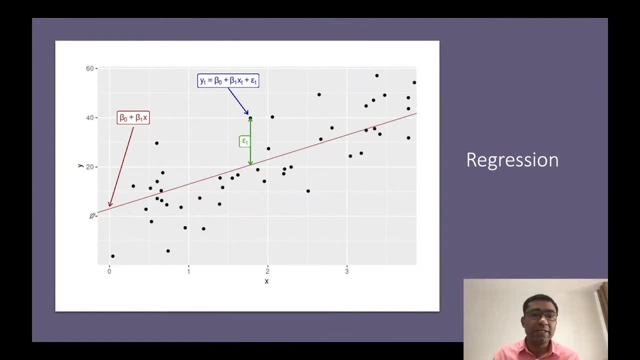 in a while how it is different than correlation and what is actually regression is. so let's see, this is regression. okay, you can see this equation. it is same like your correlation, but it follow this equation. okay, so this equation is very, very important. now let me try to explain the correlation. 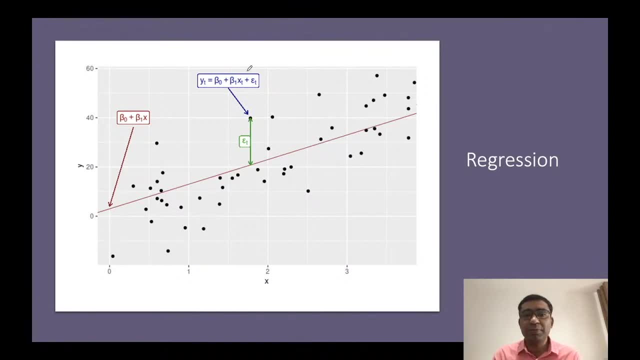 so let me try to solve it. so let theهم pass. i will test the internationally by manually. so let me test the internationally by manually. okay, you can see at Coach OP中共. now let me show you. you can see, we have to solve it. how to solve the correlation. so the question: 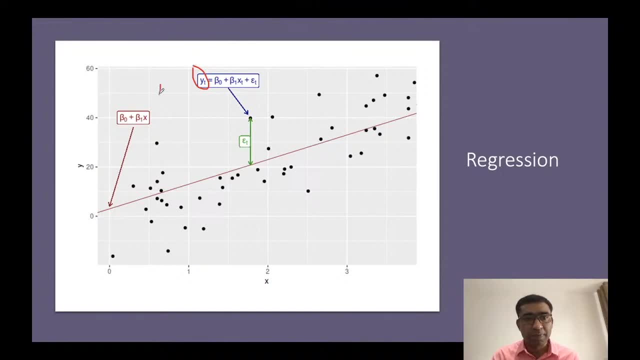 problem, okay, guys, is to come back to the situation. let me just conclude the Parcel points and the causative performance it will show, and then will be the next step, statically. so, basically, the relationship between the roughly, where we are talking about the correlation okay, and r? r is just minus and plus, so we cannot determine the exact location of that line. 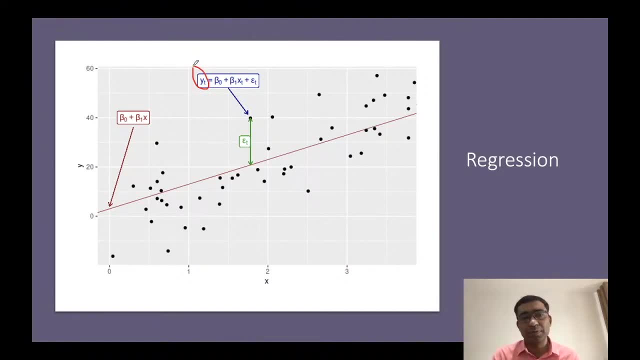 so why is your dependent variable okay? so this is, for example, in our case, sales. now this is b1 in the regression, in the correlation, it gives us only R. R is just minus and plus. so we cannot determine the exact location of that line. we cannot predict. we can just see the strength of relationship. it tells us that. 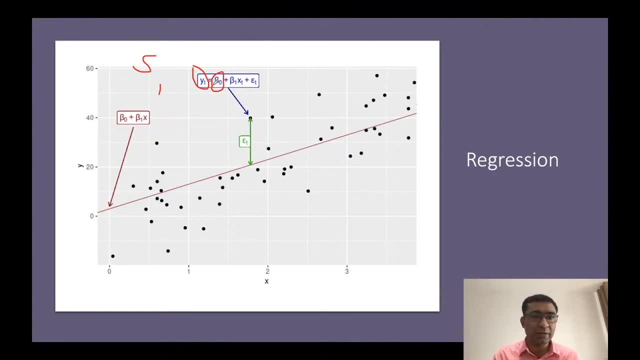 strength of relationship, not exactly the nature, okay. so why the nature is not there? this is beta naught, beta naught, or. sometime we call it alpha. okay, so this one is basically this y-intercept constant. okay. sometime we call it a constant. okay, so this is constant. now the question is this: in the correlation, 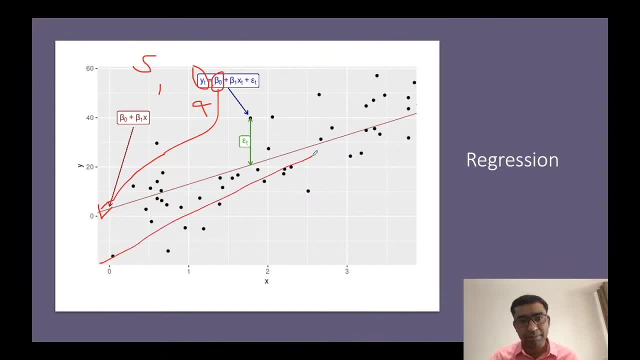 the line was started from the beginning of the correlation and the line was started from here technically. but you see, here in regression, the line is starting from a different point. okay, now, from where this line intercept the y-axis is called your beta. okay, beta naught. beta 0 or constant: okay, we call it C constant. okay, clear. so. 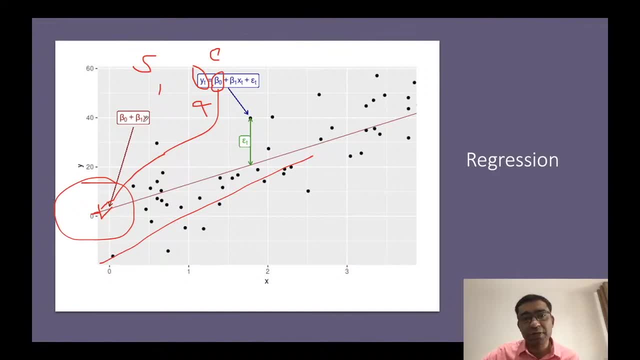 here it's different than correlation. so first value: beta 1 is telling us that, the line is telling us beta naught is telling us this value, or we call it constant, okay, constant, remember. sorry for this amazing writing, but first my writing is like this, and the second: 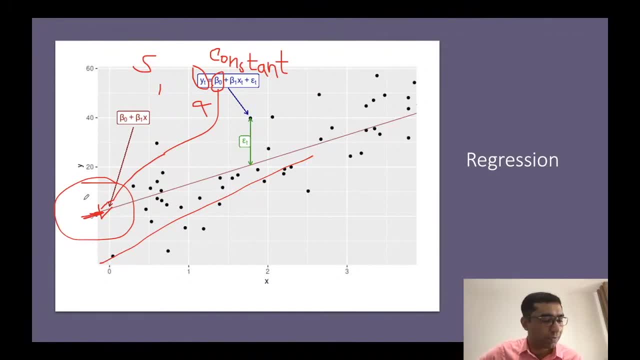 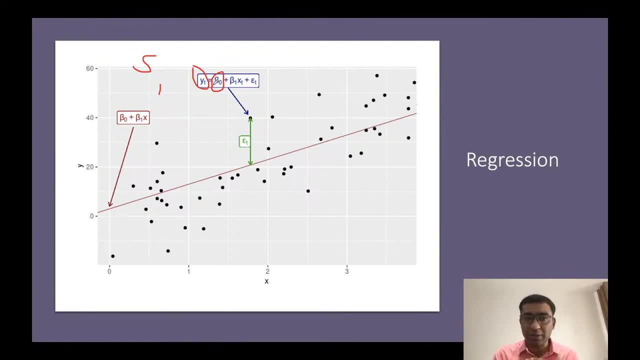 we cannot predict. we can just see the strength of relationship. it tells us strength of relationship, not exactly the nature, okay, so why the nature is not there? this is beta naught, beta naught, or sometime we call it alpha. okay, so this one is basically this: y intercept. 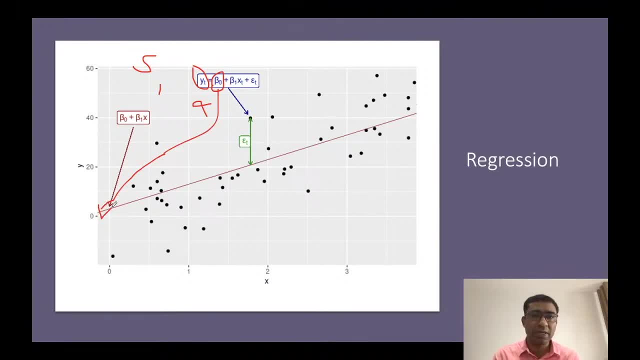 constant, okay, sometime we call it a constant okay. so this is constant. now the question is this: in the correlation the line was started from here technically, but you see, here in regression the line is starting from a different point. okay, okay, okay, okay. now, from where this line intercept the y axis is called your beta, okay, beta, naught beta. 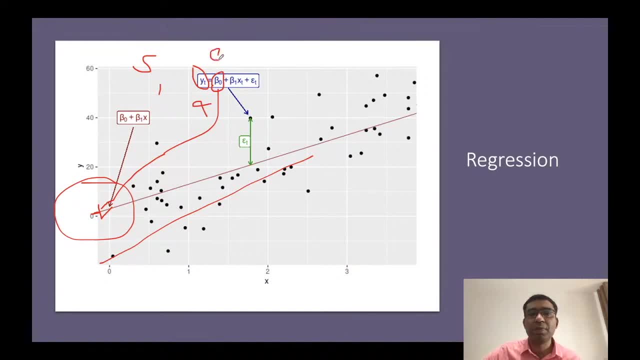 zero or constant, okay, we call it c constant, okay, clear. so here it's different than correlation. so, first value: beta 1 is telling us, beta naught is telling us this value, or we call it constant, okay, constant, remember. okay. sorry for this amazing writing, but uh, first my writing is like this and the second one is: i'm 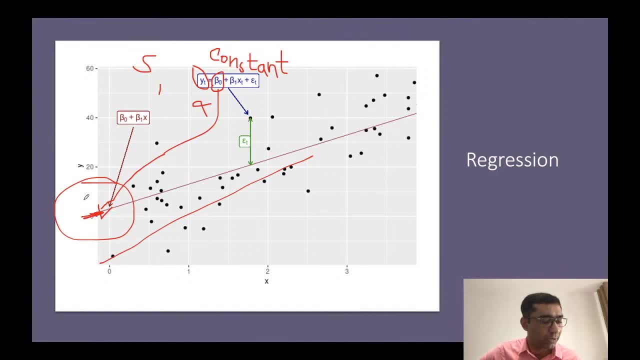 using mouse pad. that's why it's difficult for me to write. okay, now, this value is constant, okay, so constant means that this value is constant, okay, so constant means that this value is constant, okay. okay mean from where this line is going to touch the y axis. okay, so this is constant. 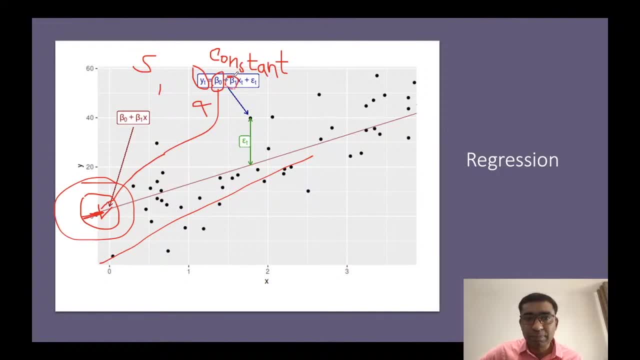 okay, now this one is beta one. beta one is we also called slope or we call it, for example, we call it how much this line is inclined. you know, here it, this line can be like this, this line can be like this, this line can have a lot of options, even starting from this point. 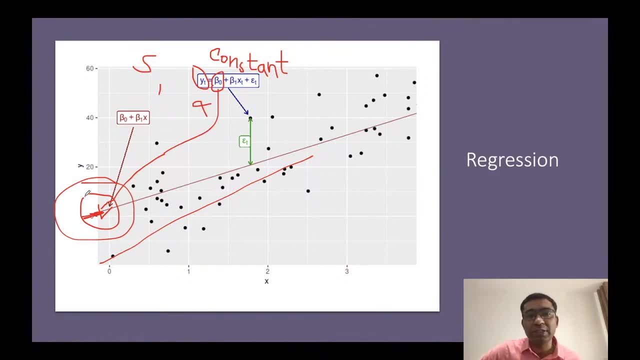 constant mean from where this line is going to touch the y-axis. okay, so this is constant. okay, now this one is beta 1. beta 1 is we also called slope or we call it. for example, we call it how much this line is inclined. you know, here it, this line. 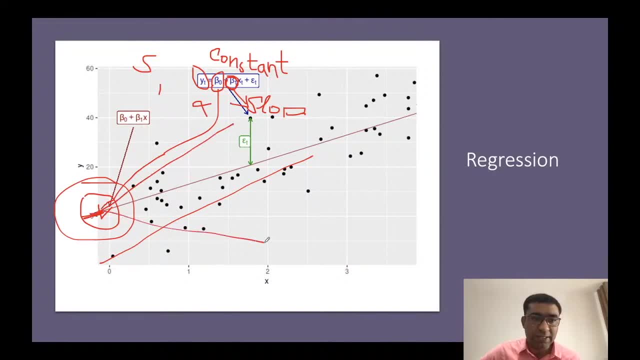 can be like this. this line can be like this. this line can have a lot of options, even starting from this point, but this line can have multiple options, okay. so these options means that how much this line is inclined with the x-axis is called your beta naught, and also, in simple world, it tells us the strength of relationship. 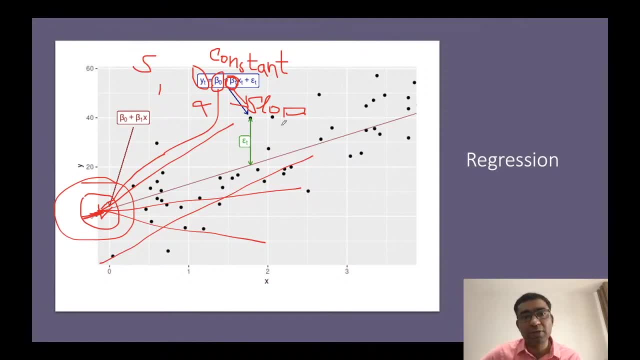 ok, I will explain it a bit later more in detail. ok, so are you clear about this point? so beta 1 is basically the your inclination of this line. okay, so inclination of this line with the x axis. ok, now here we have another term. this is called e. e is your error term. ok, so this. 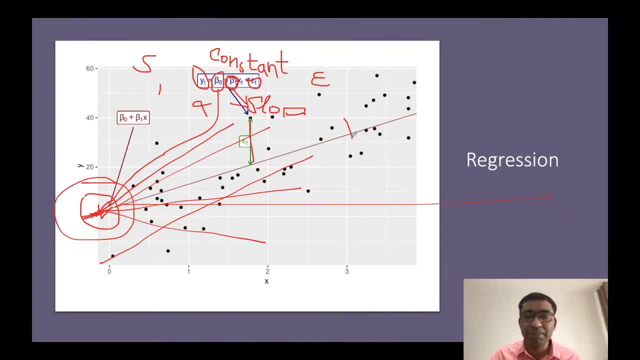 is the error, because this is the predicted line and this is your actual data. so the difference between actual data and predicted line is called error. or we also call it standard deviation- st ok, so we have a sorry residue, not standard deviation, we call it residue, so this is called a error term. 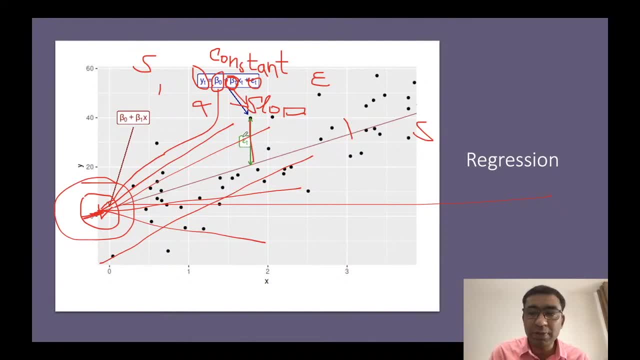 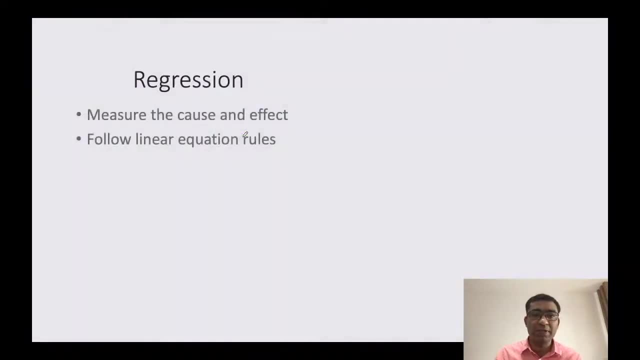 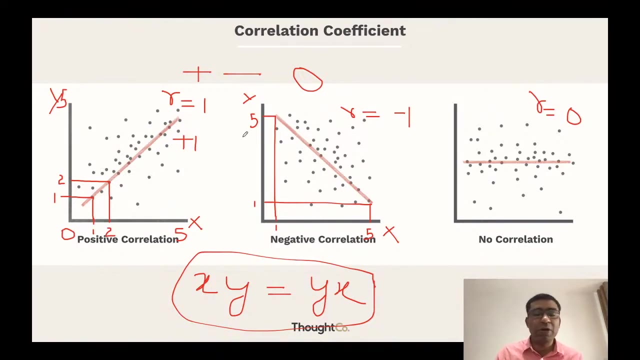 ok, error residue. so we we use these terms in the regression. now you can see that the regression is more comprehensive and in the correlation we have just one or two thing. for example, here in the correlation we have just our value. there is no error, there is no XY intercept, there is nothing. 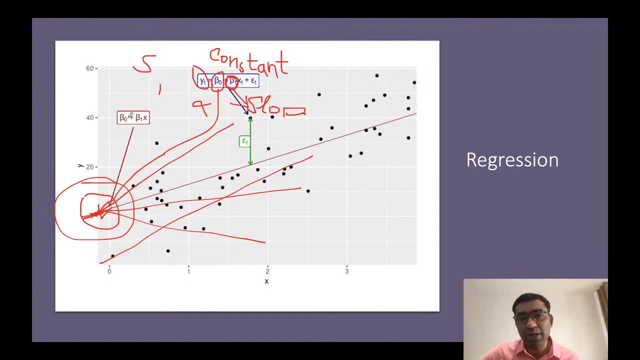 but this line can have multiple options, okay. so these options mean that how much this line is inclined with the x-axis is called your beta naught and also, in simple word, it tells us the strength of relationship. okay, i will explain it a bit later more in detail. okay, so are you clear? 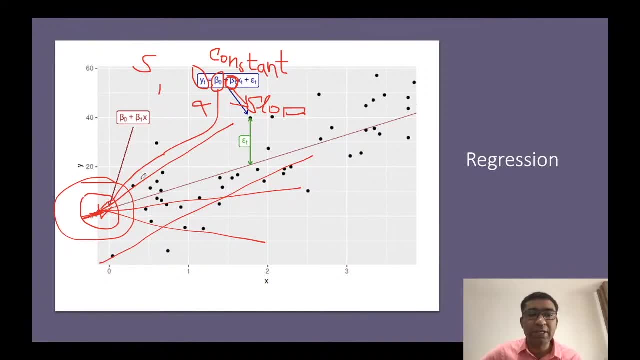 about this point. so beta 1 is basically the your inclination of this line. okay, so inclination of this line with the x-axis. okay, now here we have an another term. this is called e. e is your error term. okay, so this is the error, because this is. 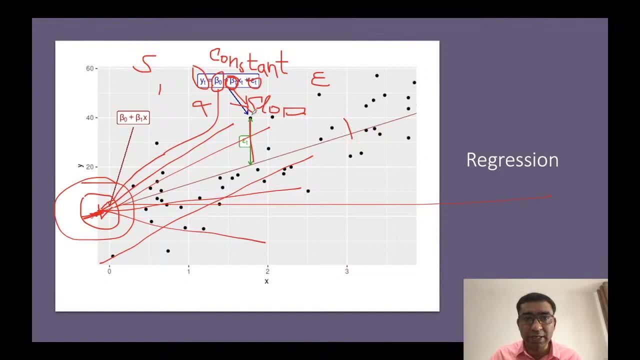 the predicted line and this is your actual data. so the difference between actual data and predicted line is called error, or we also call it standard deviation- st. okay, so we have a sorry residue, not standard deviation, we call it residue. so this is called a error term. okay, error residue. so we 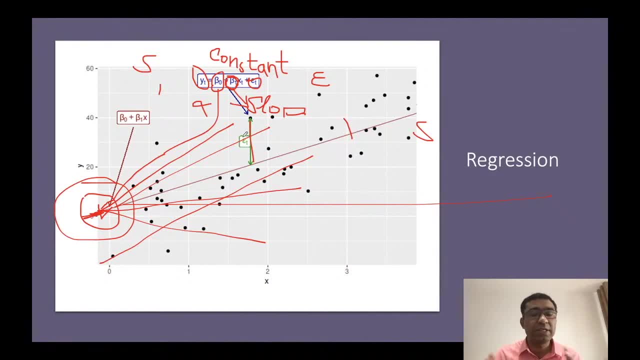 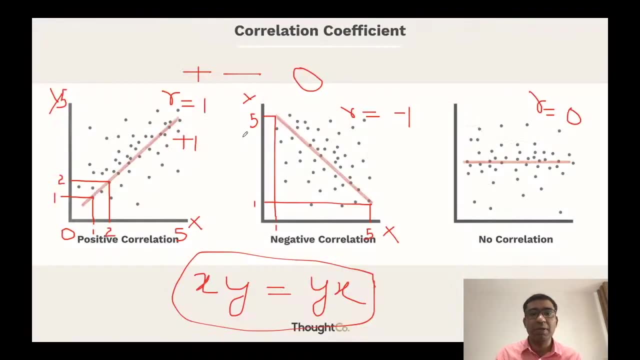 use these terms in the regression. now you can see that the regression is more comprehensive and in the correlation we have just one or two thing. for example, here in the correlation we have just our value. there is no error, there is no x, y, intercept. there is nothing, it's just tell us the strength. 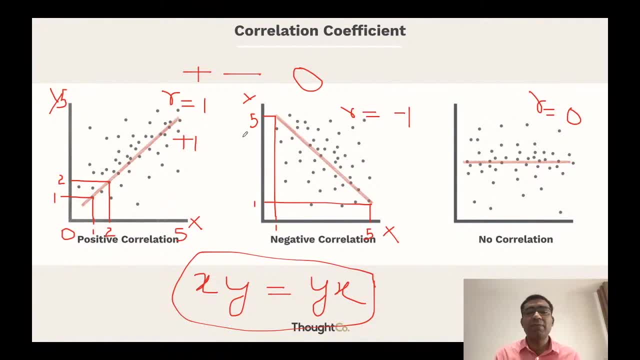 of relationship. okay, in simple word, it will tell me if i increase one unit of x, how many units of units of y will be increased. this is simple: R. ok, let me tell you again. it is very important. you should write this with your notebooks. ok, now, in this simple correlation tells us: 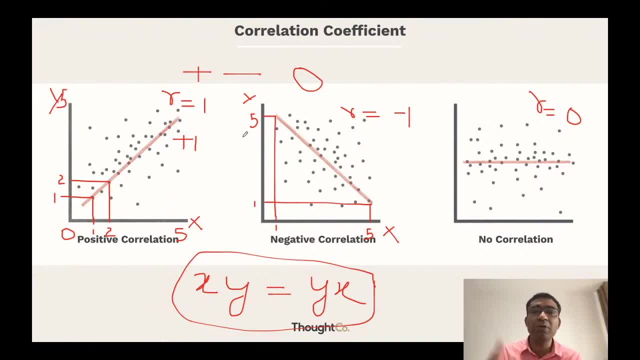 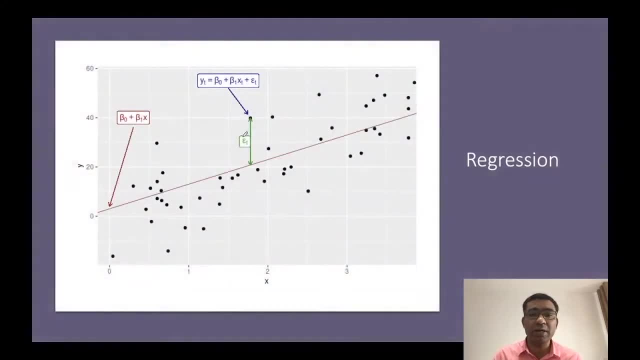 if I increase one unit of x, how many units of y will be increased? ok, so this is called correlation coefficient, but in the regression we are not just concerned with one. what I say is one value. we are concerned with the. where this line is going to be start, how much? 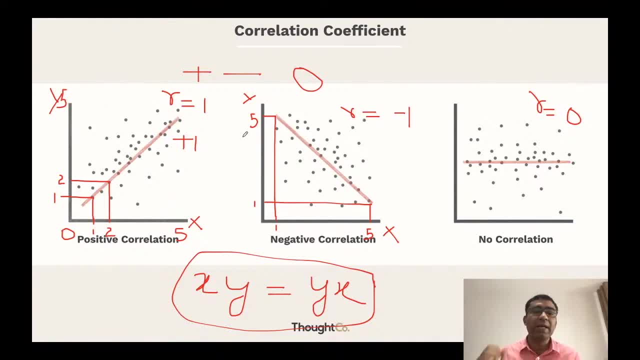 it's just telling us the strength of relationship. ok, in simple words, it will tell me, if I increase one unit of X, how many units of y will be increased. this is simple, are? ok, let me tell you again. it is very important. you, you should write this with your notebooks. ok, now, in this simple correlation, 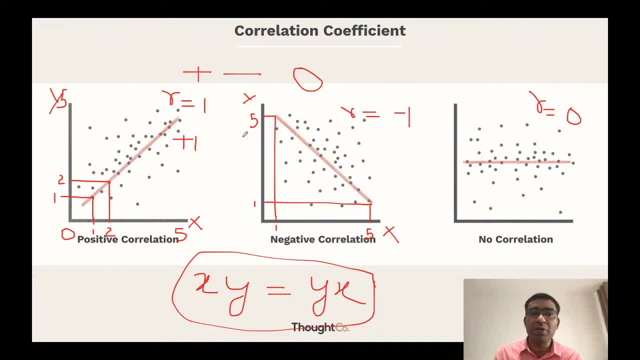 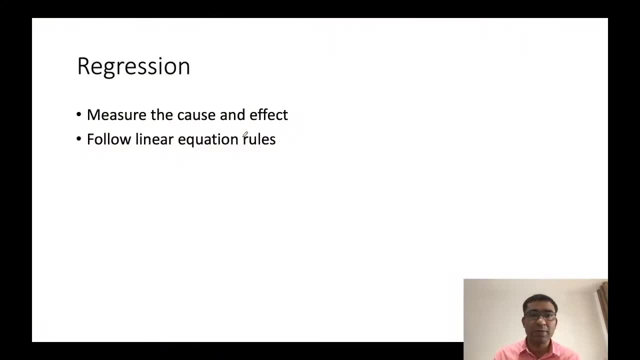 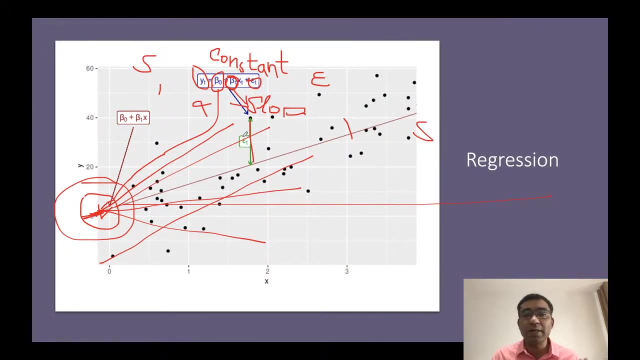 tells us, if I increase one unit of X, how many units of Y will be increased. okay, so this is called correlation coefficient. but in the regression we are not just concerned with one. what I say is one value. we are concerned with the where this line is going to be start, how much this line is inclined with the x-axis. so 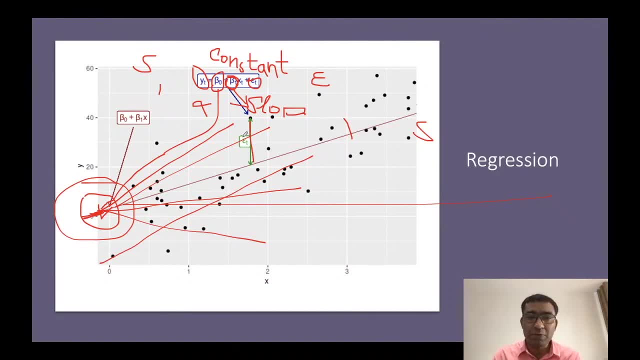 we can predict our values very clearly. okay, so this is how simple, okay, clear. okay, if it is clear, is there any question? okay, if it is clear, is there any question? okay, if it is clear, is there any question you want to ask? to the next step: we are going to use SPSS now to do all this in. 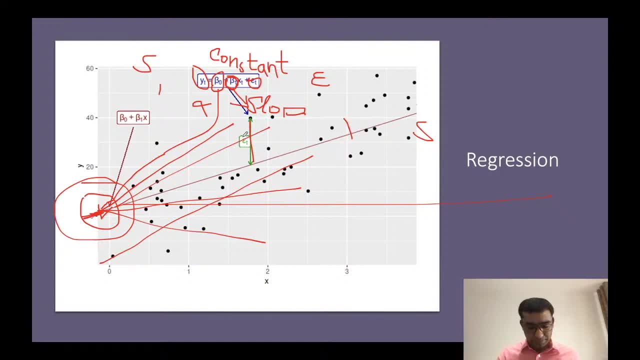 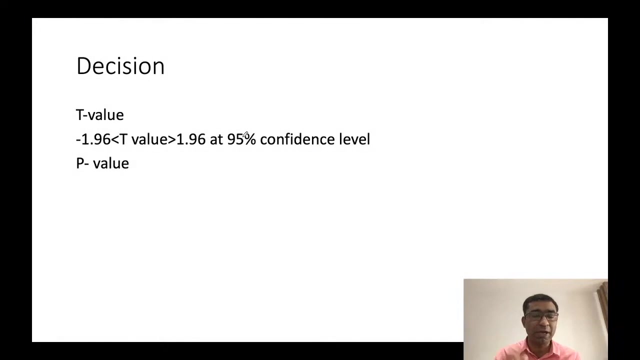 practice. okay, okay, let's, let's move to this point. but, as I mentioned in the final, in the in the start of this lecture, I told you we are going to. I am going to give you one simple tip through which you can analyze whether your hypothesis is accepted or rejected. so you have to make this decision. so the decision. 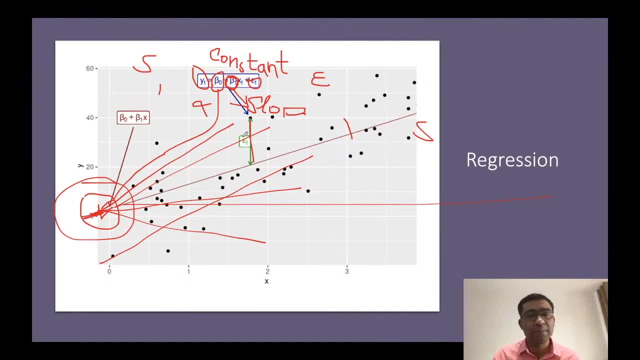 this line is inclined with the x-axis, so we can predict our values very clearly. ok, so this is how simple, ok, clear, ok, if it is clear, is there any question you want to ask? to the next step: we are going to use SPSS now to do all this in practice. ok, 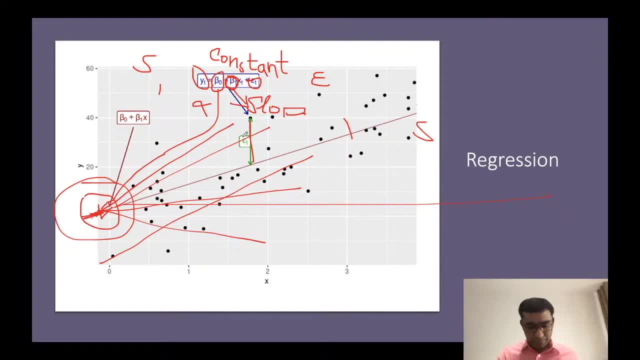 ok, ok, ok, Ok, let us, let us move to this point. but, as I mentioned in the final, in the start of this lecture, I told you we are going to. I am going to give you one simple tip through which you can analyze whether your hypothesis is accepted or rejected. so you have to make this decision. 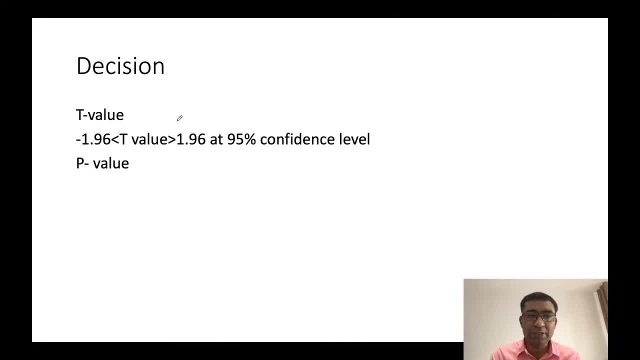 So the decision of the hypothesis is not accepted or rejected. decision of your hypothesis is very simple. okay, so you have to check the p value. only one p value. okay, so p value should be less than 0.05. okay, so please mark this word. okay, so please mark this word. 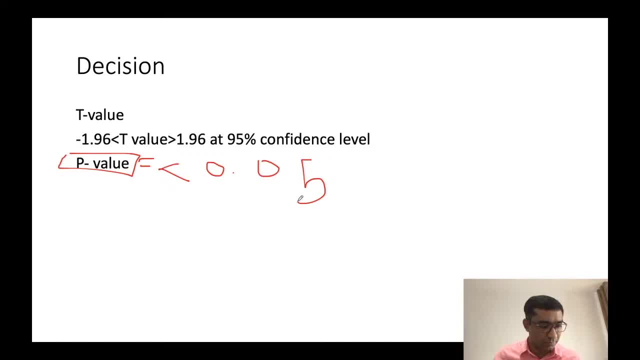 okay, so let's move on. uh, we we need to understand. the p value is one which we are going to calculate, and the p value will decide whether our hypothesis is accepted or rejected. so, mainly, our hypothesis is rejected if the value is less than 0.05. okay, clear. 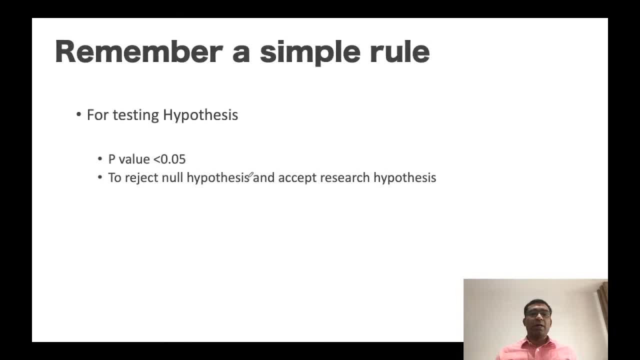 okay, let's move on. uh, let's do some practice. uh, remember this rule: p value is less than 0.05. i'm going to explain. 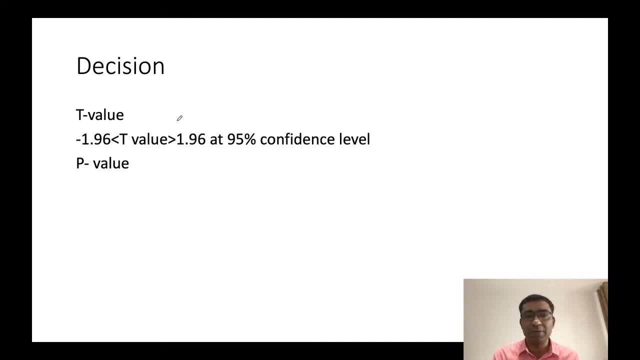 of your hypothesis is very simple. okay, so you have to check the p-value. only one p-value, okay, so p-value should be less than 0.3, 0.3, 0.3, 0.3, 0.3, 0.3. 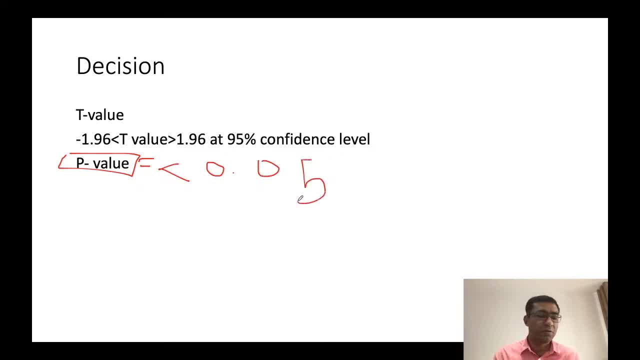 0.3- 0.5. okay, so please mark this word. okay, so please mark this word: 0.3, 0.3 O.3. So let us move on. we need to understand. the p-value is one which we are going to calculate. 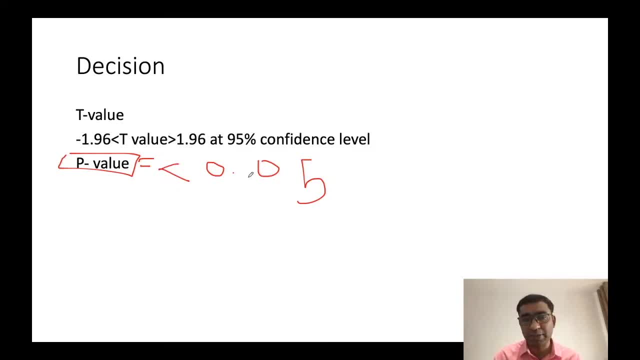 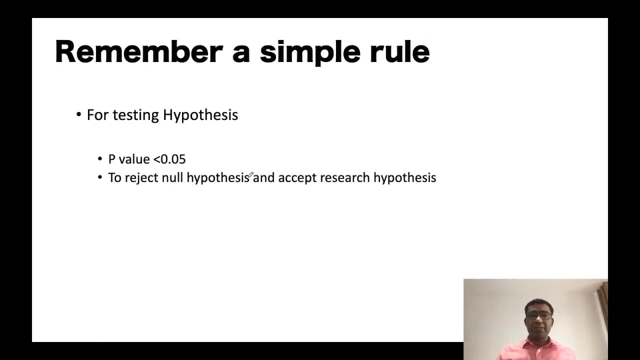 and the p-value will decide whether our hypothesis is accepted or rejected. so, mainly, our hypothesis is rejected if the value is less than 0.05, okay, clear, okay, let us move on. let us do some practice. remember this rule: p-value is less than 0.05,. I am going to explain. 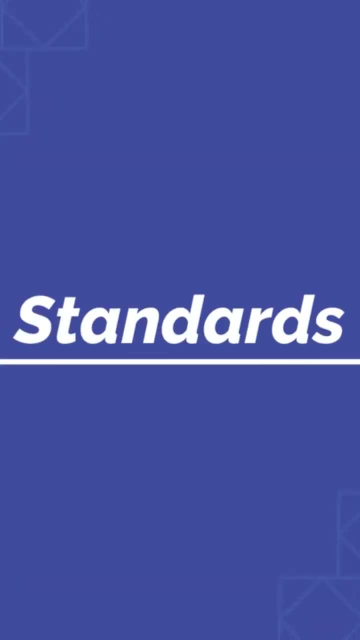 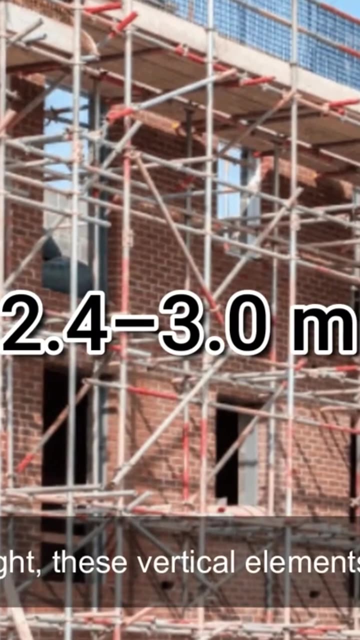 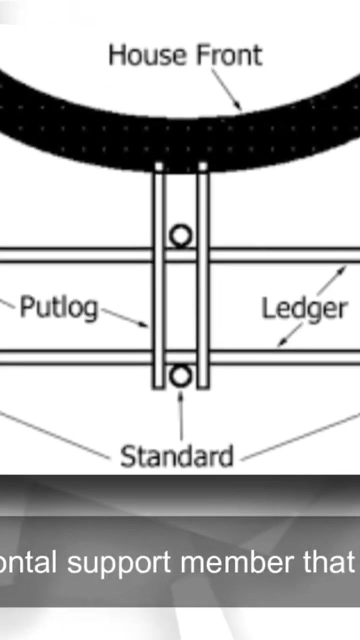 Components or parts of scaffolding Standards. Scaffolding is supported by standards with vertical members embedded in the ground. At 2.43.0 meters in height these vertical elements are spaced apart. Putt logs, Putt leg, is a horizontal support member that rests on ledgers. The standard 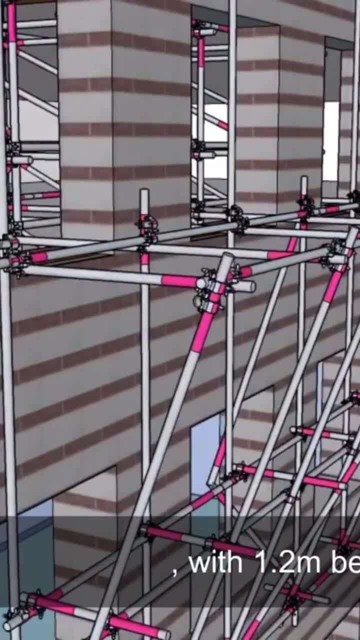 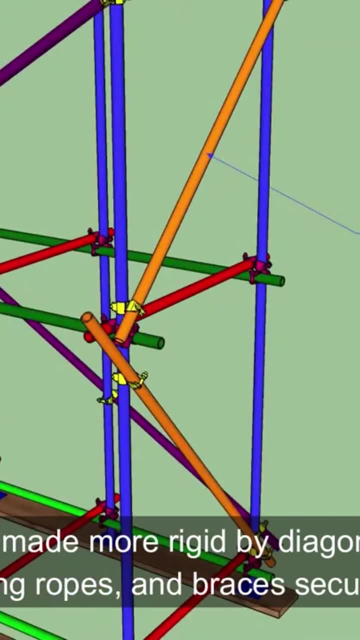 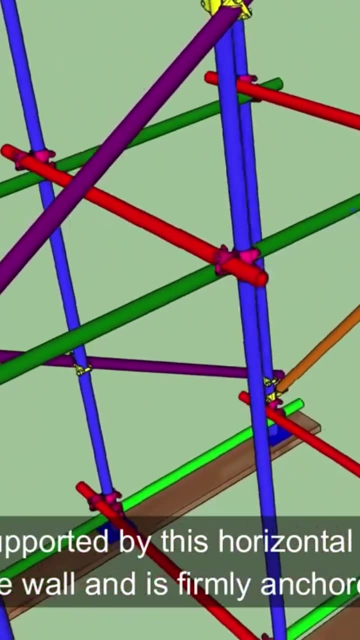 length is 90 centimeters, with 1.2 meters between each one Braces. The scaffolding is made more rigid by diagonally tying bracing pieces. Using ropes and braces secure the poles Ledger. The putt leg is supported by this horizontal element which runs parallel to the wall and is firmly 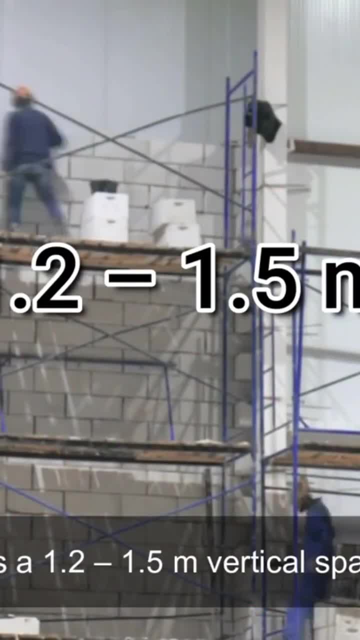 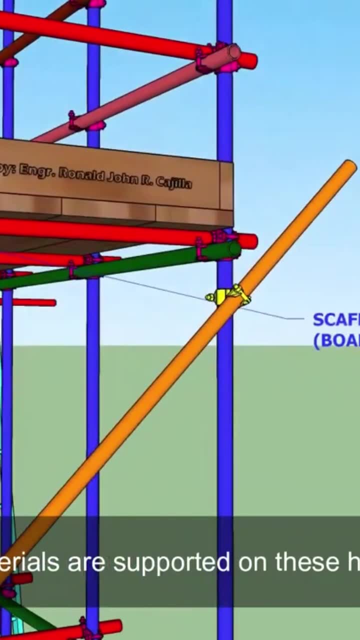 anchored in the standard. It has a 1.2- 1.5 meters vertical spacing Boarding. Site staff and construction materials are supported on these horizontal platforms by masons. The putt logs are able to deal with them Railing. This is a working